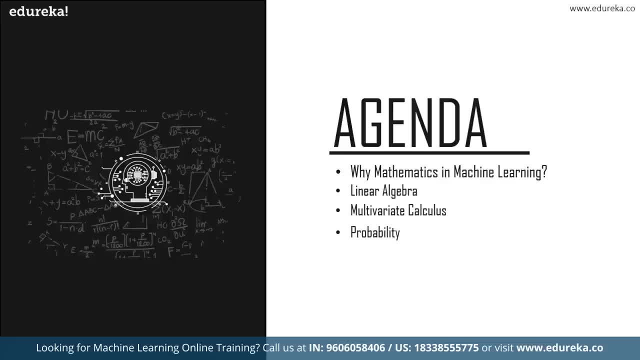 move over to probability, where we will learn its basics and discuss about the naive Bayes classifier. We shall be then ending the session with statistics basics, the types, hypothesis testing and a practical example. So I hope you are clear with the topics being covered. 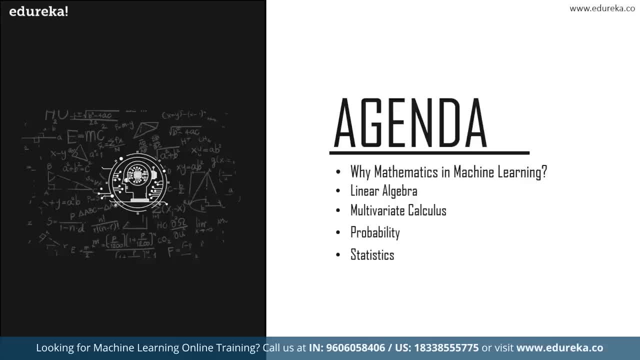 for today. Now, before we get started, subscribe to the Edureka YouTube channel and hit the bell icon to never miss an update from us on the trending technology. Also, if you are looking for an online training certification on machine learning, check out. 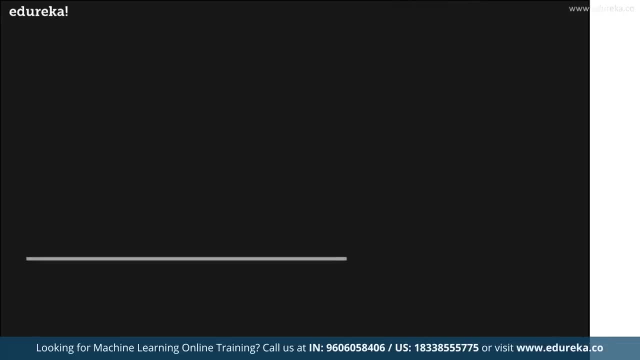 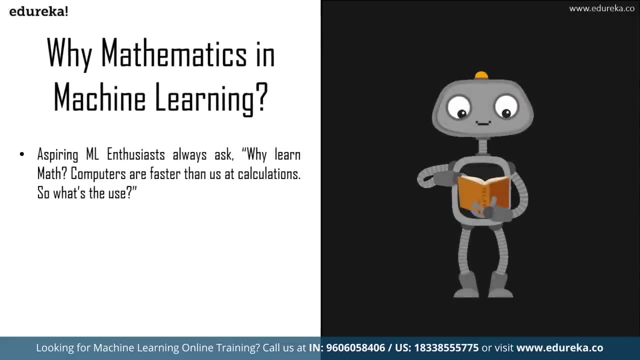 the link in the description box below. So let's jump into the first topic for today: Why mathematics in machine learning? Aspiring machine learning engineers often tend to ask me: what is the use of mathematics, machine learning when we have computers to do it all? 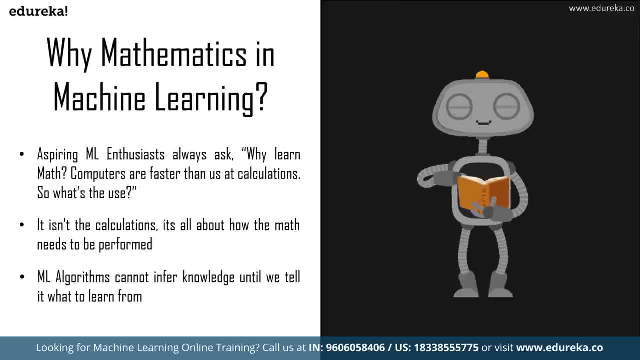 Well, that is true. Our computers have become capable enough to do the math in split seconds, where we would take minutes or even hours to perform the calculations. But in reality, it is not the ability to solve the math, Rather it is the eye of how the 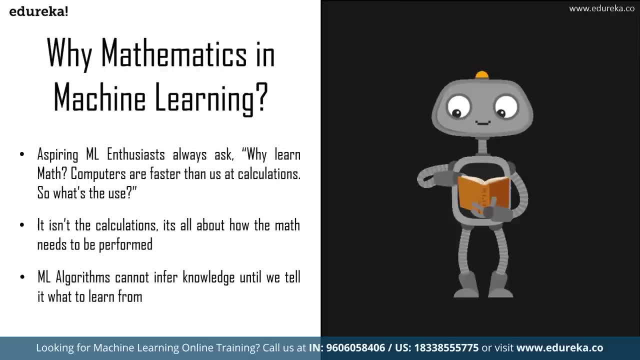 math needs to be applied. You need to analyze the data and infer information from it so that you can create a model that learns from the data. Math can help you in so many ways that it becomes mind-boggling that someone could hate this subject, Of course, doing. 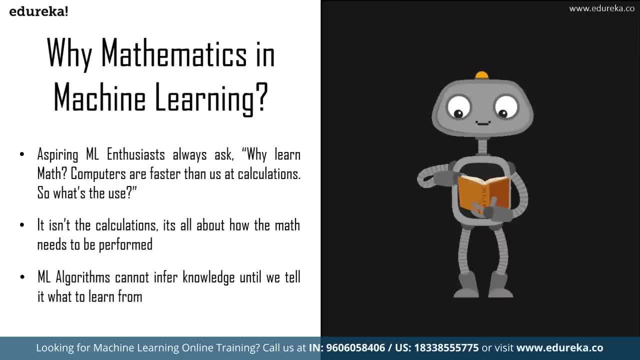 math by hand is something I hate too, But knowing how I use math is enough to explain my love for math. So allow me to extend this love to you guys too, because I won't be teaching you just the mathematics for machine learning, but the various applications you can use it for in real life. 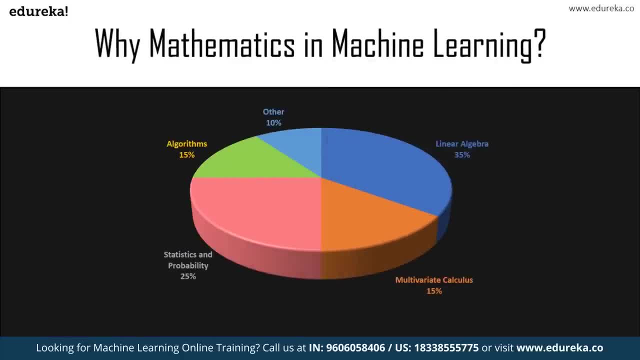 So what math do we need to learn for machine learning? Here is a pie chart which comprises of all the needed math. Linear algebra covers a major part, followed by the multivariate calculus. Statistics and probability also play a big role, and you need to know the knowledge. 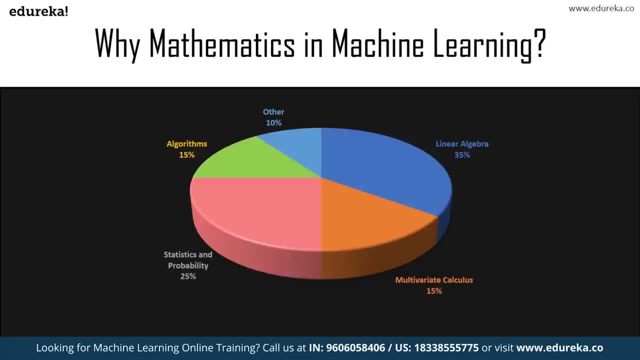 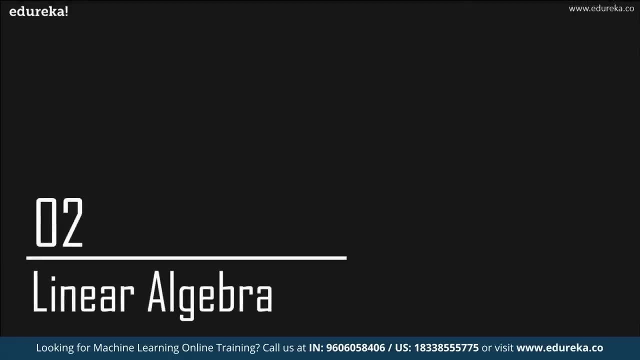 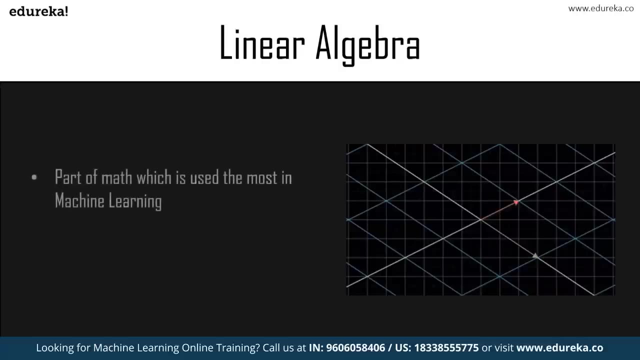 of algorithms and much more. This is the requirement for machine learning. So now that we have developed this understanding, let's do some math. We shall kick off with linear algebra. Linear algebra is used most widely when it comes to machine learning. It covers so many aspects, making it unavoidable if you want to learn mathematics for machine. 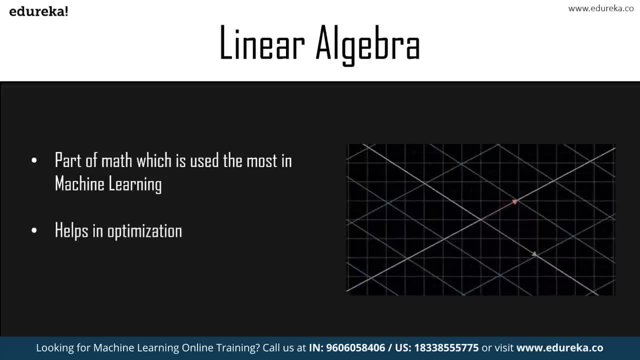 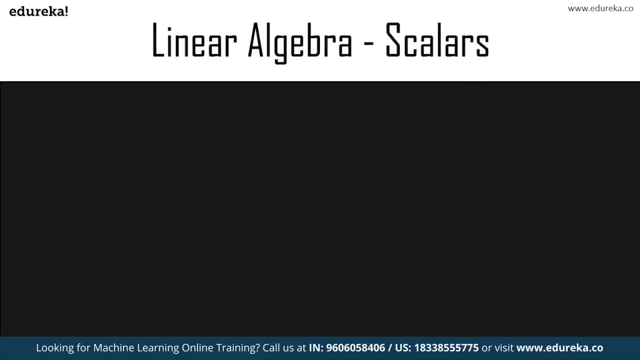 learning. Linear algebra helps you in optimizing data operations that can be performed on pixels, such as sharing a rotation and much more. You can understand why linear algebra is such an important aspect when it comes to mathematics for machine learning. So let's move over to the first topic in linear algebra: scalars. 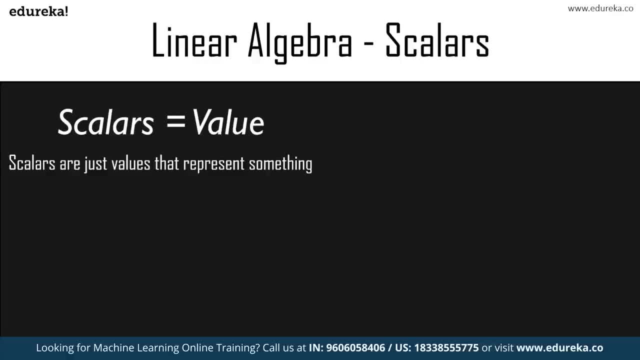 So what is a scalar? A scalar is basically a value. It represents something, right? So scalars are just values that represent something thing. Suppose we had a laptop on sale and it is priced at 50,000 rupees, right? So this 50,000 rupees is the scalar. 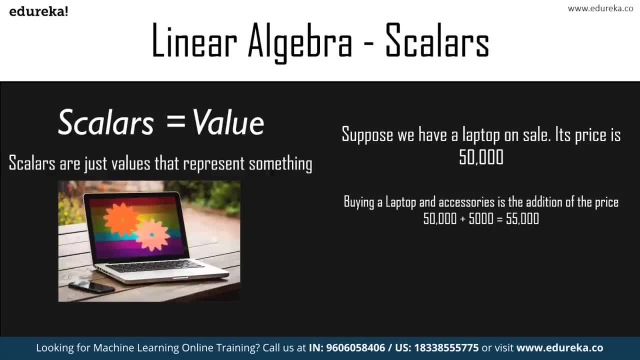 Okay, Scalar value of that laptop. What are the operations that can be performed on scalars? first, It is just basic arithmetic. So, for example, we have addition, subtraction, multiplication, division. all of those operations can be applied on scalars. 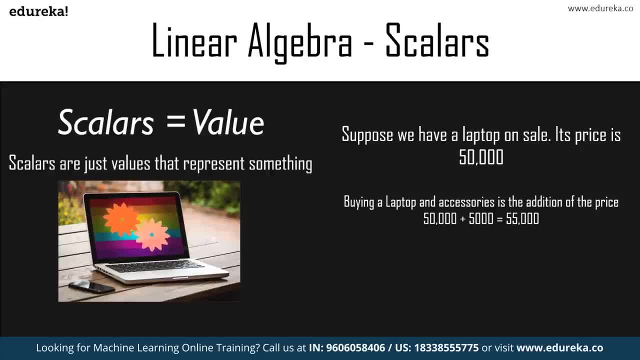 Okay, For example, over here we are buying a laptop and the accessories. What is the total price? It will be the addition of both the prices, So 50,000 for the laptop and 5,000 for the accessories, brings it up to 55,000 rupees. 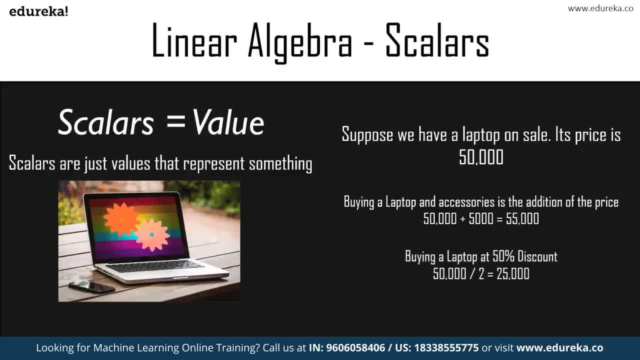 What happens if you're buying a laptop at a 50% discount? So it is half the price right? It is 50,000 divided by 2. that becomes 25,000 rupees for the laptop. So this is just a brief introduction and all that is required from scalars. 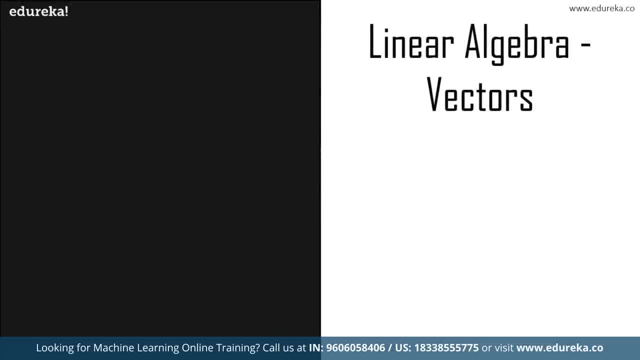 So once we are clear with this, let's move over to vectors. So vectors can get a bit complicated as they are different for different backgrounds. Let me tell you how computer science people can interpret vectors As a list of numbers that represent something. physicists consider vectors to be a scalar. 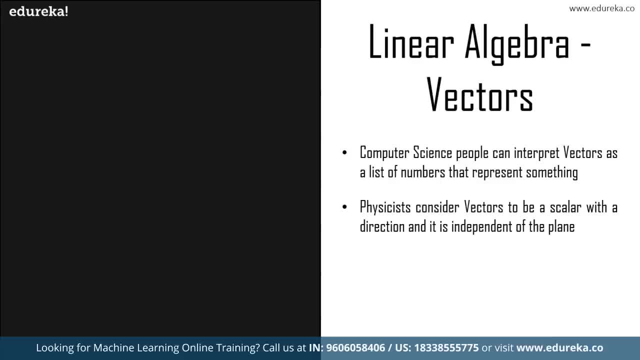 with a direction and it is independent of the plane. mathematicians take vectors to be a combination of both and try to generalize it for everybody. All of these standpoints are absolutely correct and that's what makes it so confusing for anyone learning about linear algebra, for mathematics, for machine learning, in machine learning. 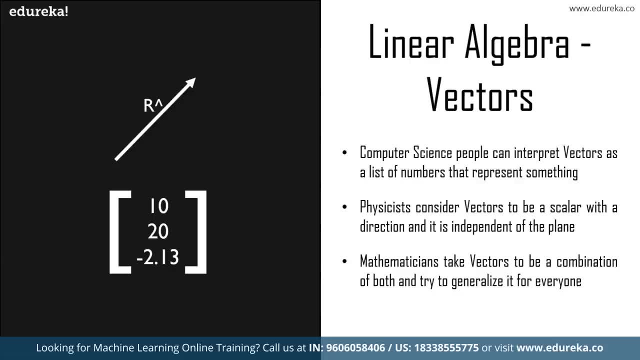 We usually consider vectors in the standpoint of a computer Scientist. where the data is in the tabular form, consisting of rows and columns right, And when our data is in the form of pixels or pictures, we consider them as vectors that are bound to the origin and transform them to matrices and perform operations that we 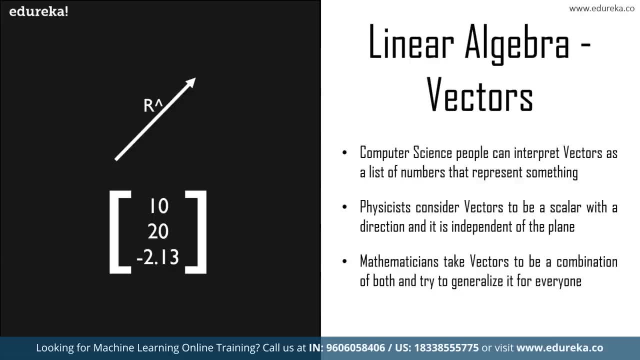 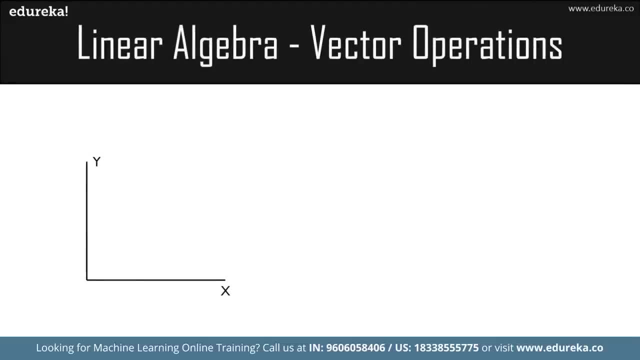 shall discuss later. So now that you have a brief idea about vectors, let's jump over to the operations that you need to know when working with vectors. operations on vectors can be applied only when you know what kind of data Data You're working with. suppose you have pixel data and you want to apply rotations, but end. 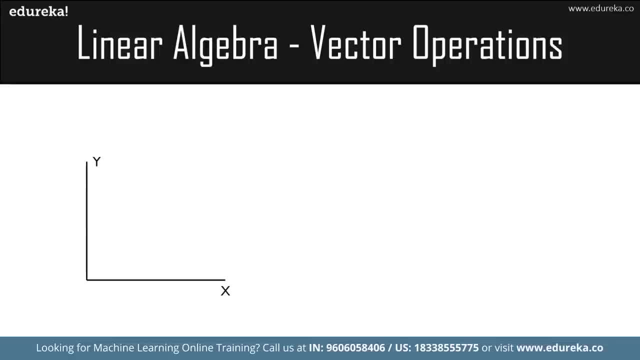 up doing something wholly different. your model will not work because it is doing all the wrong operations here. It's important that you make sure that you know what you're working with. only then you will be able to apply the required operations. So the first operation that we have here is vector addition. 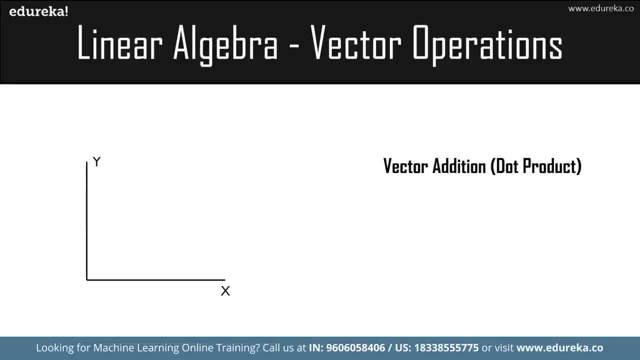 So let's understand what vector addition does us. So, for example, vector addition is also called as dot product. Vector addition is something that is completely different from operations that we've been learning now for scalars. It's not simple arithmetic, It is actually the total work that is done by both the vectors in a quantified form. 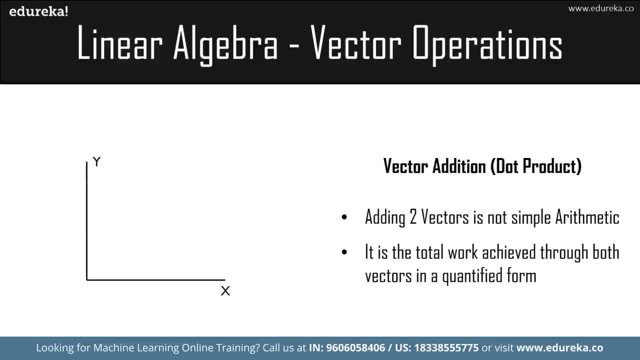 So, for example, let me say that I want to walk forward by 50 meters, and that is one vector. So me walking forward for 50 meters is one vector, and from there I go right for 25 meters. So that is the second vector. 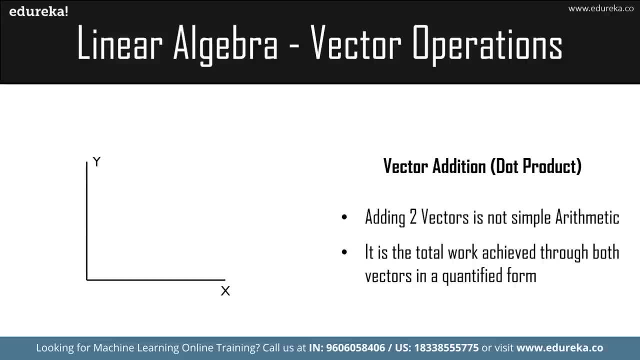 So what is the work that is completely done by both these vectors? is me moving forward and then moving right? So let me say, for example, V1 is what I walked forward, Okay, and then V2 is something that I moved right. So what is the addition of this? the addition is basically putting both the vectors point. 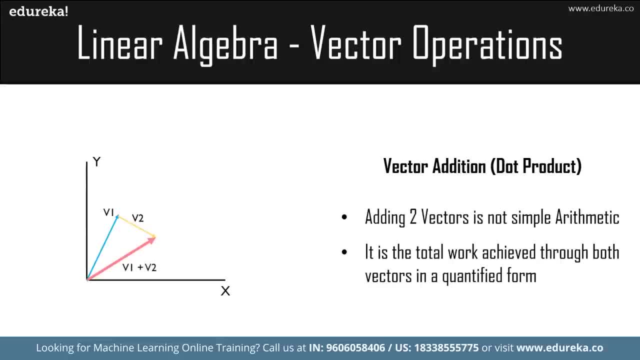 to point and then finding the displacement or the work that has been done. If you look at it over here, it is V1 plus V2.. V2's work, that is in the quantified form of V1 plus V2.. It is the displacement. 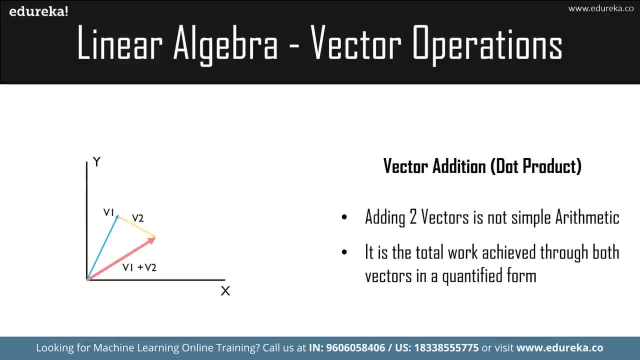 So, for example, V1 is a distance and V2 is a distance. V1 plus V2 is the displacement. So that is basically what is a dot product. I hope you've understood this. So let's move over to the next operation, that is, a scalar multiplication. 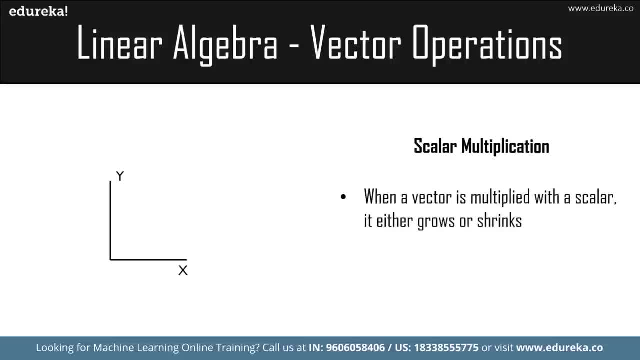 So what is scalar multiplication? So whenever a vector is multiplied with a scalar value, It either grows or shrinks. what this means is that you have a particular value, a scalar value, which is either positive or it is negative, and it may be greater than one or lesser than. 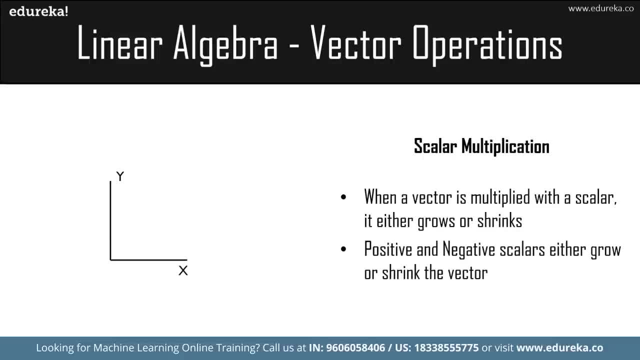 one. whichever is lesser than one and it is negative, It will always make it shrink, or else it will do the opposite, It will make it grow. So let me just show you an example over here. So let's say I have a vector called V1.. 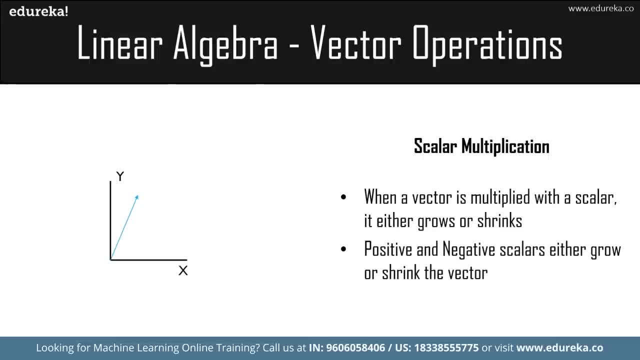 Now, if I'm trying to multiply This with a positive scalar value, say K, positive scalar value into V1 will make the vector grow, Whereas if I am trying to multiply this particular vector with a negative scalar value, say minus K, it will be shrinking down, down. 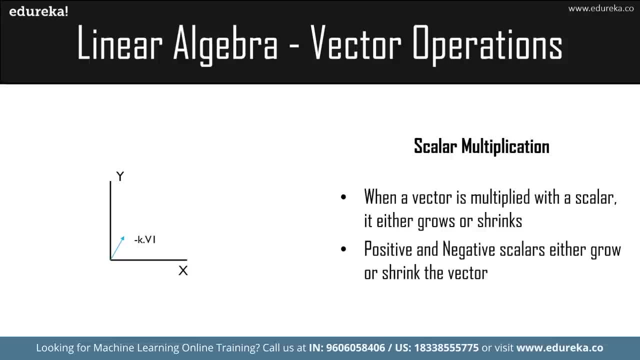 So it is minus K into V1 gives me a shrink vector. So, as you can see, this was my normal vector and if I multiplied it with a constant K, which was positive, it grew, And if it was negative, it shrink down. so that is basically what is a scalar multiplication. 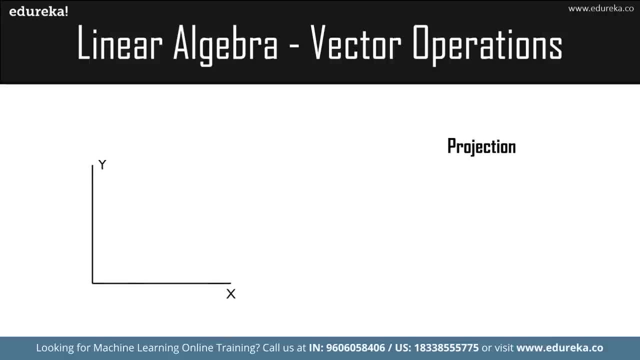 So the next vector operation is projection. So what does projection help us with? so, for example, let's say I have two vectors, okay, V1 and V2. now I do not know much about V1 and I just know more about V2. so, if I can, 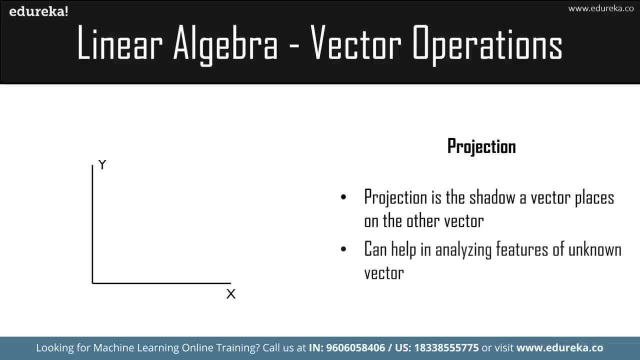 try to find a way in which I can project the vector V1 onto V2.. Well, to v2 I'll be able to obtain information about v1, so let me just show you. so, for example, I have a vector v1 and I had another vector, v2. so I know all about v2, but I do not know about v1 vector. 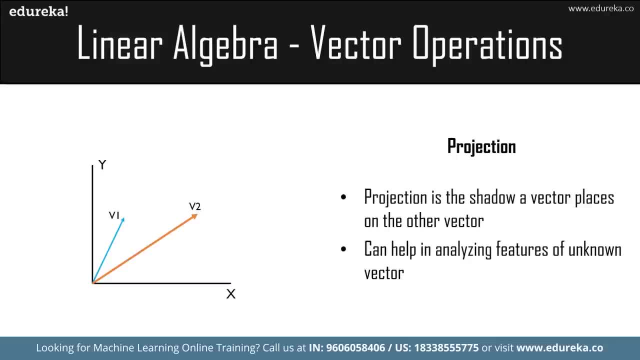 so what happens over here is, if I'm able to project the projection of vector v1 onto v2, I will be able to analyze and know the unknown features that vector v1 has. okay, actually, if you go with this into deep learning, right, you can be able to find unknown features of the vector. 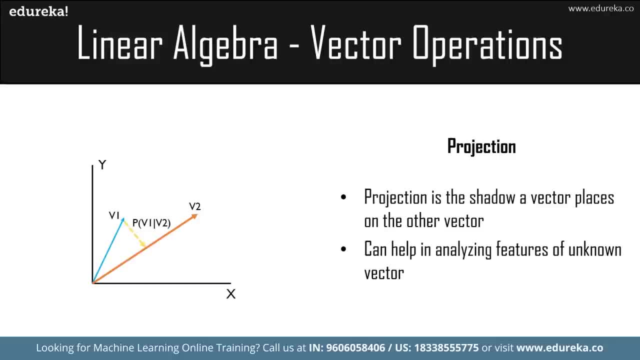 which can help you modify your one image into so many images that you can basically simplify and modify that image into something that it is not okay. that comes under deep learning, but we are not going to cover that, but this is a very important concept that you need to understand. 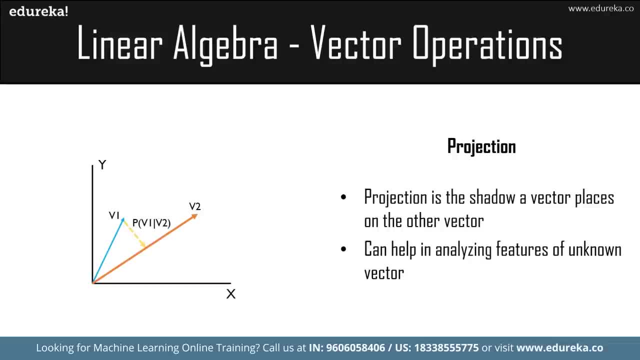 it is basically like it's said over here: projection is the shadow of a vector that it places on the other vector. so whatever information you have, you can modify it into something that you can project into it. so if I have the information that v1 vector has, I'll be able to somehow 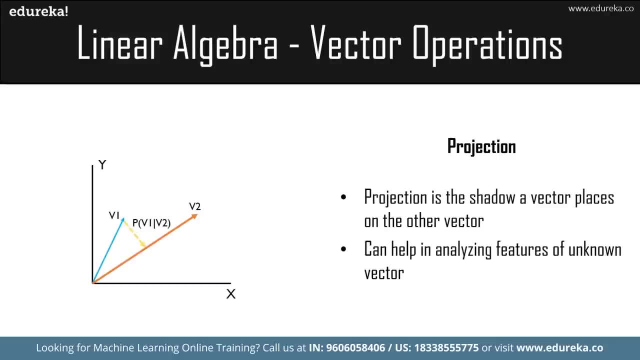 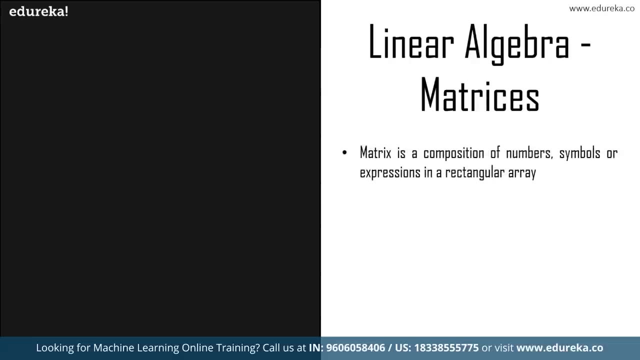 extract it from the vector v2, because the projection falls onto v2. that basically brings us to the end of all the vector operations that you need to remember for machine learning. let's move over to matrices. so what is a matrix? a matrix is the composition or it is the mixture of numbers. 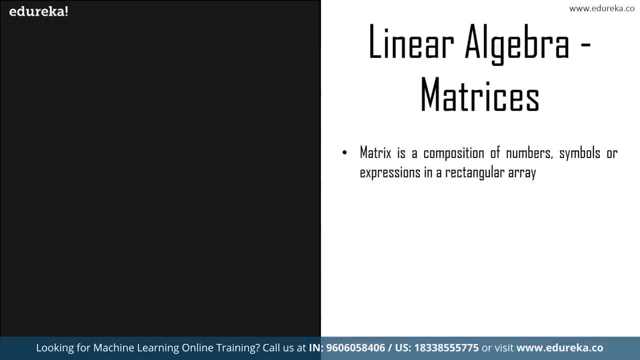 symbols, expressions which are in a rectangular form, and the matrix is the composition, or it is the mixture of numbers, symbols, expressions which are in a rectangular form and the matrix is the composition array. it can be rectangular, it can be square, it depends on the order. so what do we use? matrices. 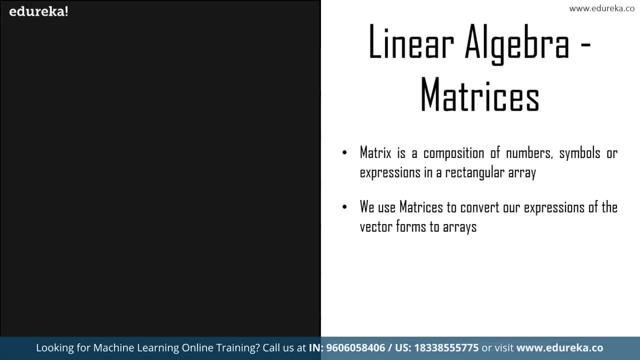 for we use matrices to convert our equations into the form of arrays. for example, if you've got an equation, you cannot simply put that into your computer saying that, okay, solve this and give it to me. you need to convert it into a list or an array so that you will be able to perform your 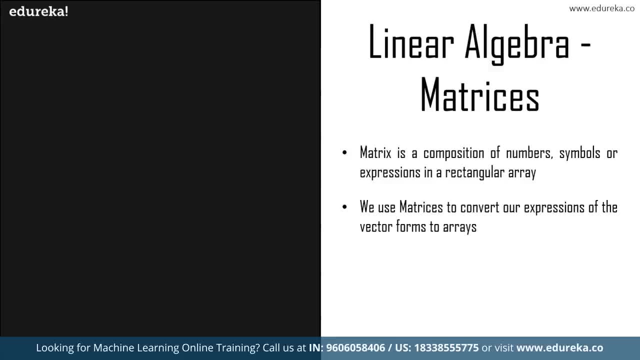 operations on it, right? that is the reason matrices are so much important to us and that is the reason it is much more easier for us, so that we can convert our equations into lists and arrays and then perform our operations on them. so suppose, for example, you have two equations over here, so how do you convert these two equations into matrices? 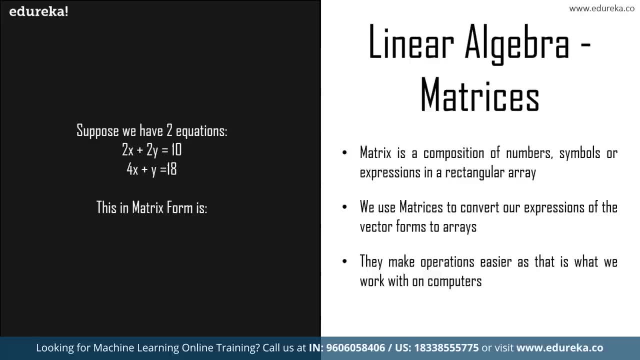 so what does a equation tell you? if you have, 2x plus 2y is equal to 10. what this basically is trying to convey the information to you is that you have to convert these two equations into matrices. so what does a equation tell you? if you have, 2x plus 2y is equal to 10. what this basically is trying to convey the information to you is that you have to. 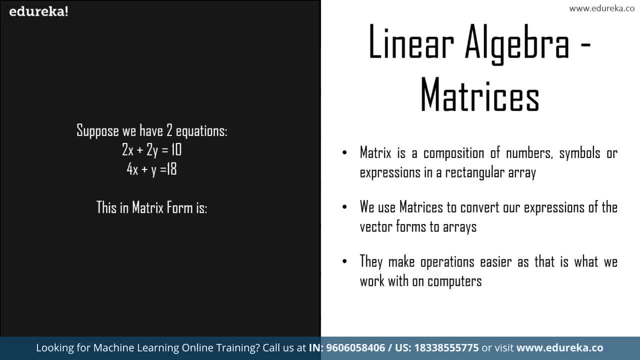 constants X and Y. in these constants, if you keep giving different numbers, you will be able to find a different value for it. let's say, for example, the scalar value is 10 and you have 2x plus 2y, which is basically a vector. I need to find the points of X and Y. find the points of X and Y. 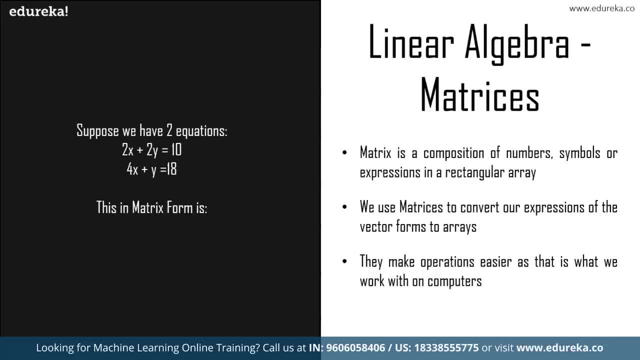 meaning that I'm trying to find the direction of the vector and then, if I'm able to substitute values and then find out how 2x plus 2y is equal to 10, I am finding all the information I need from that vector so that I can basically find out what all the other information I need from it. that is how. 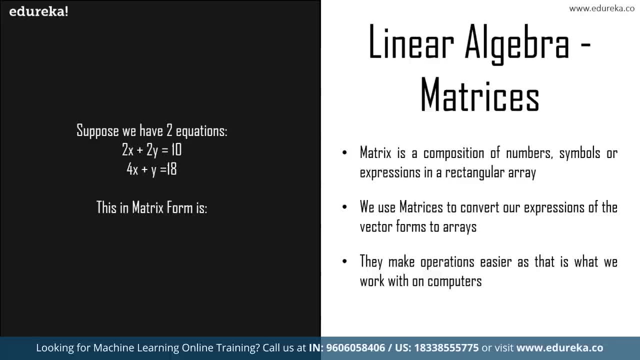 functions are very important. you need to understand what a function is trying to convey to you. let's say, for example, you have the equation of a straight line. so what does the straight line be? it is: Y is equal to MX plus C. what does this mean? it means that the Y coordinate 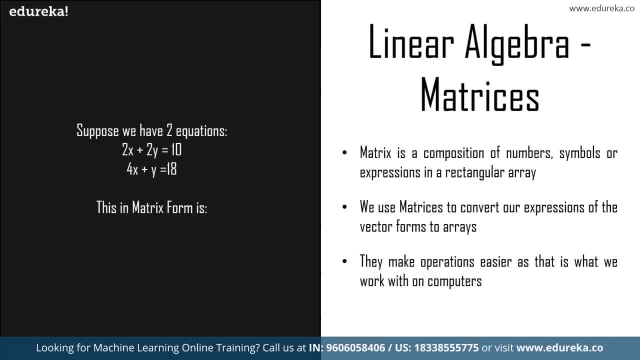 is equal to some value, M into X plus a constant. so I'm able to plot this: I'll be getting the Y coordinate, the X coordinate and I'll be able to get a straight line. so whatever numbers I put into these, I will always be getting a straight line. so that is the reason it is called the equation of a. 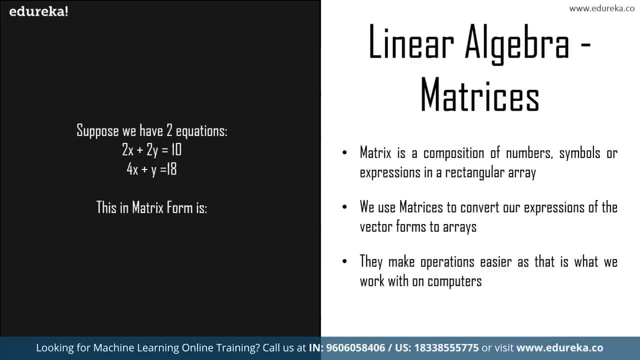 straight line. it is always going to be constant, so you have to understand what a function is trying to convey to you. once we are done with that, let me just tell you how you convert equations into matrices. it's really simple. take out all the numbers so you have 2x plus 2y, equal to 10, right? so 2x and 2y has two numbers, two. 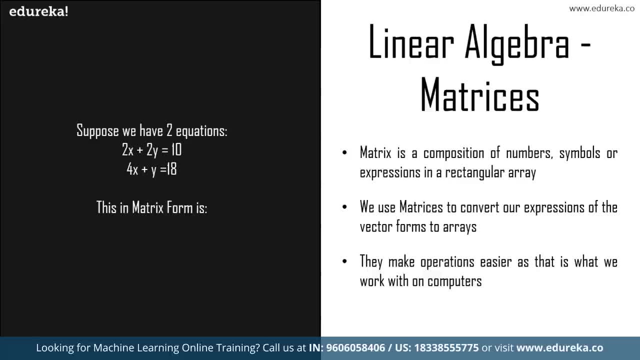 so those two become one row four and one in the second equation become one row X and Y becomes one column, and 10 and 18.. so let me just show it to you. so, as you can see, we have a matrix: 2, 2, 4, 1. 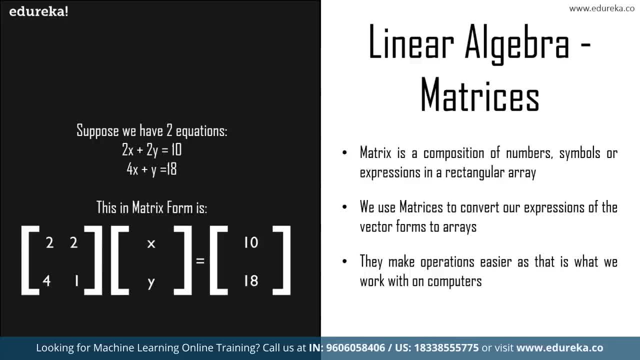 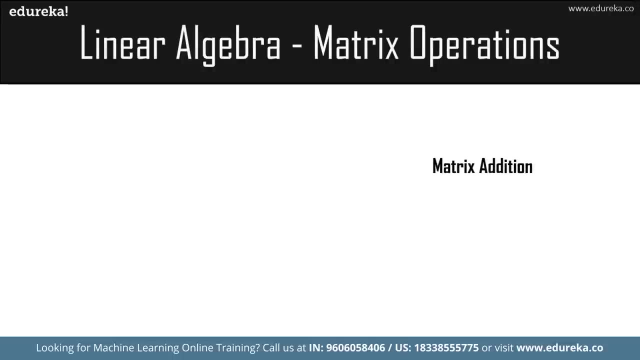 then we have X, and Y is equal to 10 and 18.. if you multiply it accordingly, you will be getting back the same equation that we had earlier. this is how matrices are used in linear algebra. so once you know how the equations are converted into matrices, let's move over to the matrix operations. so what? 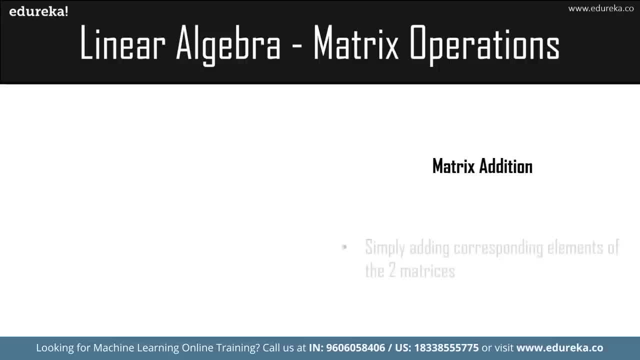 is the first operation, simple addition. what does addition help you with? it is just basically adding all the directions of two vectors. why is it two vectors? because I am converting vectors into matrices. right, simply just going to add the corresponding elements of both the matrices. simply add the corresponding. 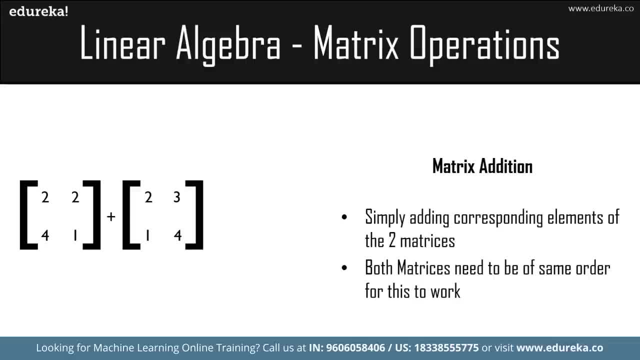 elements of both the matrices and you have to remember that if you are adding two matrices, it has to be of the same order. what do I mean by order? it is basically the number of rows into the number of columns. so, for example, if I have the first matrix, that is, 2, 2, 4 and 1, I have two rows and I 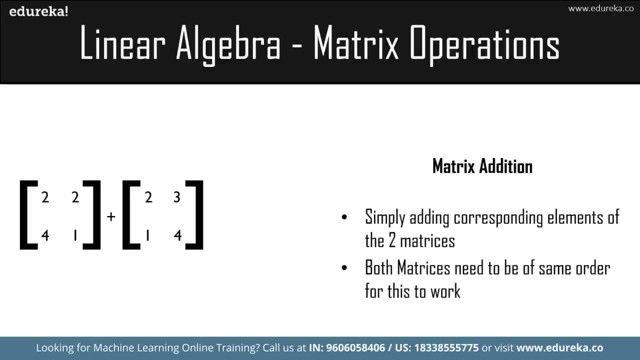 have two columns, so that becomes a 2 cross 2 matrix. that is the order of the matrix. the next one also 2, 3, 1, 4. it has two rows and two columns. that makes it an order of 2 cross 2. so if I had three rows and I had two, 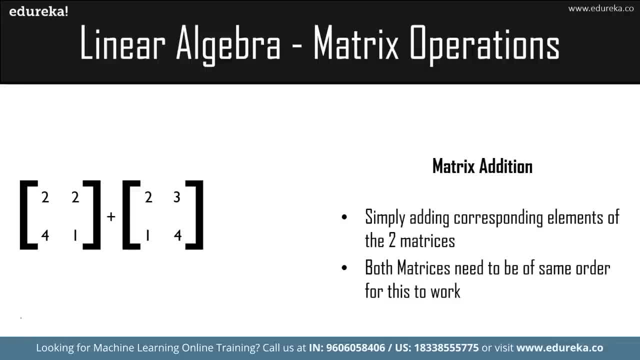 columns. it would be 3 into 2, so I hope you've understood what a order is. let's say I had these two matrices and I want to add them, so what I do it is 2 plus 2. so let's say I have two over here. 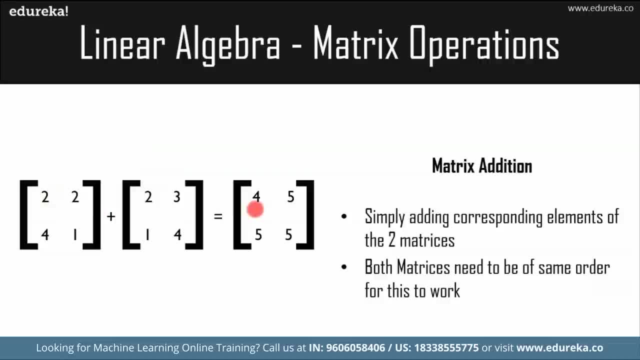 and I have two over here. so what is 2 plus 2, it becomes 4. what is 2 plus 3, it becomes 5. what is 4 plus 1, it becomes 5. what is 1 plus 4, it becomes 5. so it is adding the corresponding elements of. 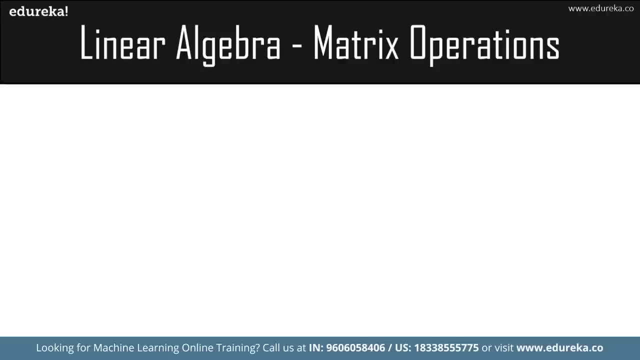 the matrix. so I hope you've understood that. so let's move over to the next operation: matrix subtraction. it's the same thing as how you did it for addition: you just subtract the corresponding elements. if you had 2 minus 2, it becomes 0. 2 minus 3 becomes minus 1. 4 minus 1 becomes 3. 1 minus 4 becomes minus 3. simple, you. 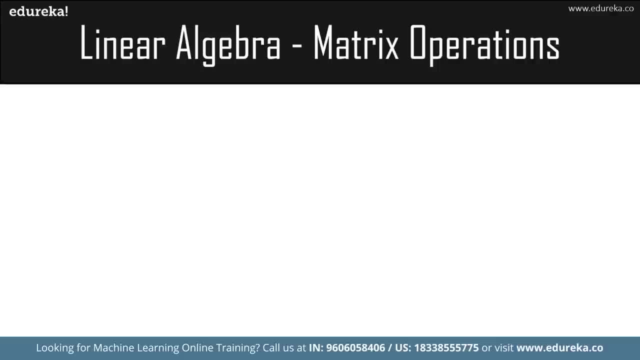 can understand this very easily. moving ahead from matrix subtraction is matrix multiplication. what do you do with matrix multiplication? you are basically multiplying the rows with the columns, the matrix of row 1 with the columns of matrix 2.. what happens? you have to remember that the number 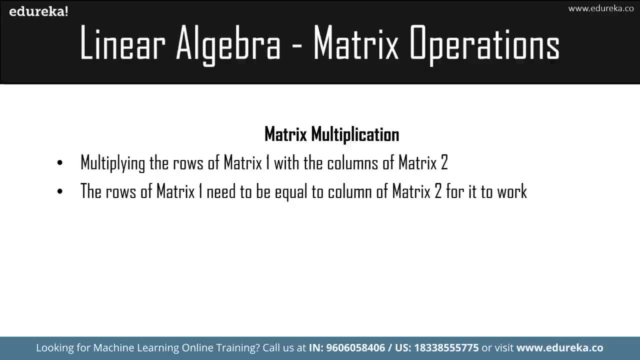 of rows in matrix 1 has to be equal to the number of columns in matrix 2. only then will you be able to perform the matrix multiplication. so, for example, if I had a 2 cross 2 matrix, it would be a 1: 1 into b 1 1 a 1. 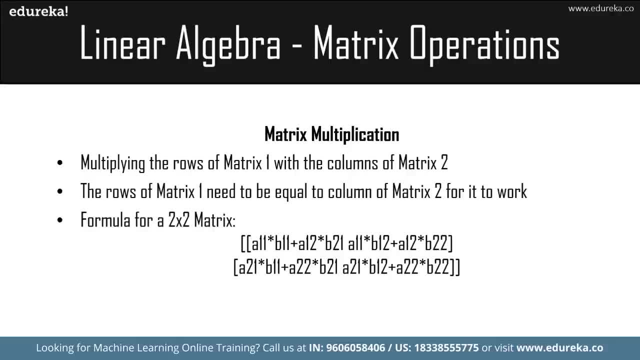 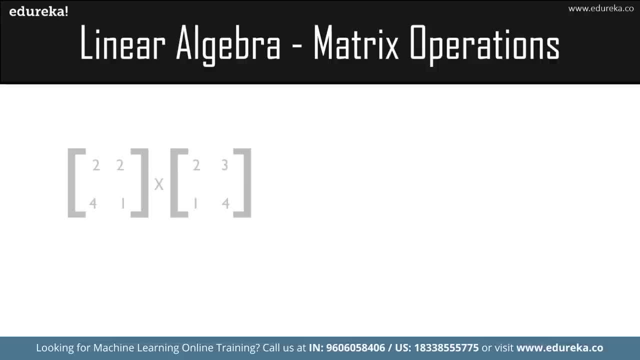 2 into b 2, 1. a 1 1 into b 1- 2, plus the a 1: 2 into b 2, 2 accordingly. so let me show you an example for matrix multiplication so that you can understand how it works. suppose I have a 2 cross 2 matrix. 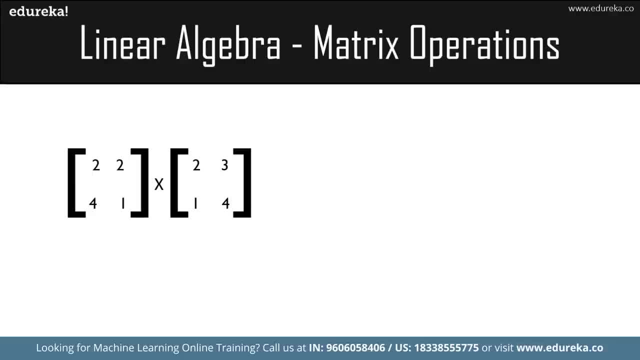 that I've already been using for matrix addition and subtraction. now How am I going to perform the matrix? multiplication is basically, I'm going to, you know, multiply the first row into both the columns of the matrix 2, so I have 2 into 2 plus 2 into 1, and I have 2 into 3. 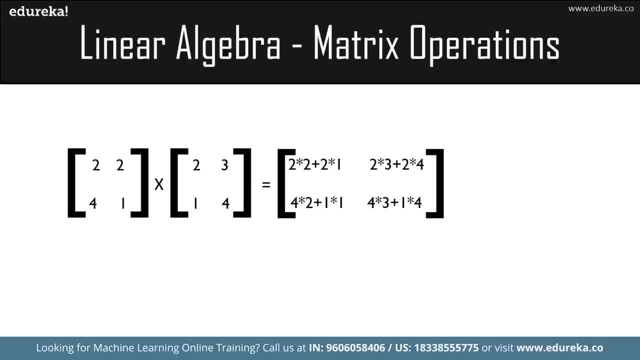 plus 2 into 4. the same thing goes for the second row also. So what do I get? I get 4 plus 2, 6 plus 8, 8 plus 1 and 2, L plus 4. that accordingly gives me 6, 14, 9 and 16.. 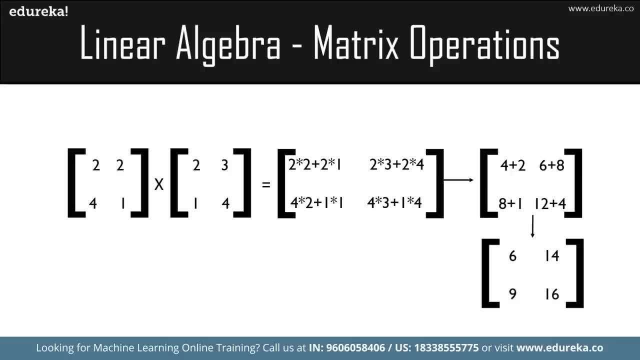 So this is the matrix multiplication. It's really simple to understand. So if you have any doubts, and leave them in the comment section, we'll get back to you as soon as possible. So once we are done with matrix multiplication, let's move over to the transpose. 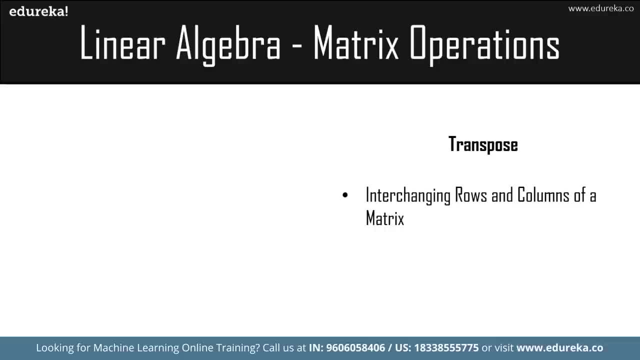 So the transpose is a really simple operation. All you do is you convert the rows into columns, That's it. But why is it so important? transpose is really important when you want to change the dimensionality of your data. suppose All your data is in a row. 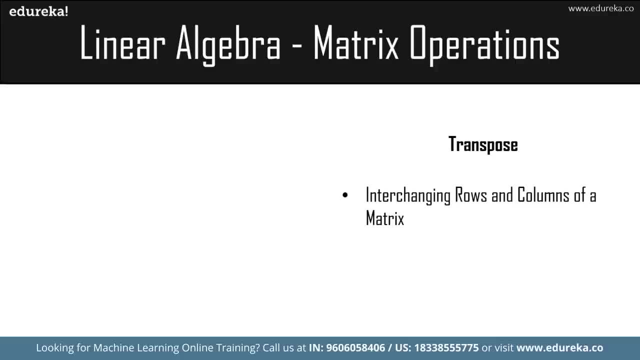 You can reiterate through that, or all your data is in a column. You can do it accordingly. So it is really important when you work with transpose, because it helps you to change the dimensionality, It helps you flip the dimension. So, for example, if you're working with pixels, right pictures, if you change the rows or the columns of 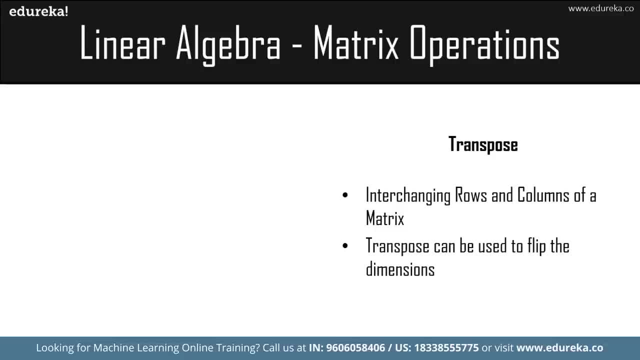 your pictures data. you are basically changing the picture and then you can, you know, analyze it more, get more information, Information from it. So transpose plays a very important role. you need to understand that. So, for example, I have two to four and one. what happens is the first column becomes the first row. 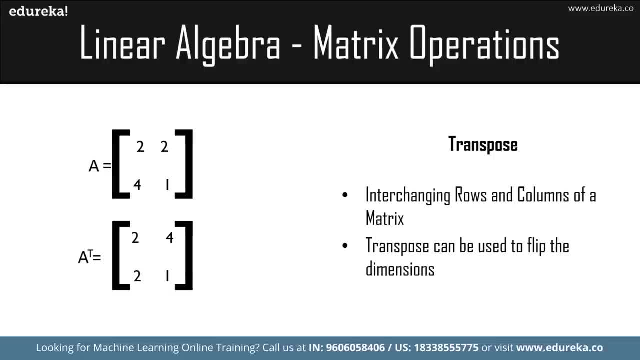 and the second row becomes the second column. So, as you can see, here it is a two to four and one, and that is all transposes. So let's move over to the next operation. We have determinant of a matrix by now. All we have been doing is having matrices being 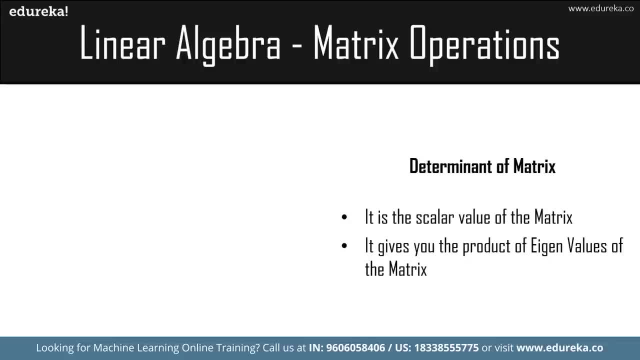 Added, subtracted. So what is all of this is? it is basically all the vectors being added, subtracted, multiplied, you know, then flipped with their dimensions. You will understand this when you do all of this practically, because all of this is something that we do not do it in our daily lives. 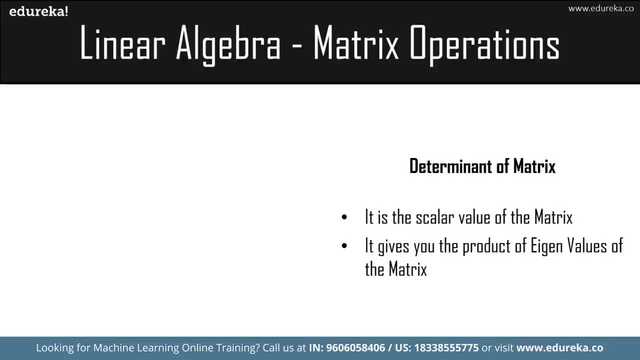 But when you're learning with machine learning, when you're performing machine learning, all of these operations come into picture. So all that you've learned by now is basically adding values of vectors, Subtracting vectors, multiplying two vectors, then transpose, that is the flipping of vectors. 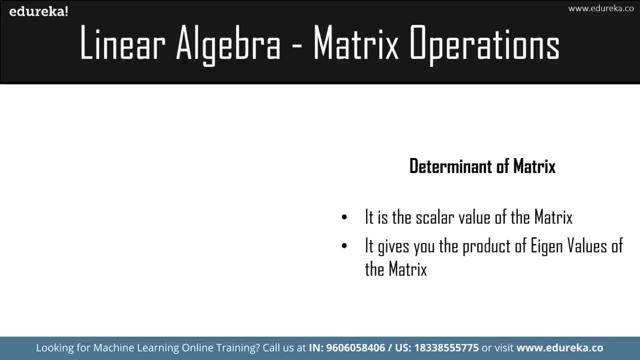 And now you're going to learn about determinant. What is a determinant? All the matrices that we had till now. They are basically directions. They are basically directions and values of all the vectors. Now, all these vectors are definitely going to have a scalar value in them, so that you can understand. 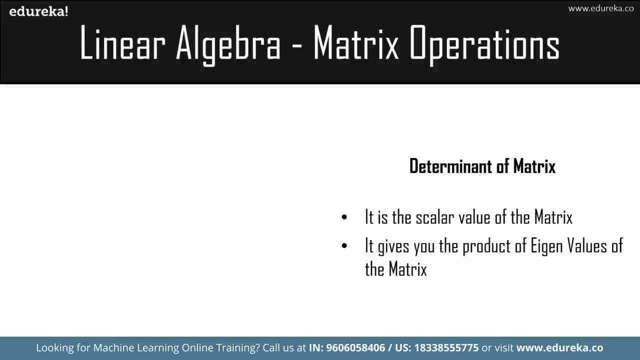 the weight, you can understand the depth of that particular Matrix. What is the determinant helping you with? with the determinant helps you with understanding the weight or the- you know- sensitivity that it can provide on the data set. that is the reason determinant is really important. 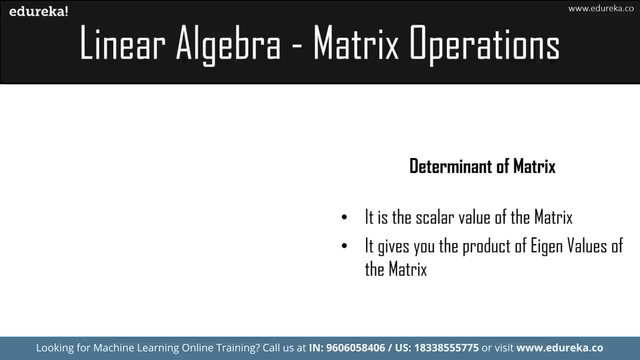 It is the scalar value of the matrix and it can help you give the eigenvalues of the matrix. What do I mean by eigenvalues? I'll teach that to you in the next part, because we are going to understand in depth water eigenvalues and eigenvectors. 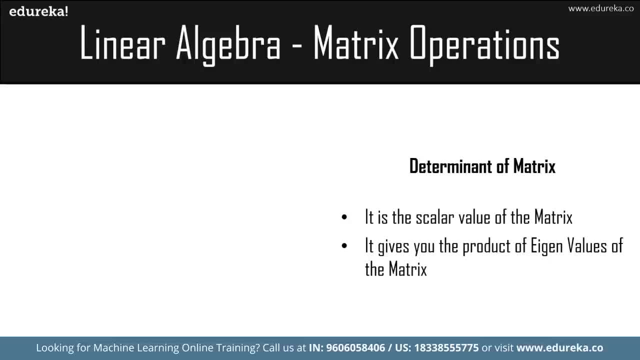 That is the reason determinants Are so important. So let's say, for example, I had this particular Matrix, ABCDEFGHI. It would be a into EFHI and then it would be minus B into DFGI, plus C into DEG H. 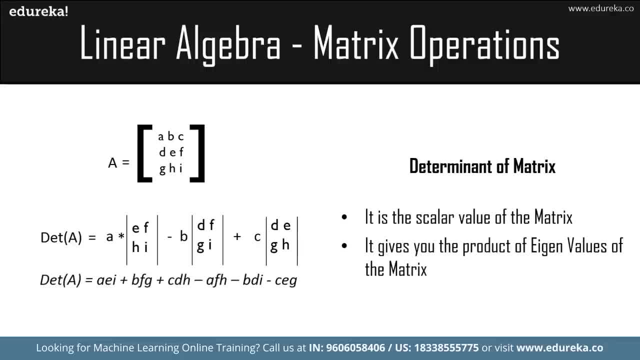 So what happens now is I'm going to get this particular equation, So it's AEI plus BFG plus CDH, minus AFH, minus BDI minus CEG. This is basically What is going to give me the scalar value of the matrix. 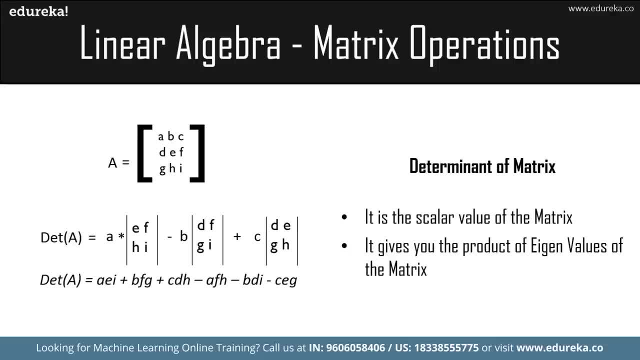 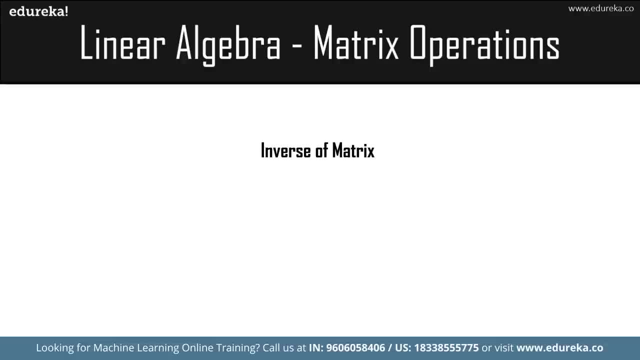 So I hope you've understood the importance and how determinants are important in machine learning. So next we will learn about the inverse of a matrix. So how do I explain inverse to you? It's a very simple example, If you understand that. suppose I am walking on a road and I walked straight for 50 meters. 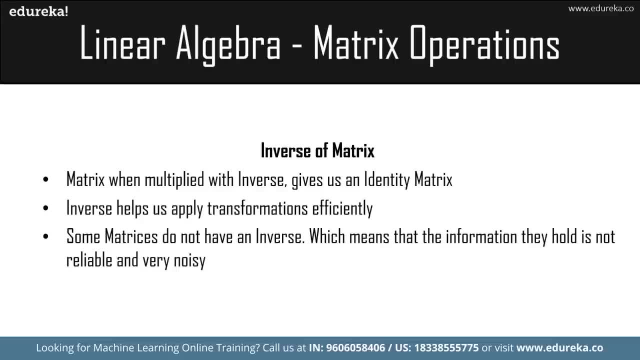 but then I remember that I had to get back something from the place I started, So I walked back 50 meters. What is the distance that I traveled? the distance that I travel was hundred meters. Why? because I went 15 meters forward and 50 meters backward. 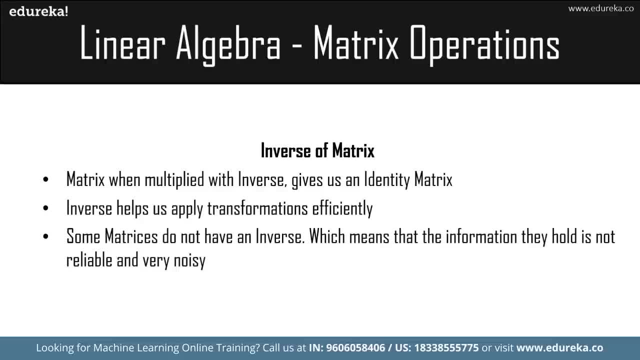 But what is the work that I have done? It is zero. Why is that? it is because I am at the same place that I started from. that is not the work done. If I move from one place to another place, that is the work done. 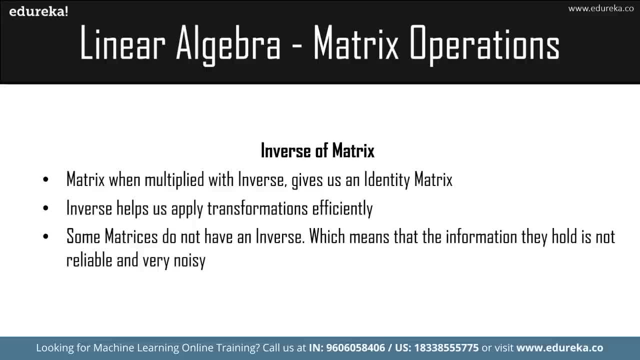 That is some displacement that my body has achieved. But I have not achieved that over here. Why? it's because I have gone straight and come back straight for 50 meters, making my work done zero. So just the same way, inverse of a matrix works. 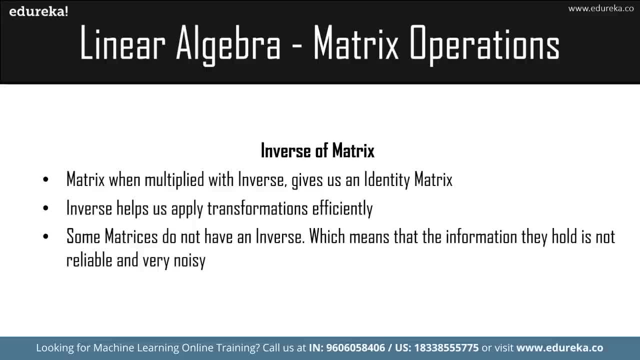 Suppose you have a vector that moves in the forward direction, You will have the inverse of that particular vector that comes in the negative direction and it makes all the work done zero. Sometimes there is no inverse of a matrix that exists. That's because the vector does not have all the information that is required to obtain its inverse. 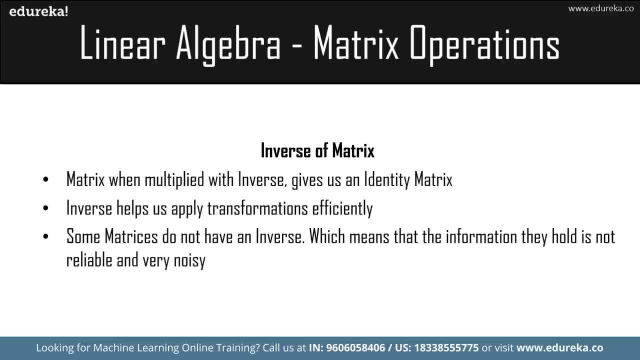 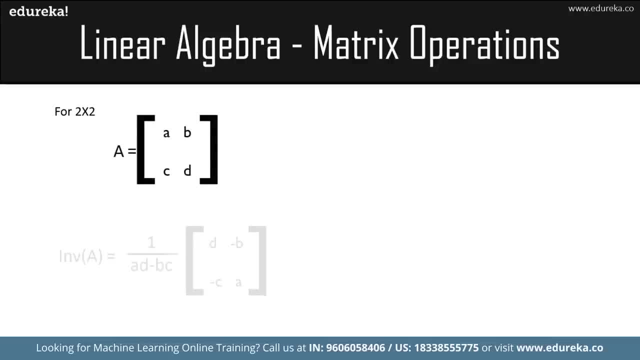 So I hope you have understood what is a inverse. Let's see How do you find an inverse of it. Okay, for a 2x2 matrix. And this is how you're going to find it. It is finding the determinant into the transpose, or, you know, finding the inverse of the matrix. 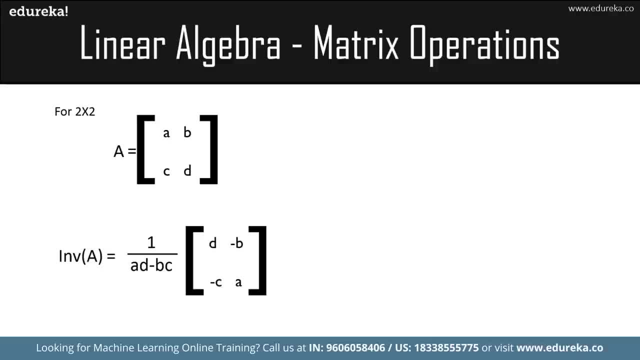 So it is a and D that is going to be, you know, switched over, and minus B and minus C. This gives you the inverse of the matrix. So, for orders 3 and above, what do you do? You find the determinant of a and then you accordingly find all the different determinants inside of it. 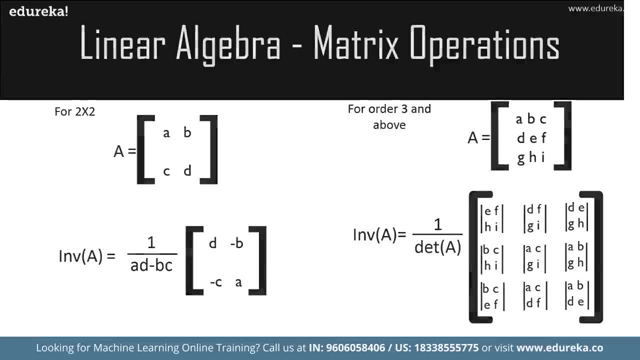 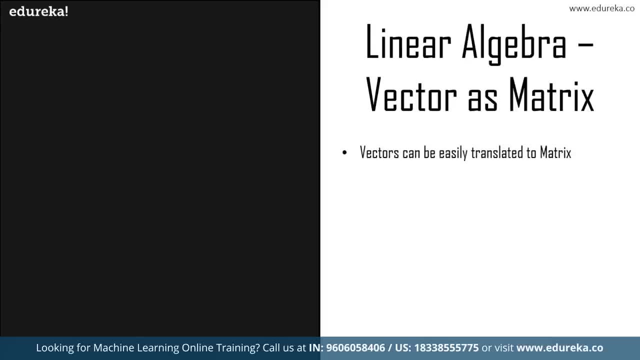 So that is basically how you find the inverse of a matrix. Let's move over to how a vector can be used as a matrix. Okay, so by now that I've been telling that vectors can be easily translated into matrices, and I've already showed it to you. and why is it so important? 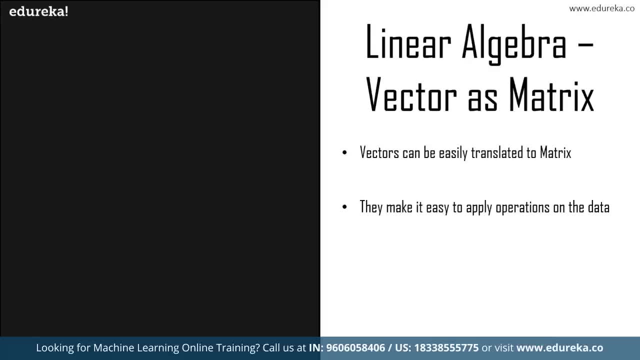 It's because they help you apply operations on the data very easily. and then you have certain well-known operations such as scaling, rotation sharing and much more. all of this come under computer graphics. Okay, making these operations on your image or your vectors becomes really easy when you're working. 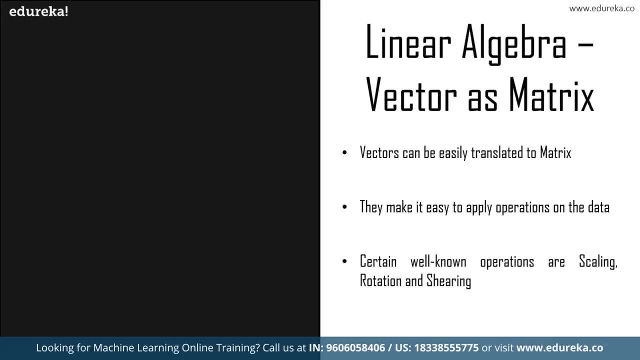 with matrices. So that's the reason matrices are so important. So, for example, right now I've shown you that if there was an equation V1 as 3x plus 4, it would be 3 and 4, and then you had X and Y. then you would have X plus 2 Y, which would become 1. 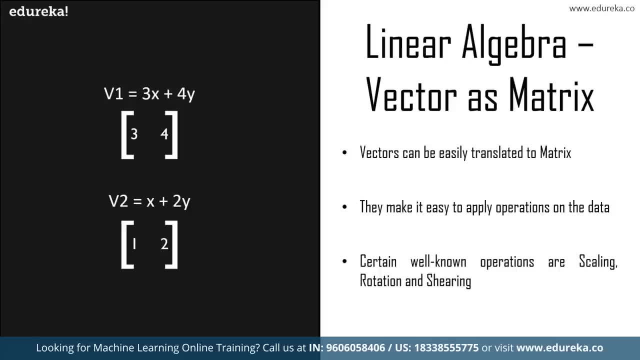 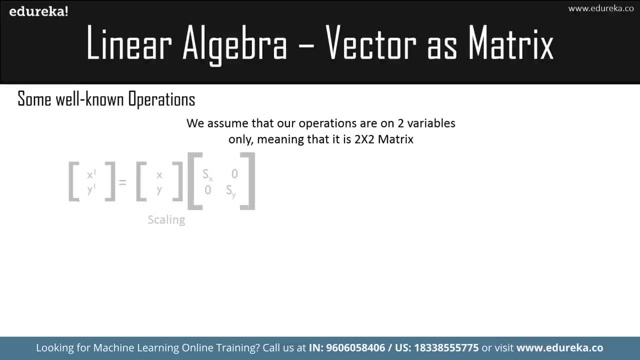 and 2.. And then X and Y. that is how vector as a matrix works. What are some of the well-known operations? right, I'm assuming that there is going to be a 2 cross 2 matrix. whenever you're scaling, It is basically increasing the size. 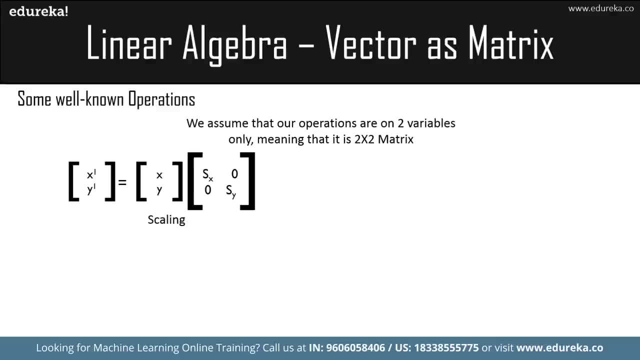 So how do you increase the size? It is SX and SY which are the scaling factors which you perform on your X and Y coordinates, and you have sharing, which is basically moving or reshaping your particular object that you're working with, so it can be M, which is the sharing. 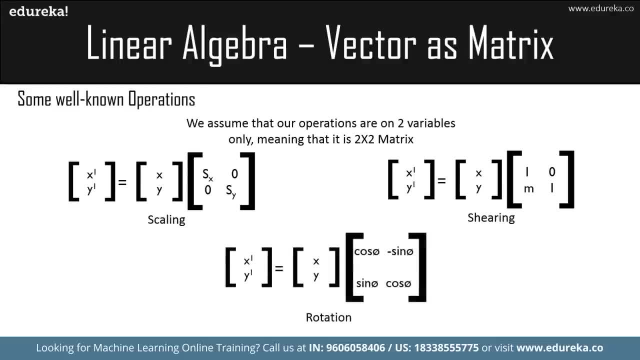 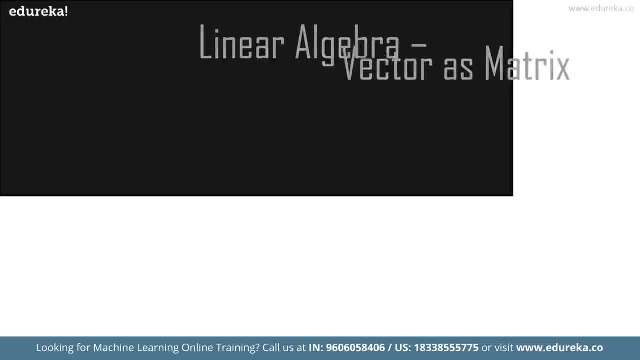 Sharing factor. and then you have the rotation. So how do you rotate your particular object? in which direction? So all of that can be done using these particular matrices. So let's move over and understand how matrices can help you solve equations and, you know, obtain solutions. 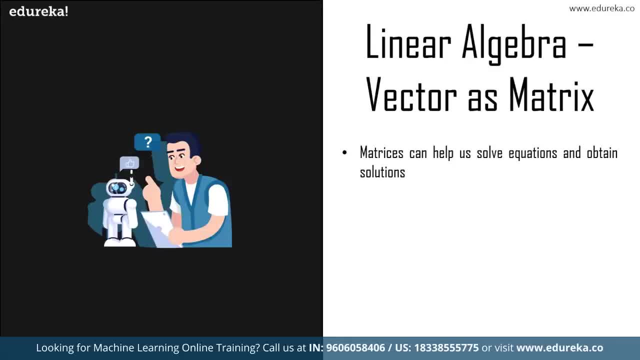 much more easily. So that is basically vector as a matrix fix. We have two methods over here. They are the echelon method and the inverse method. for our tutorial I've been taking the row echelon method Third, because it's much more comfortable for me. 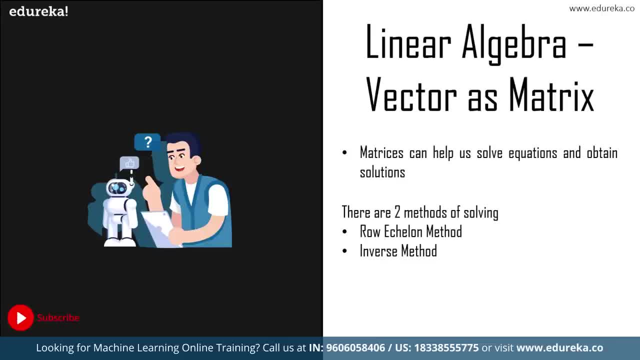 If you are much more comfortable with column echelon method, you can go ahead with that, but because I am comfortable with row echelon methods, I've used row echelon method and next we have the inverse method. So we are basically going to solve the equations. 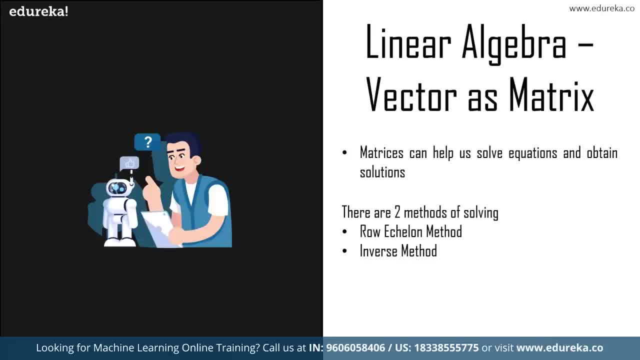 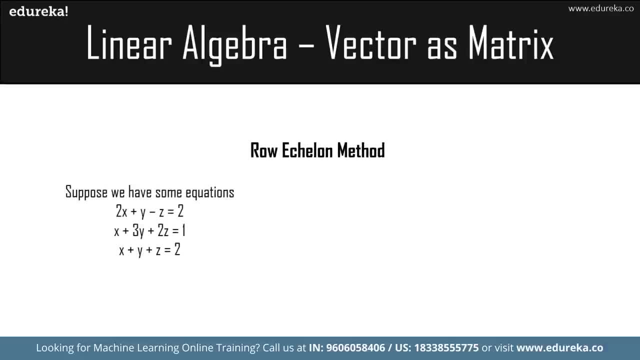 We are going to find the coordinates at which our points give us that particular value. So let's move over with the first method, which is the row echelon method, and I have some equations over here which go ahead like 2x, Y minus z equal to 2x plus 3y plus 2z equal to 1x plus y plus z equal to 2.. 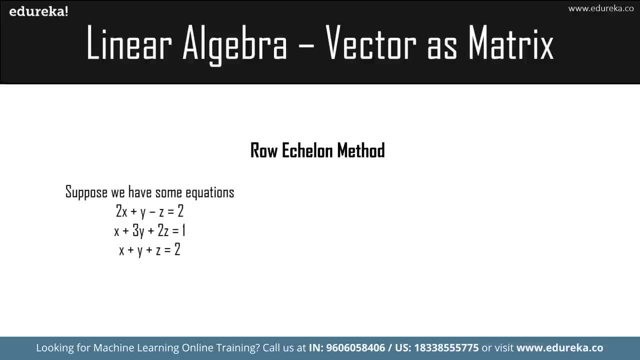 So I'm going to convert all of this into a particular matrix. So let me show you how the matrix looks. It is a 2, 1 minus 2 and 2, 1, 3, 2, 1 and 1, 1, 1, 1.. 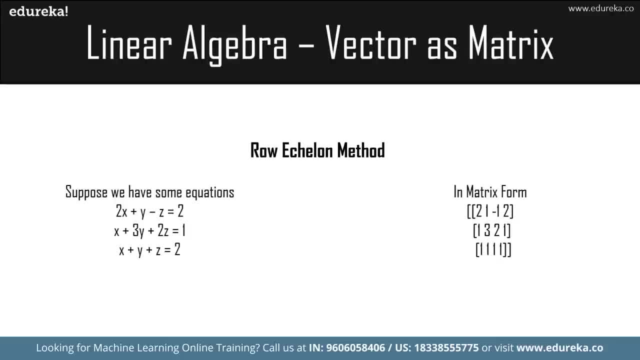 So all the information about the equations have been put into the matrix form, and the answers that we are going to get are: x is equal to 2, y is equal to minus 1 and z is equal To 1. so this is the reason I am going to get all these particular values. 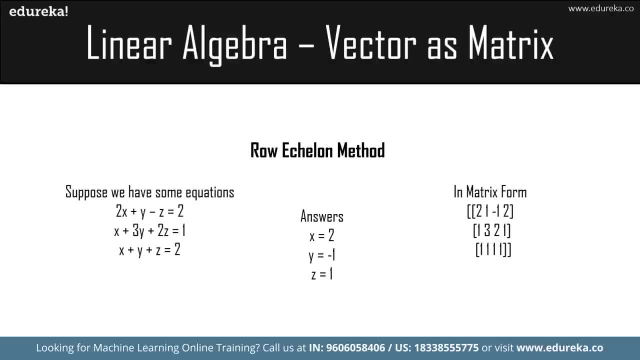 That is 2, 1 and 2, which I am getting from the equations. Whenever I put the x, y and z values into them, I'm going to, you know, get those particular coordinates. Now let me just tell you why we are solving equations. 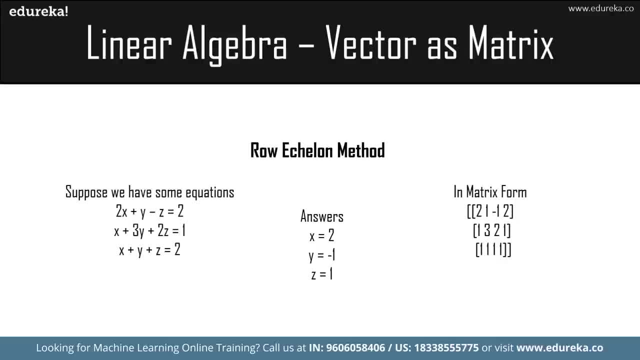 Okay. so if I am telling that there is this particular vector that goes like this or comes in this direction, or something like that, I want to find the x, y and z coordinates so that I can obtain the information, Visualize it and then learn more about that particular vector. 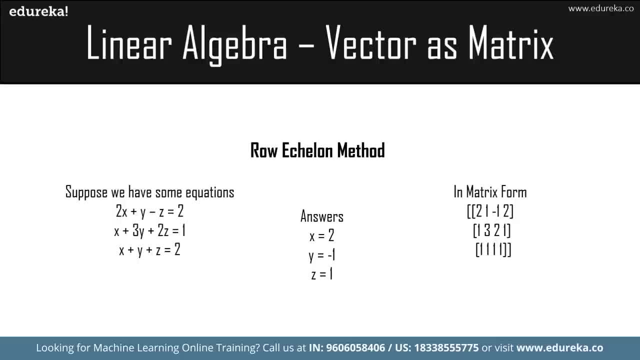 Now see, for example, this is just 2x plus y minus z, equal to 2.. Let's say, for example, if, what if it was a two boxes plus one candle minus one chocolate is equal to giving me a profit of 2 rupees. 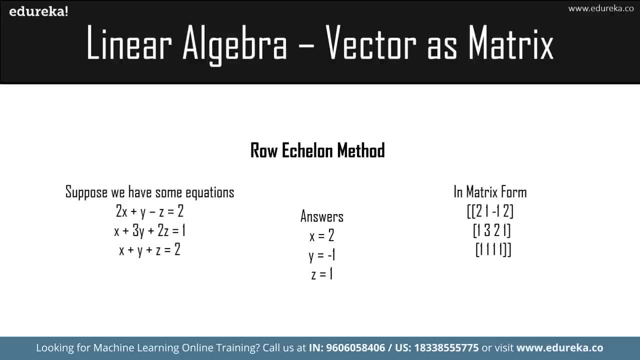 Okay. So, as you can see, these are just simple equations and these are the coordinates that we get. x is equal to 2, y is equal to minus 1 and z is equal to 1.. But what is the importance of this? Okay, 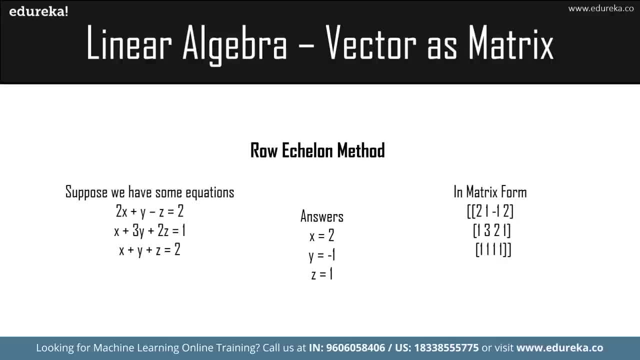 Let me just give you a simple example so that you can understand what we are actually trying to find out over here. Okay, suppose I have a factory and I want to get a profit of 2 rupees and I have boxes, I have candles and I have chocolates. 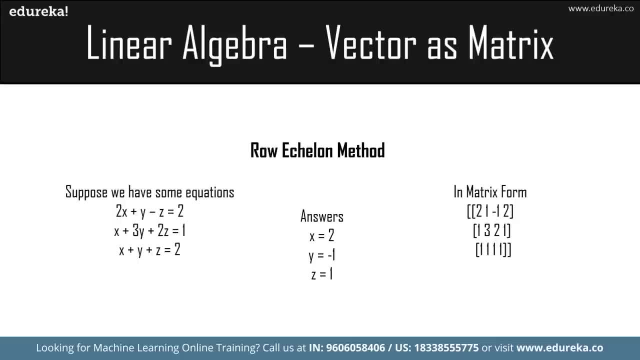 So if I take the first equation, I am seeing that if I have two boxes, one candle minus the chocolate, that it is going to give me 2 rupees profit. So what is x, y and z exactly? x, y and z are the investment costs. 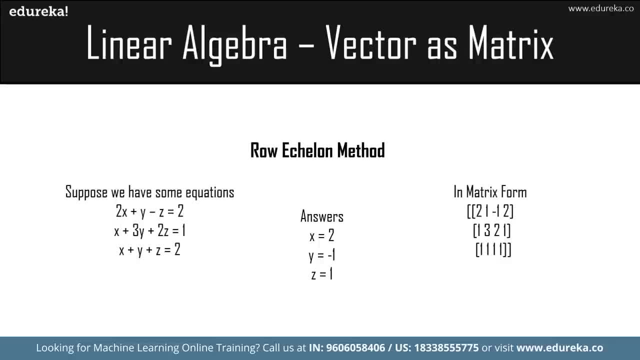 How much do I need to invest into them so that I can get back what I really required? So for boxes, I need to invest 2 rupees. for chocolates, I need to invest nothing. for candles, I need to invest minus 1, or something like that. 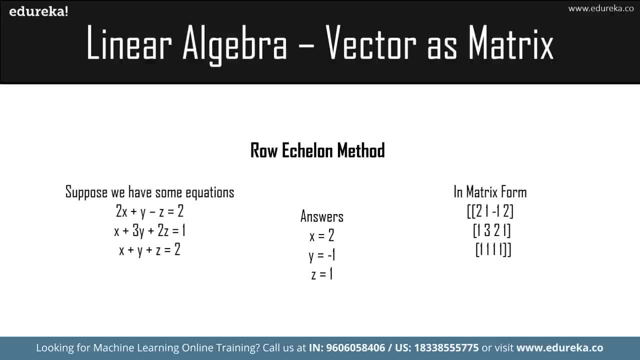 Okay, if I invest so much, I'm going to get 2 rupees profit. So this is like a real-life example which is being converted into some equation and then we just need to solve it. That is the reason Those are so important and how they can be converted into matrices. 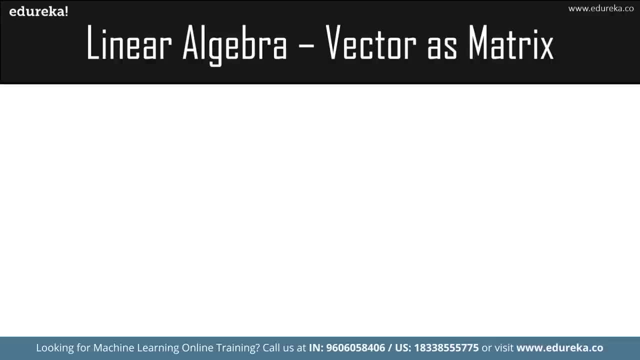 and then you know, solve very easily. How does the row echelon method work? I'm going to be taking the step one, which is r1 divided by 2, r1.. When we divided by 2, we get one, half minus half and one. 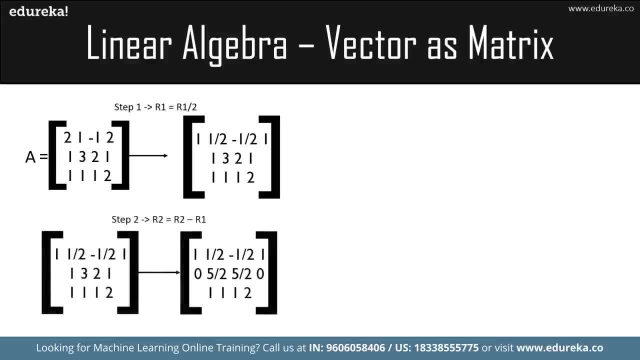 So what's the step to? we will do r2 minus r1.. So we have r2, which is the minus of r1.. I am going to get the particular equation, which is one half Minus half, and 1, 0, 5 by 2, 5 by 2 and 0, 1, 1, 1, 2. simple enough, right. 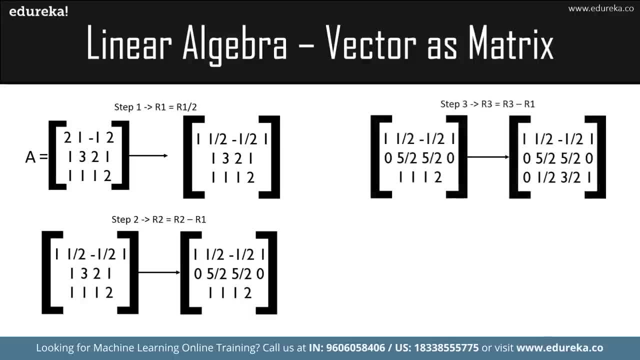 So what is the next step? It will be r3 minus r1.. So it is 1 half minus half, 1, 0, 5 by 2, 5 by 2, 0 and 0, half, 3 by 2 and 1. the next step: 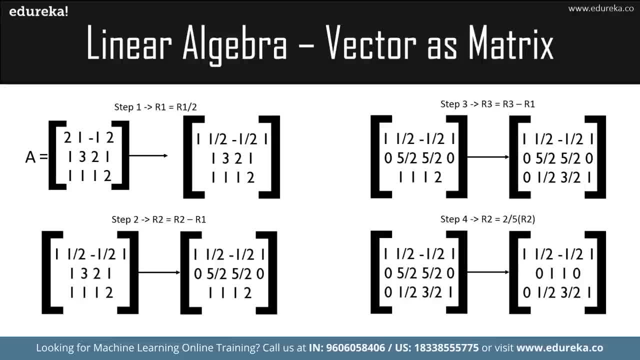 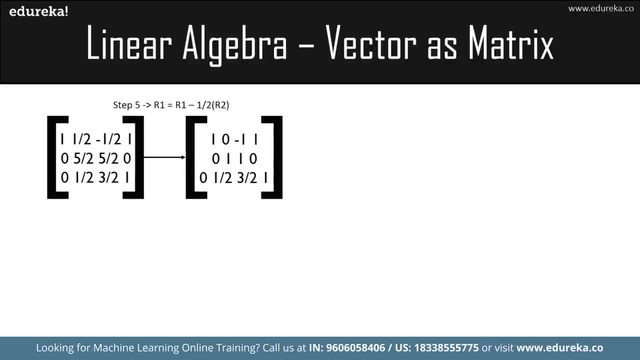 It's 2 by 5 by r2.. So you get one half minus half, 1, 0, 1, 1, 0 and 0, 1 by 2, 3 by 2 and 1.. So what's the step 5? step 5 is basically: 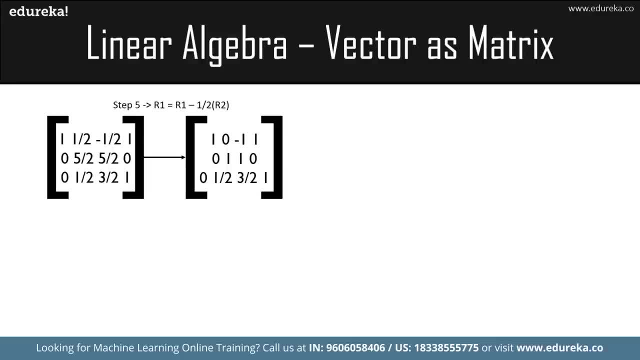 r1 minus half of r2.. So I get 1, 0 minus 1 and 1, 0, 1, 1, 0 and 0, 1 by 2, 3 by 2 and 1.. Step 6 is r3 is equal to r3 minus half of r2.. 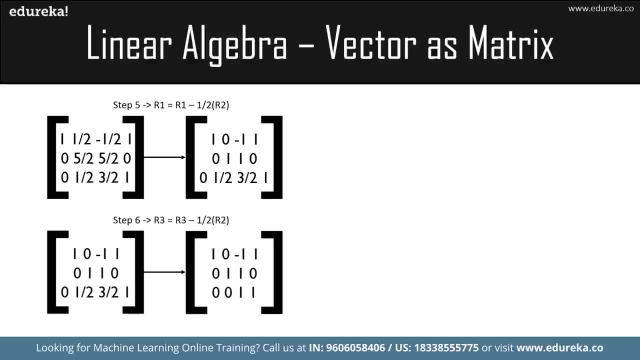 So I have 1, 0 minus 1 and 1 0, 1, 1, 0 and 0, 0, 1, 1. step 7 is r1 plus r3.. So I have 1, 0, 0, 2 0, 1, 1, 0 and 0, 0, 1, 1. step 8 is r2.. 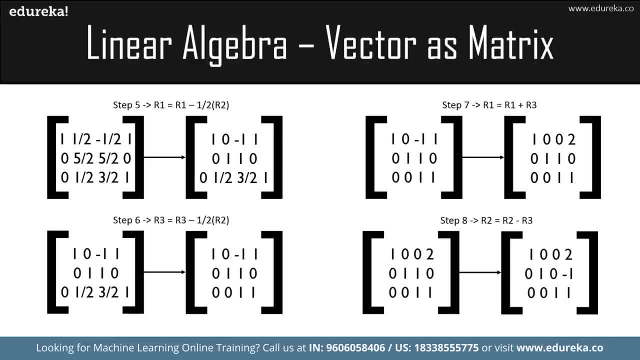 2 is equal to r2 minus r3.. So I have 1 0 0 2 0, 1 0 minus 1 and 0 0 1 1. if you put all of this back into the equation, 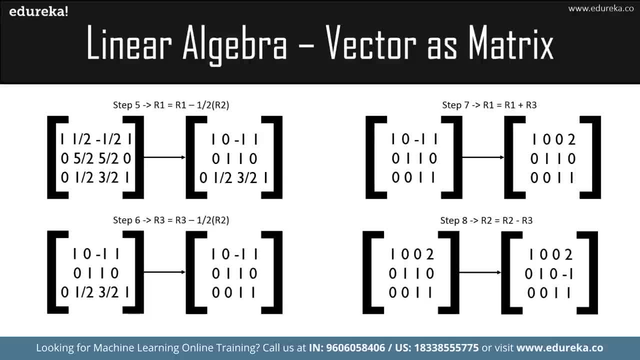 you will find out that for the first row, 1 0, 0, 2 is equal to x plus 0 plus 0 is equal to 2.. The value of x is is equal to 2, the value of y is equal to minus 1 and value of z is equal to 1.. 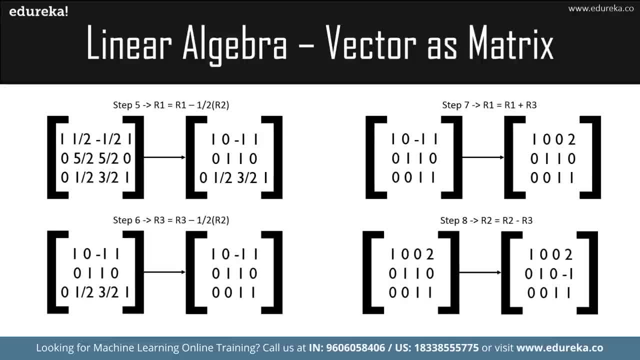 So this is how the row echelon method works, And what Do you have to actually perform in row echelon? It is basically: the first row has to start with the value 1, the second row has to have a 0 and then somewhere in the middle. 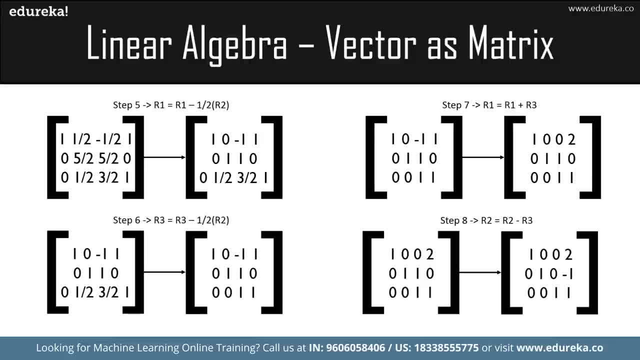 It has to have a value of 1, and then the third row should be starting with zeros and then getting some value where it starts with one only. So row echelon or column echelon- whatever method you use, you have to make sure that whichever element is the first starting element. 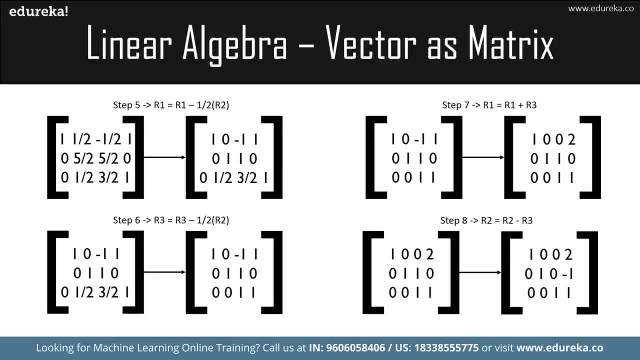 of the row, it has to have a 1 or it has to be preceding with zeros. So, as you can see here, the first row has 1 0 0, 2, and then you have 0 1 0 minus 1, and then you have 0 0 1 1.. 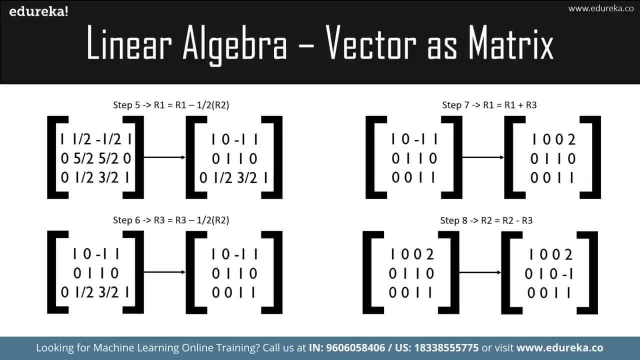 So that is how you are performing the row echelon method to solve your matrix. So, as you remember, we had: x is equal to 2, y is equal to minus 1 and z is equal to 1.. Those were the answers that we wanted, once we are done with row echelon method. 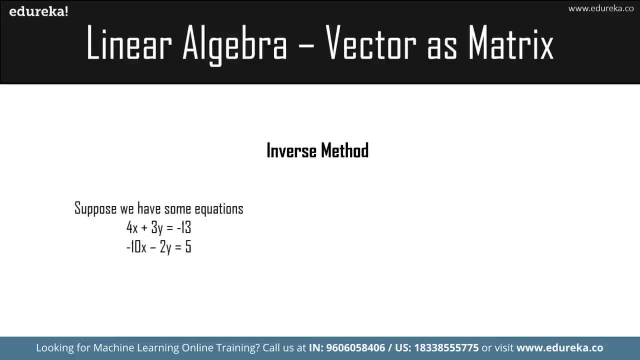 Let's move over to the inverse method. So suppose we have some Equations of 4x plus 3y is equal to minus 13 and minus 10x minus 2y is equal to 5.. What does the inverse method tell us? 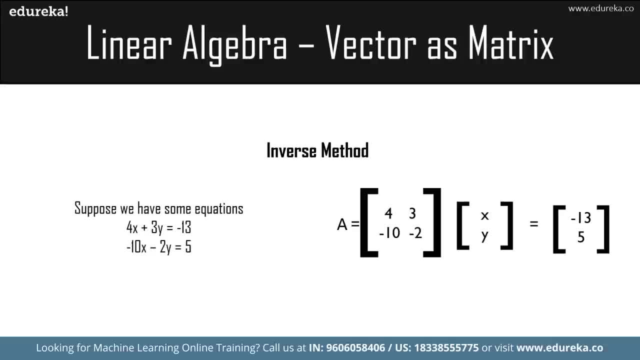 Let me show it to you. So this is the matrix that you come up with. So it is a 4, 3 minus 10 and minus 2, then you have x and y, and which is equal to minus 13 and 5.. 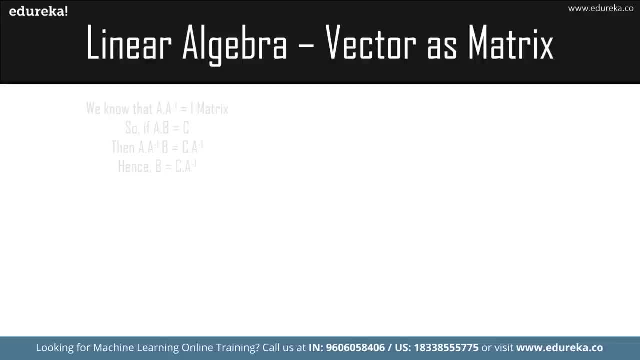 So what does the inverse method actually tell us? For example, we know that a into a inverse is equal to 0 work done right. It is the identity matrix, I matrix. So if I have a into the a inverse, so it is like I'm doing the work. 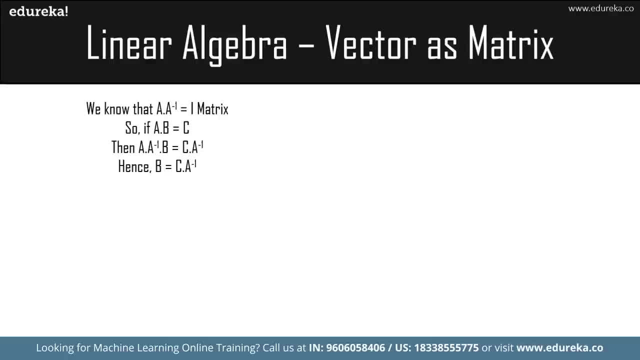 and I don't do the work is equal to no work done. So a into a inverse gives me the identity matrix. if a into B is equal to C, So a is my. you know all the numbers. then B is my x and y and C is the output value. 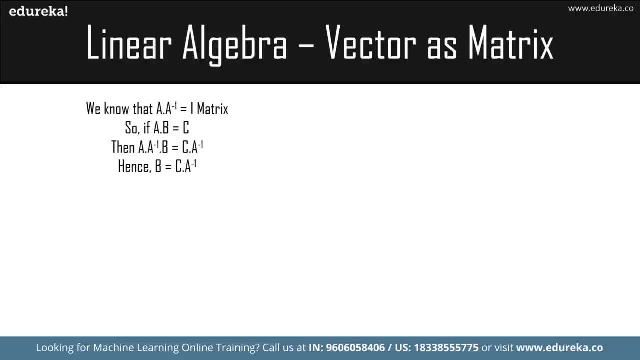 If I do a into a inverse, into B is equal to C into a inverse, I am going to get B is equal to C into a inverse, because a into a inverse gets cancelled. So B is equal to C into the a inverse of it. 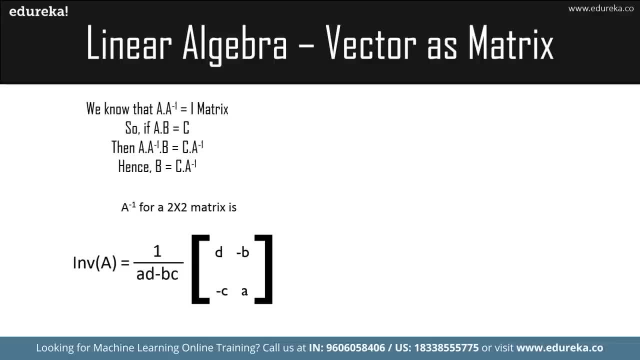 So that's what I'm going to do. So what is the inverse of the 2 cross 2 matrix? The inverse is formed by this formula, and the inverse is actually 1 by 22 minus 2, minus 3, 10 and 4.. 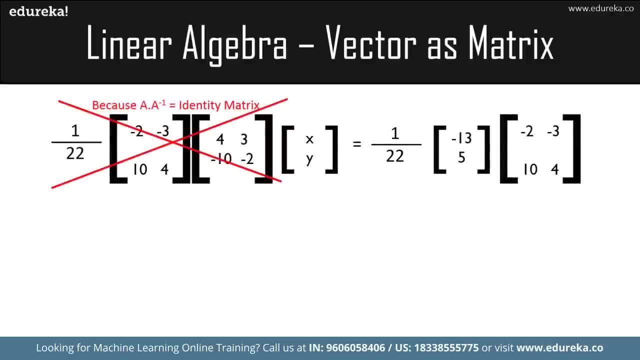 So that's the inverse of the matrix. So let me show you how it works. What happens is I'm having a To a inverse into B is equal to C into the a inverse. So a into a inverse is obviously going to get cancelled out because you know it's an identity matrix. 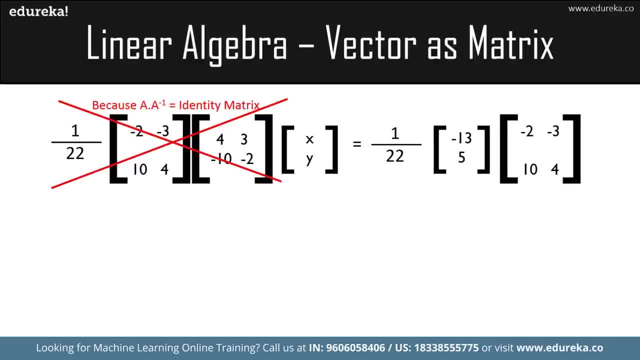 So I'm just going to be left with x and y is equal to 1 by 22, into minus 13 and 5, minus 2, minus 3, 10 and 4.. So what I do later, I'm going to just multiply and this is what I get. 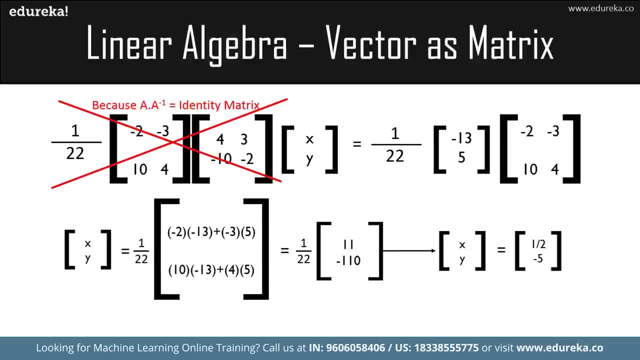 So it's basically 1 by 22 and 11 by minus 110.. So if I do 1 by 22 into the particular Matrix that I found, it is going to be x is equal to half and y is equal to minus 5.. 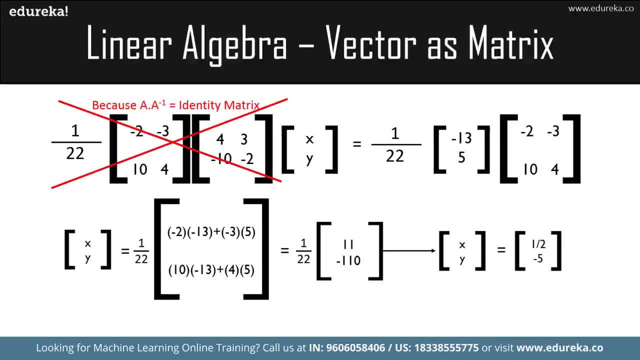 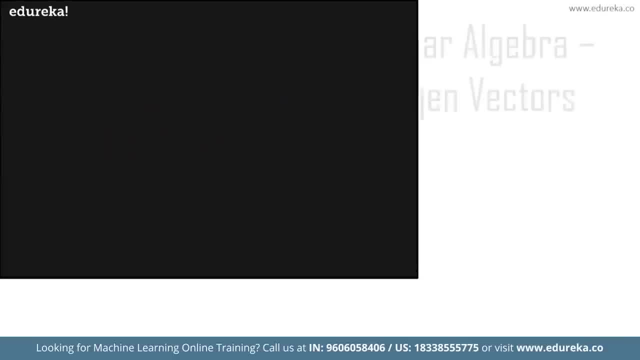 So that is how I'm going to be using the inverse method to find or solve the equations. I hope that was simple to understand. So, once we've done all of that, we are now capable enough to understand what an eigenvector is. 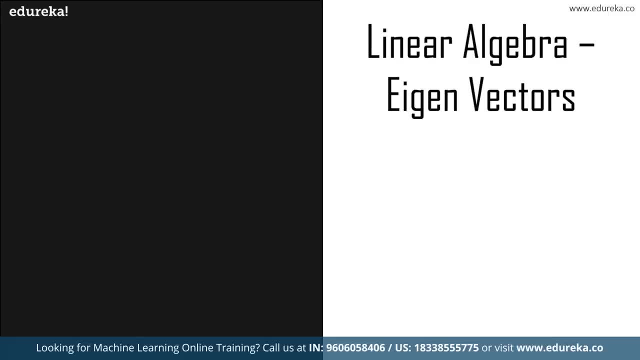 I can. vectors are really important when you're working with data. all of that, what vectors, matrices, what all we've been doing By now. think of it as the data you're working with in your machine learning algorithm. right? What is an eigenvector? eigenvector does not change the direction. 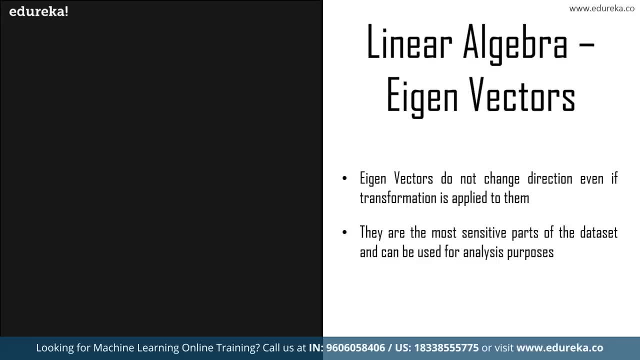 Even if our transformation is applied to it. What does a eigenvector really give us? So, for example, I have a data. if I am trying to do any transformation on it, It should not change from what it was really. it should not change from what it was initially. 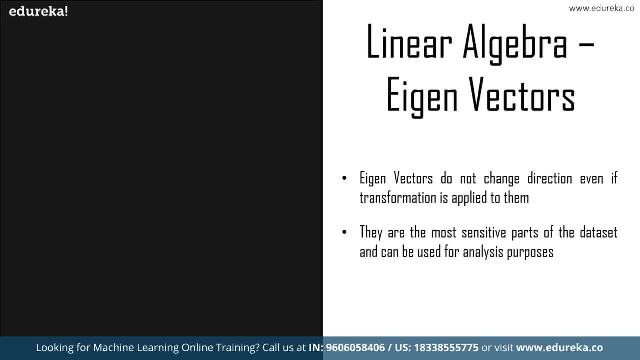 It should not become something that is Totally irrelevant to me. if I have such data that, even if I apply transformations to it, it does not change what it was supposed to be, That is an eigenvector. What does an eigenvector give me? they are the most sensitive parts of my data set and I can use them. 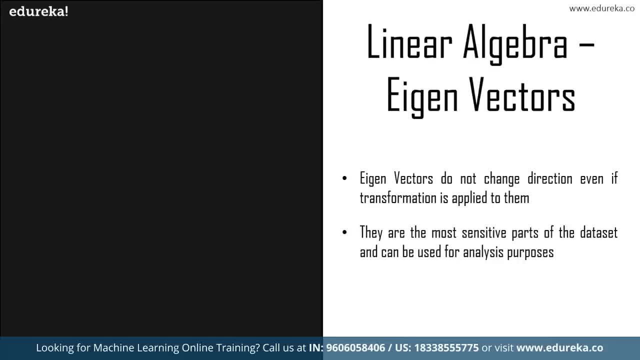 and I can trust them for my analysis purposes. So that is why eigenvectors are so important. eigenvectors help you transform and, you know, make your data much more careful. So, for example, let me show you what an eigenvector looks like. 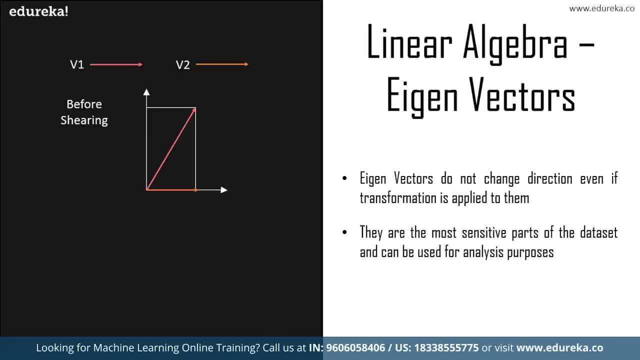 Okay, so I have a particular rectangle and I have a lot of vectors, but for my example, I'm just going to be using two vectors. Okay, I have a v1 and v2. these vectors are basically trying to explain all the data that is there. 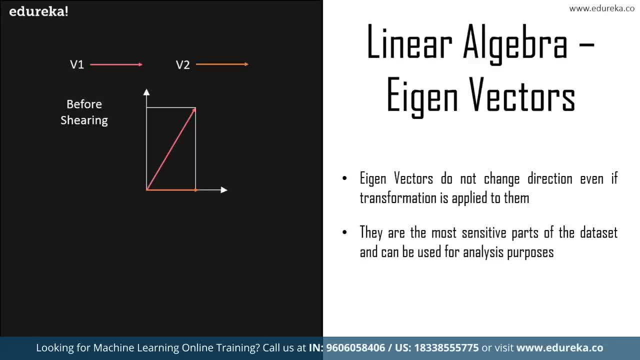 in the particular rectangle. What happens if I perform the sharing operation? when I perform the sharing operation, my v1 vector has changed its direction completely. It was at Some other direction and after sharing or after performing some operation, It has completely changed its dimensionality, its direction, all the information that it held. 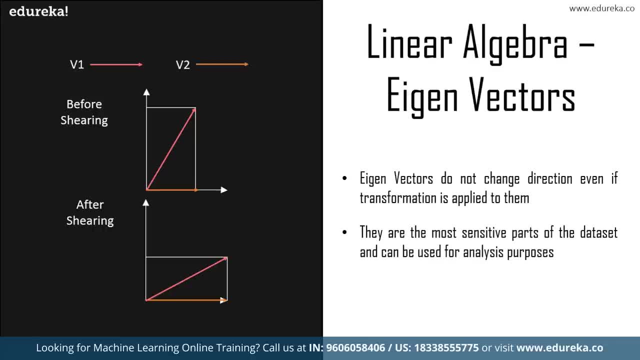 initially- has not completely been changed, Whereas my v2. it has not changed its direction. Yes, it has moved forward. It has multiplied, but it gives me the same information that it was giving me earlier also, So that becomes an eigenvector. think of this now in the form of a matrix. 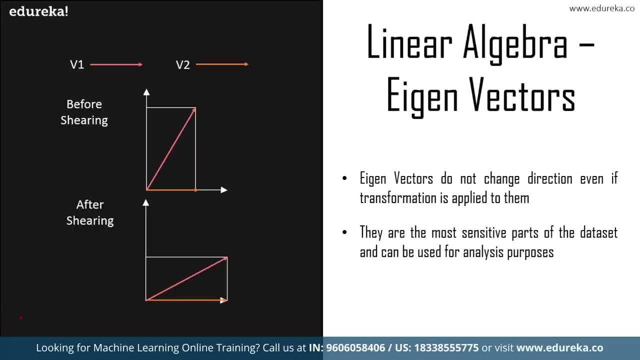 If my matrix is changing so drastically, how will I be able to perform operations on it? It becomes really difficult, Okay. So, for example, think of the vector v2 as a you know list, which is then just multiplied by 2. it does not make a difference. 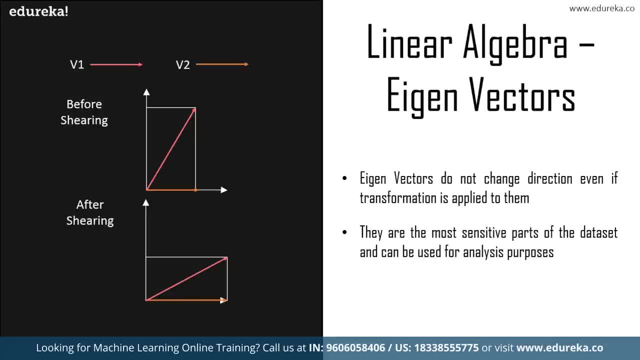 Why? it's because, even if I multiply by 2, it's just going to double the value, but the operation that I want to do on it, the information that it is giving it to me, That's the same. So that's the reason eigenvectors are so important. 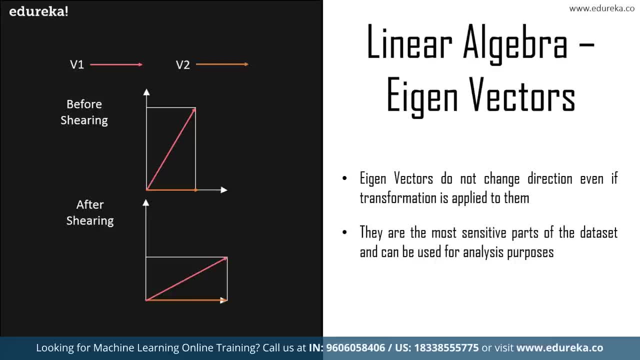 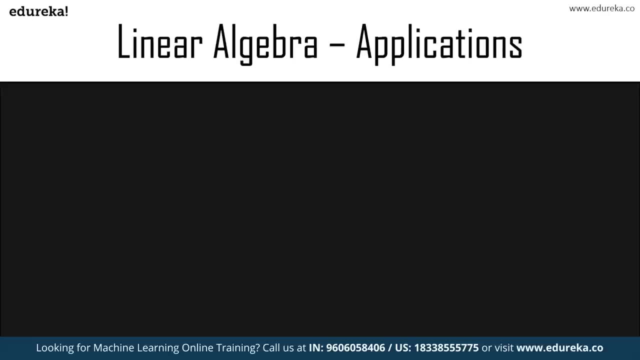 And what are eigenvalues? the values that we perform on these eigenvectors are all that are eigenvalues. It's that simple to understand. so that is all you need to know about eigenvectors. all the data which is not transforming Anything is basically the data that you should be learning with. what are the applications? 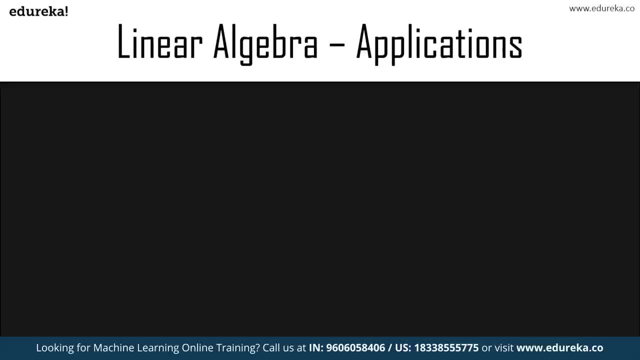 that linear algebra helps us with. you have the first and foremost, which is the principal component, analysis, PCA. It is used for dimensionality reduction and it helps increase the quality of detail. Then you are working with applying transformations. It helps in encoding, it helps in the single value decomposition. 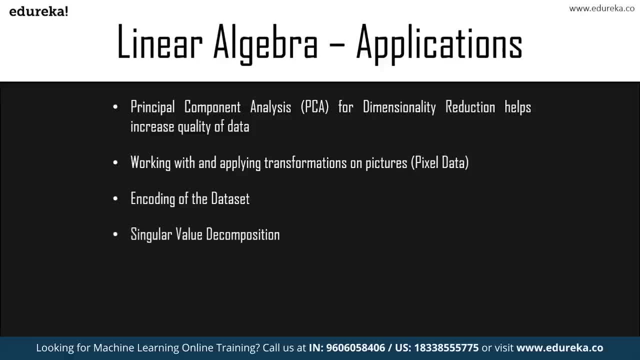 where it is again reducing the dimensionality of a single value data, and then it is used for natural language processing, for latent semantic analysis, optimization of your deep learning models. All of this can be achieved through linear algebra, So it is a very important aspect of machine learning. 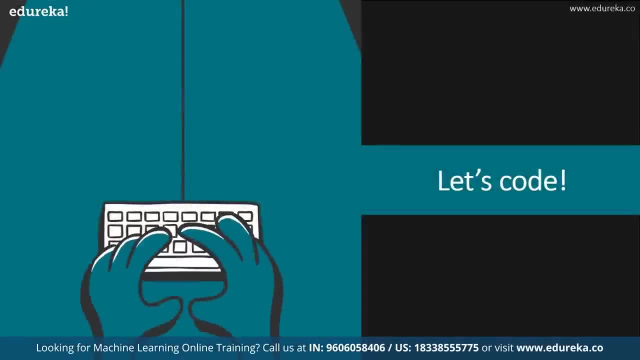 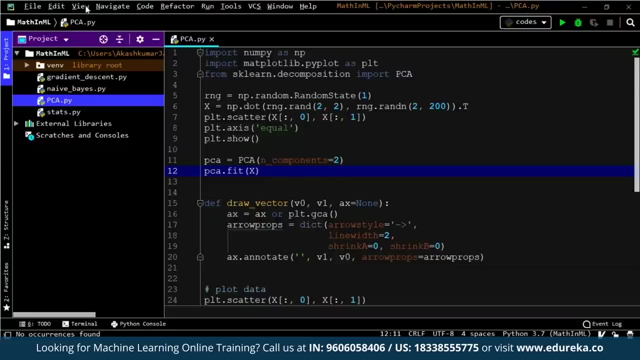 Once we are done with all of this, let's start our coding for PCA. We will now be coding for principal component analysis. Let me show you how it really works. So I am having all the programs already prepared for you guys, So we do not extend this big tutorial even more further. 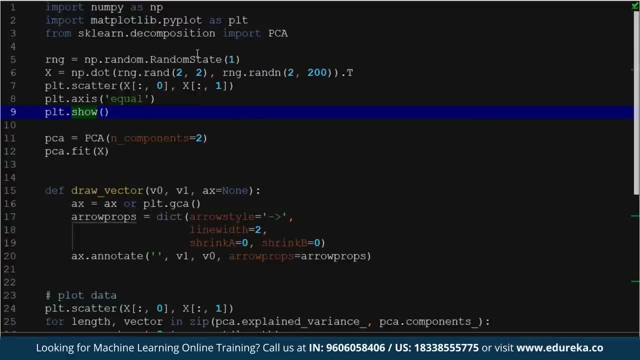 Let me go to the presentation mode mode. So what happens over here is: I am having these important, Which are important umpires NP, then I have the pi plot as PLT and then from Escalon dot decomposition import the PCA. So principal component analysis is already present. 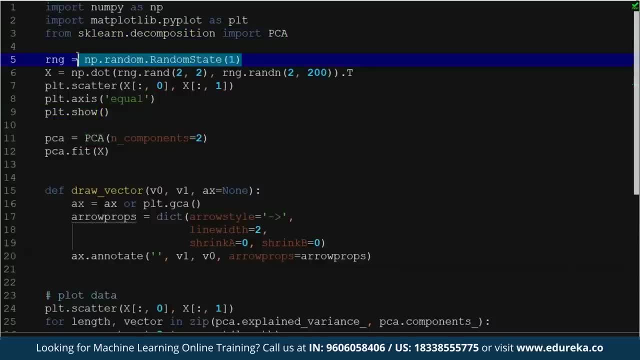 I'm just going to import in from Escalon, So I'm going to get a range of around you know, 200, 300, how much ever it is. after I'm getting that particular range, I'm going to get data. I'm going to get all of that data. 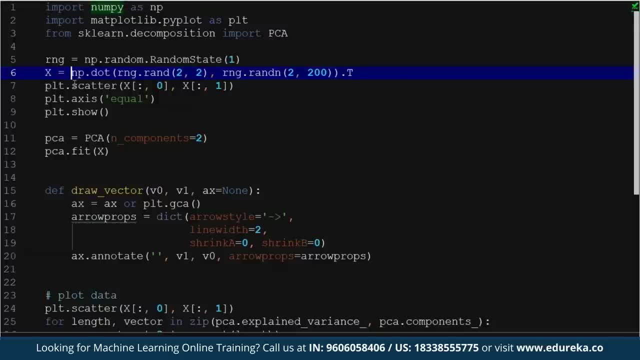 and then I'm going to put it into my particular list. So what happens over here? I have NP, dot, dot and in the range of 2 comma 2, and it is in the range of 2 comma 200.. So in the range of 2 comma 200,. 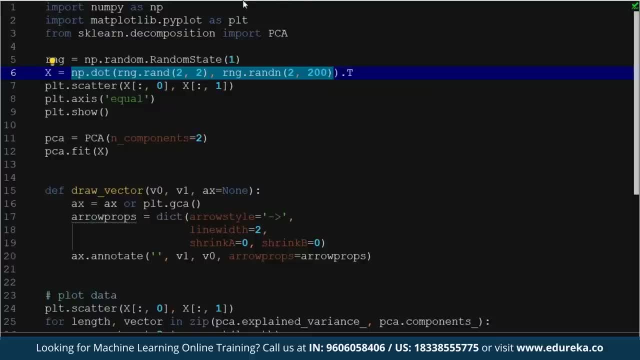 whatever numbers that you can randomly generate, please give it to me. and then dot T. Why is it dot T? It's because all of this which I'm going to get is basically in the form of a column. I do not want it in the form of a column. 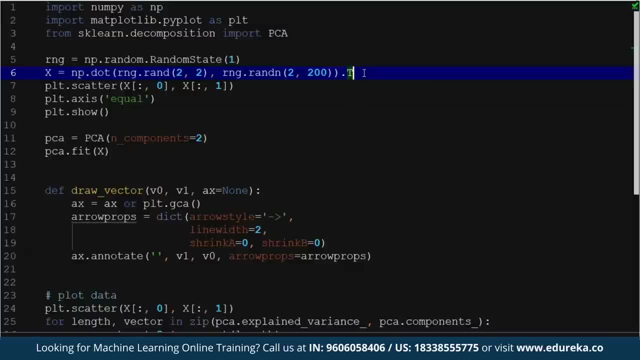 I want it in the form of a row, So that is the reason I'm using dot T. dot T is used to transform one, So I'm just going to scatter that on the plot and then show it to you guys. that is what this particular 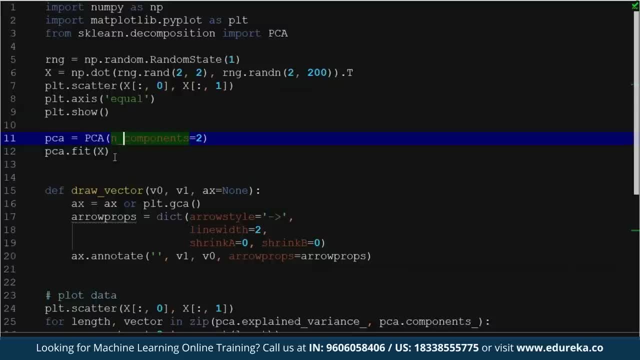 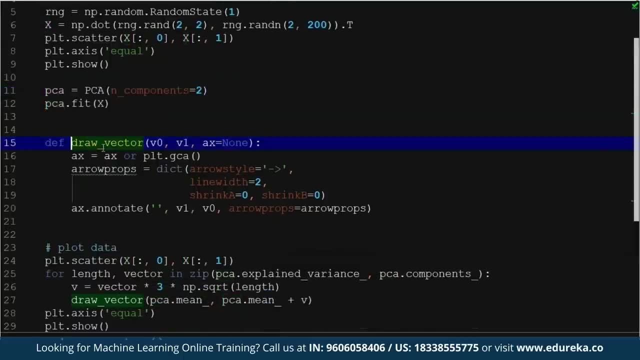 function does. and then I am doing: PCA is equal to PCA of n components is equal to 2, and then I'm going to fit the data into it, And then I have a function which is to draw the vector. So I'm going to do arrow props, dictionary style, all. 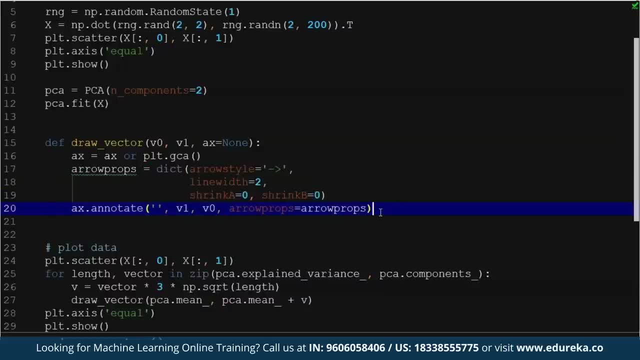 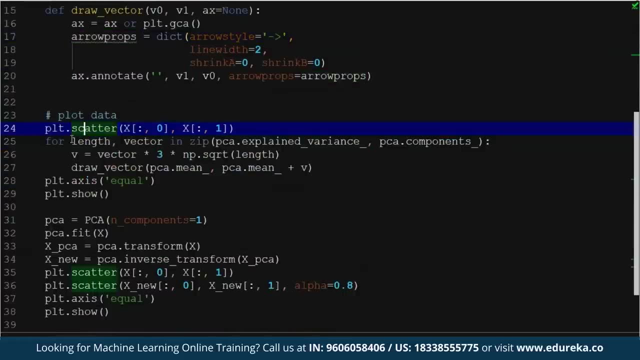 of that. I've just given the styling over here and then I'm going to annotate and draw it accordingly. So this is my drawback to function, and then I'm just going to scatter, plot everything that I had. so I have the vector. How am I going to get a vector? 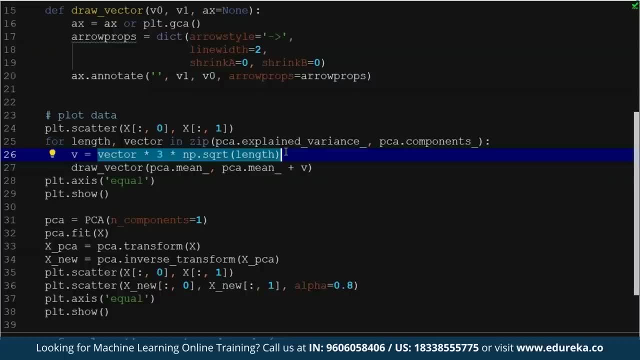 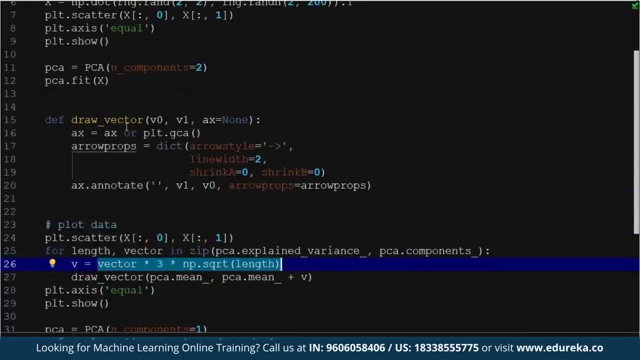 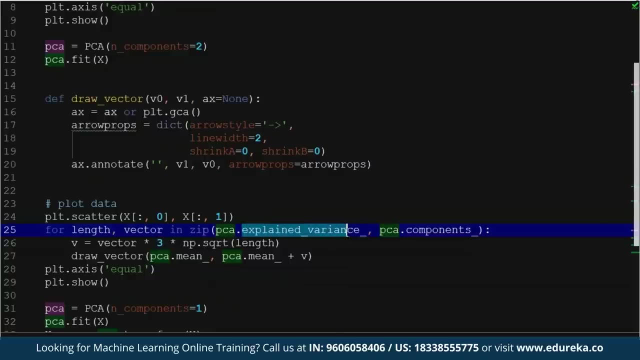 It's using this particular formula, which is the vector, and three and NP dot sqrt. So what is a PCA? explained, variance and components. Okay, So, if you remember, I had fit PCA with the data that I have generated, right. So explain variance is basically going to tell me how much. 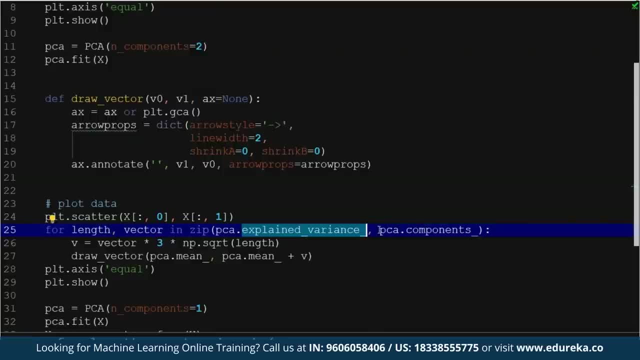 is the variance between my data points and what are the components that are really required that I look at and perform my analysis on them. So these are what the required components are for me, And after I do all of that, I'm going to get another vector. 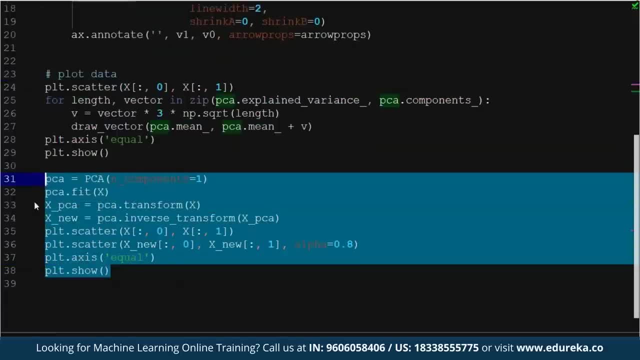 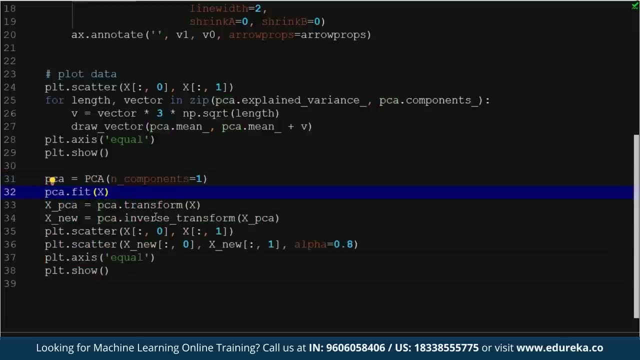 I'll show that to you guys, and then what I'm going to do is I'm going to find one component only over here and I'm going to fit the data, Okay, and I'm going to transform and perform the inverse transform, so that I am going 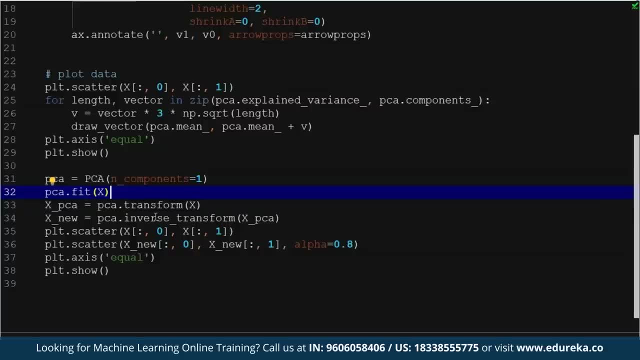 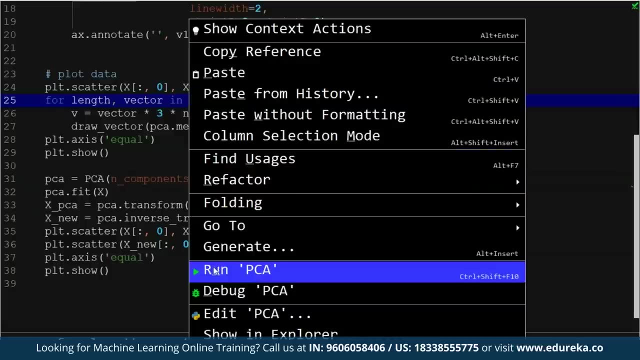 to get a particular linear line which I can just look at and find all the important Aspects of the data that I wanted to from it. Let me run the program and let me show you all the outputs. So, as you can see here, 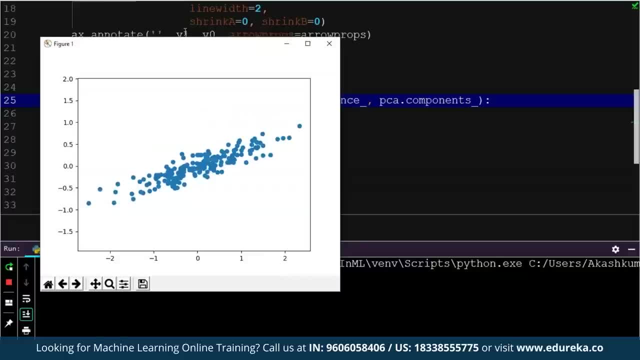 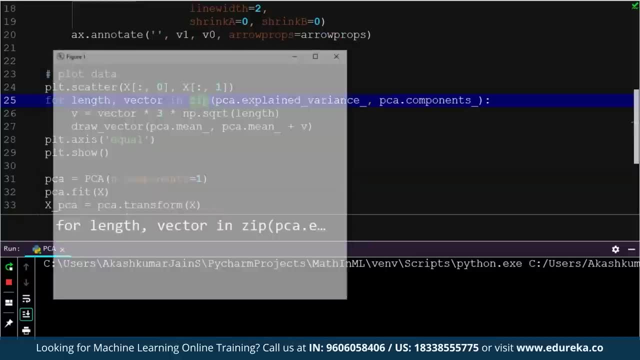 this is all the data that I had generated using the dot function of the random generating thing. So this is all the random data that I have generated. Then what I did: I had to find out two components, right. Then what I had to do, and I had to find out two components. 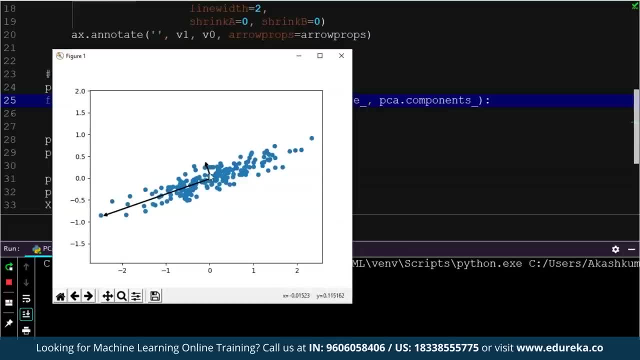 What can I understand from this particular information? This one is a small vector, So this small vector means that this is the only amount of information that it can give, whereas this vector is so long. what this means is that the longer the length of the vector is, the more information. 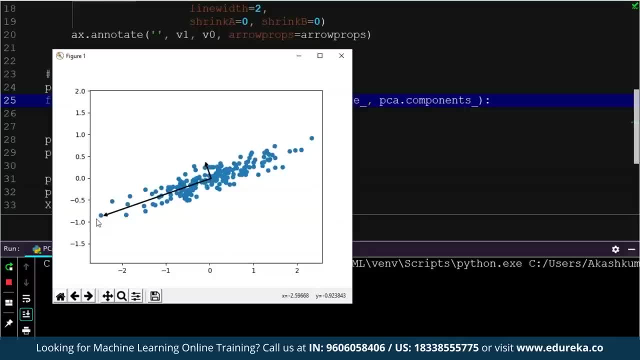 that it can pass to me. simple enough. right longer the length of the vector, the more information that it can pass to me. So what all information I have through this particular vector, all of this is going to give me the best for my analysis. So that's what I'm going to do. 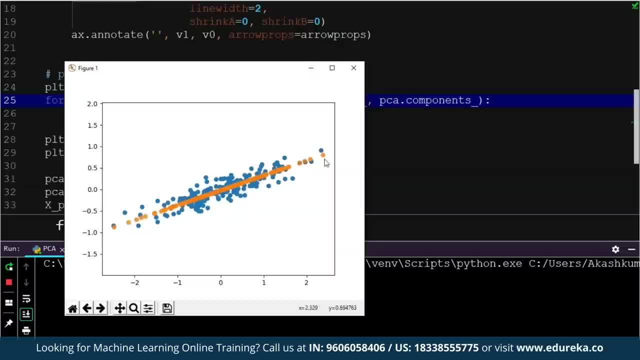 I'm going to get all the data points that are according to this vector. So, as you can see here, all of these data points are very, very important for my analysis. So this is how I converted such a big, huge data set into one particular line. 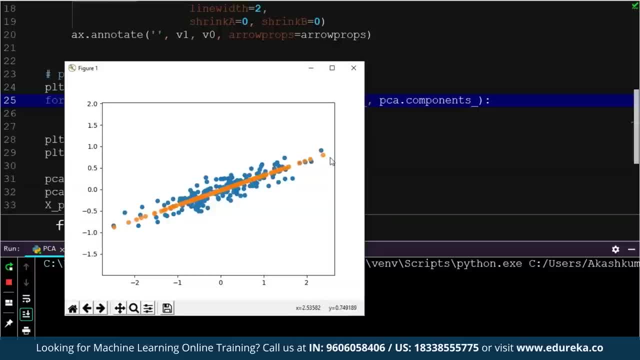 And if I follow all these points, I'm going to get almost the same amount of information. The whole data set is going to give it to me. as you can see, this was such a huge data set, but it's just come up to this one line. 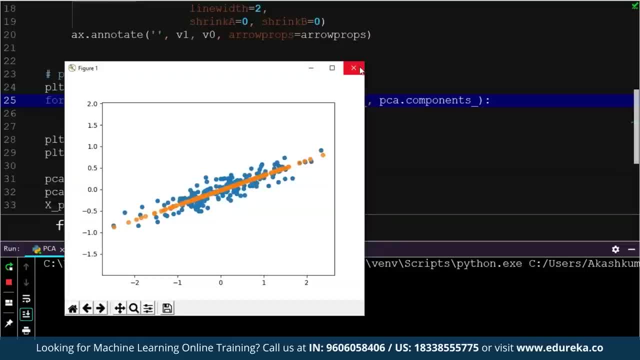 It's so easy. think, if you're working with tons and tons of data. it becomes really, really difficult when you're working with it. That's the reason: use PCA and it's just not use PCA. Make sure that you are able to reduce the data as much. 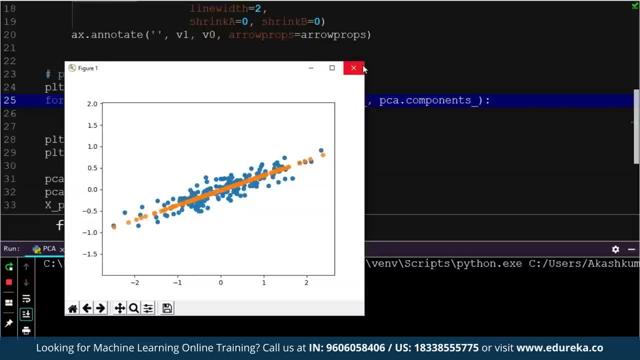 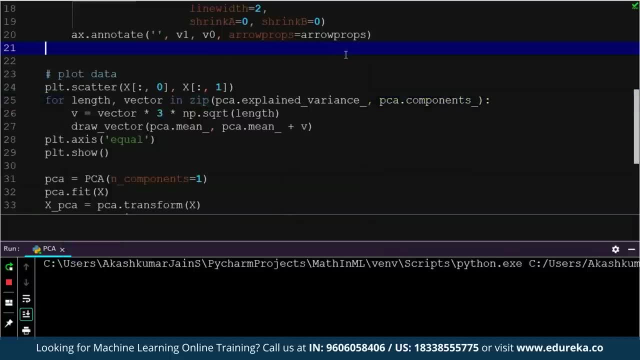 as you can so that you can get at least all the amount of information that you can from that particular data. You do not need all the data, but you need the information from that data. That is basically how PCA works. Hope it was clear to you guys. 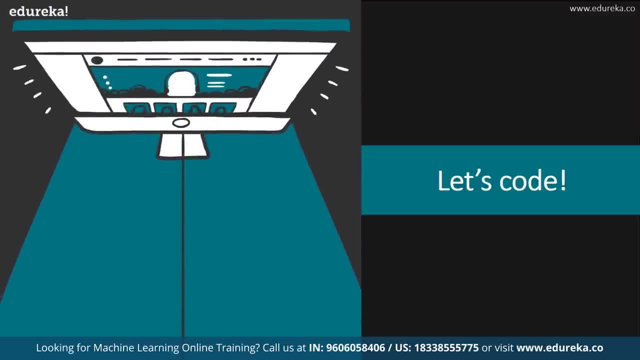 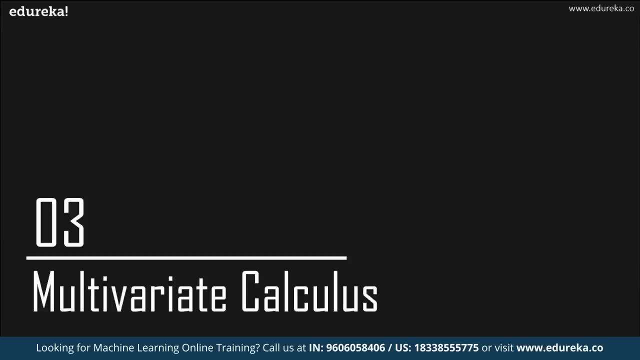 So basically, that was all we needed to learn from linear algebra, and I hope it was clear to you guys. So now that we know all about vectors, let's move over to multivariate calculus. multivariate calculus is one of the most important parts of the mathematics. 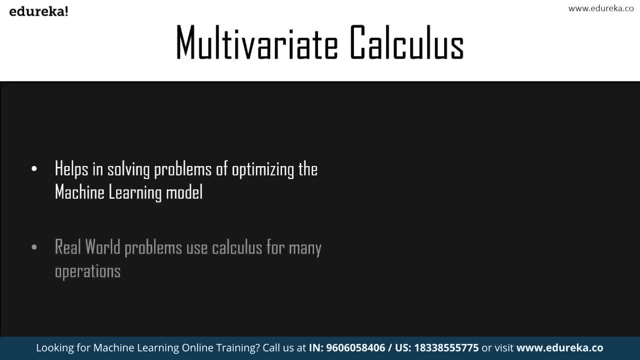 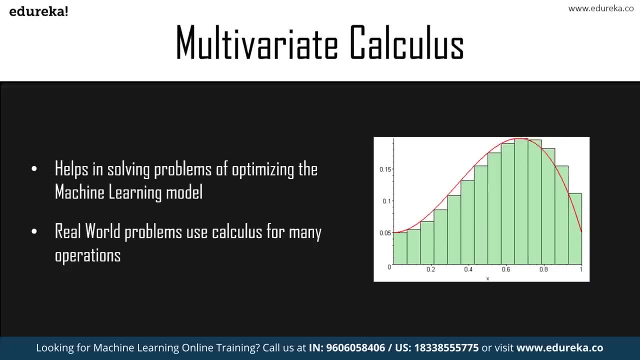 in machine learning. It helps us solve the second most important problem that we were facing in developing machine learning models. The first problem is obviously the pre-processing of the data. The next is the optimization Of the model. multivariate calculus helps us to optimize. 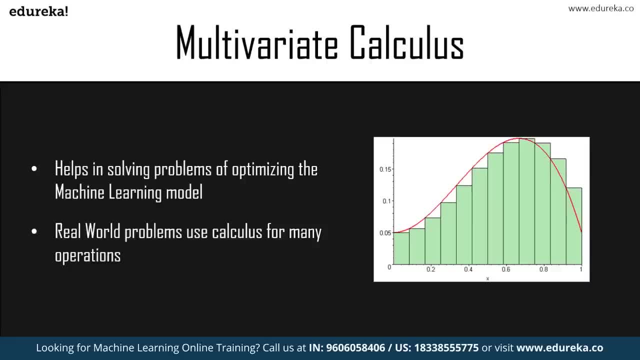 and increase the performance of a model and give us the most reliable results. So how does something that almost half the class hatred help us solve such a problem? So let's break all the eyes that surrounding this, but before that we need to understand the basics. 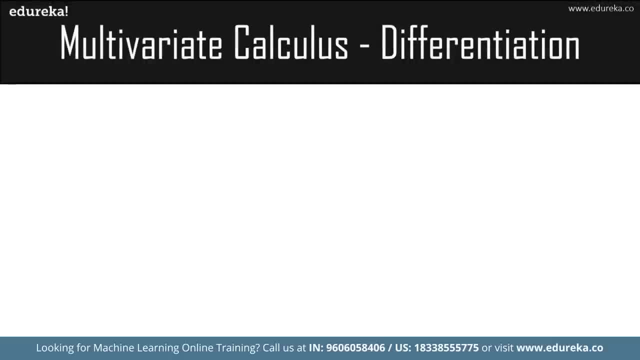 So let's calculus. So the first topic in calculus is a differentiation. differentiation is basically breaking down the function into several parts so that you can understand Every element and analyze it in depth. They're very helpful in finding the sensitivity of a function to the varying inputs. a good function gives you a good output. 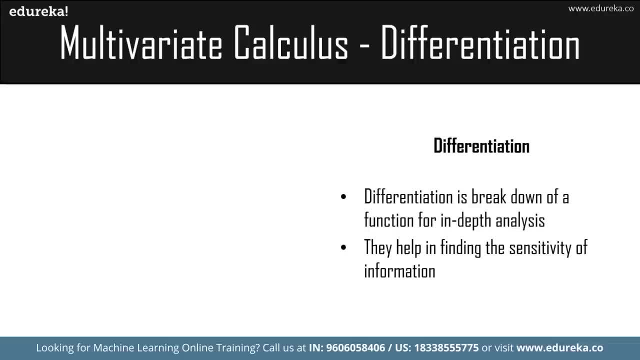 which can be described using a rather easy equation. The same cannot be said for a bad function. So for example, right here I have: y is equal to e power x. It is really easy to tell that. okay, if it is e power x. 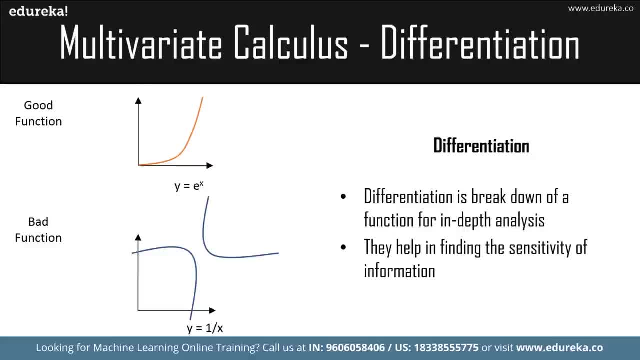 this is going to be the graph for it. But look at, y is equal to 1 by x. it is such a horrendous graph that I cannot explain it Using a particular equation. Those are the types of equations. Those are the good functions and the bad functions. 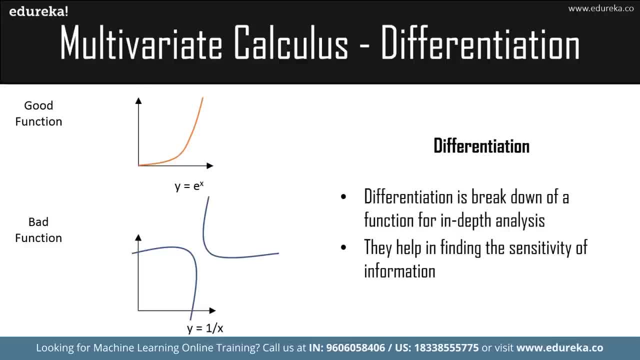 We know all of this, but what are we really after? So let's do all of that right now. Okay, So most of us already know all of this, but what are we really after? So let's understand that with a really simple example. 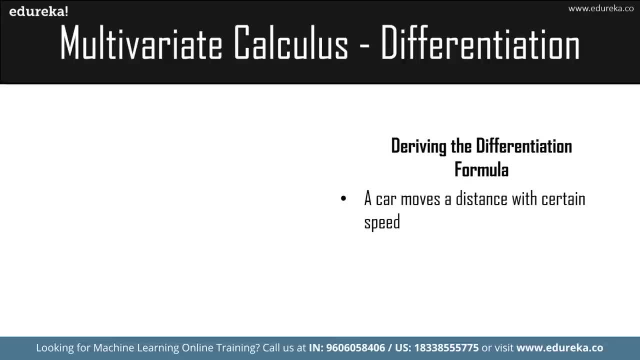 So let's assume that we have a car moving in a single direction only and is already in motion. So if we plot a graph of its speed versus time, it communicates to us how the speed varies as the time keeps increasing and it holds after a certain point. 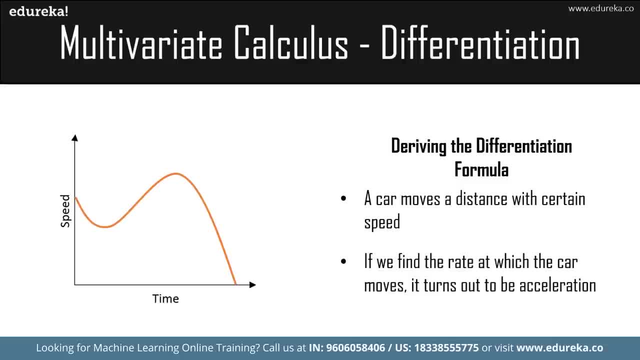 Now, if you want to know the rate at which the speed varies with respect to the time, it turns out to be that we are actually finding the acceleration. the acceleration of the car can be plotted as follows: So what this means is that acceleration is actually a. 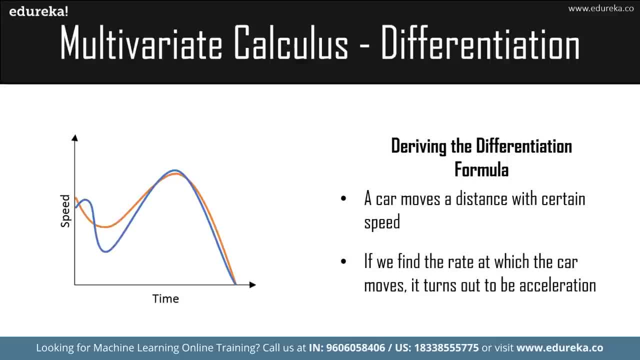 derivative of speed, because the speed we have here is just the magnitude and does not hold any more factors. just for simplifying. So if there was no speed, there would be no acceleration. It's simple as that. now that we have the acceleration, we can justify whether the car had a wearing or a constant change in. 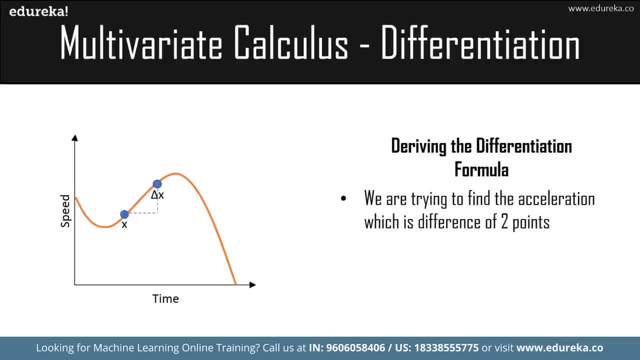 its speed, whether it was moving or not, and much more. but in this case that is all. we need nothing. that you want to find the change in acceleration between a certain range in our time span. Okay, we mark two points, X and some variable, which is a small. 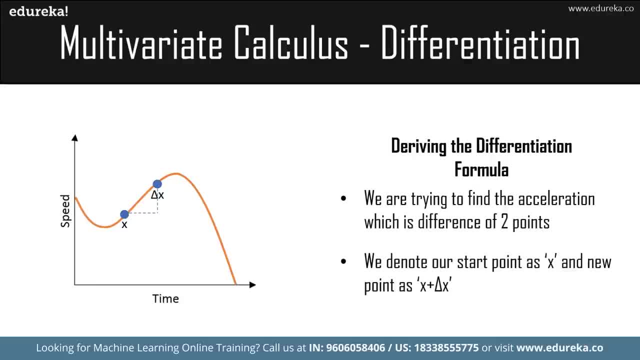 portion more than X. we can denote this using X plus Delta X. So let's denote this on the graph so you can see it as it's shown over here. Now we know that this range has many values in between, but what if we want to know the rate of change only between one? 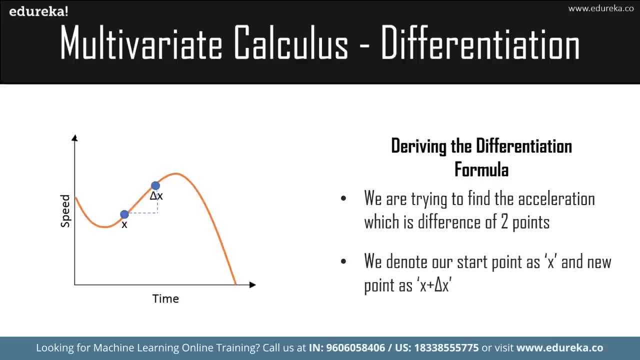 point and the next. we know that this is really kind of impossible because between a range there are countless numbers as the function is continuous. thus, be approximate that the limit or the step between two input variables is zero. Remember that this zero that we are assuming is only the small. 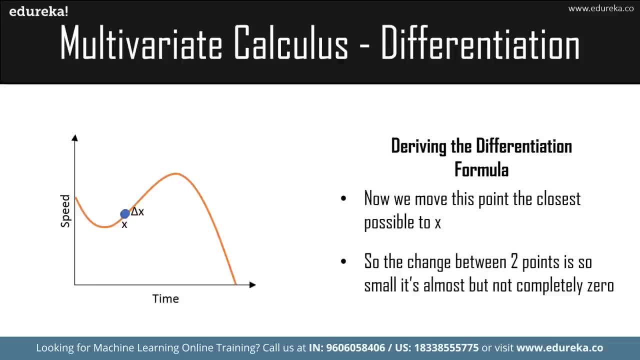 is possible value that we can make up, and it is not the absolute zero. If we ever work with absolute zero, we would never have had any functions at all. So if you are still confused, this number is basically some value of 0.00000. it just keeps going and then some numbers ahead, but it 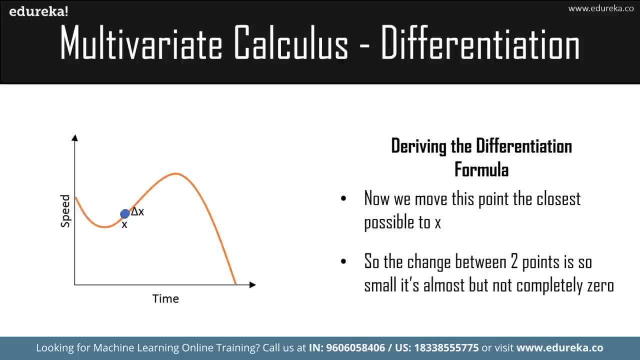 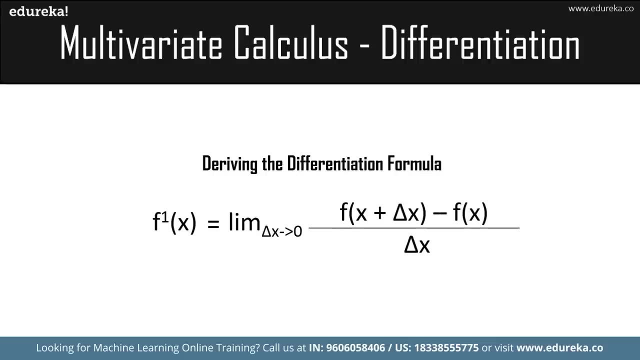 is never really zero. That is the only way that we can put this as okay. So now that we have understood what we are really trying to find, let's make it a general The equation, so let's derive the derivation formula. So the derivation formula is: f dash of x is equal to limit Delta x. 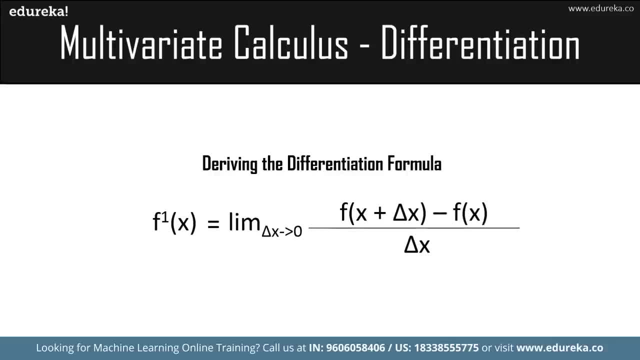 tends to 0, which is not exactly 0 part. We are assuming it to be 0 point something. So we are just going to write 0 and then we have f of x plus Delta x minus f of x divided by Delta x. that is how the formula comes into. 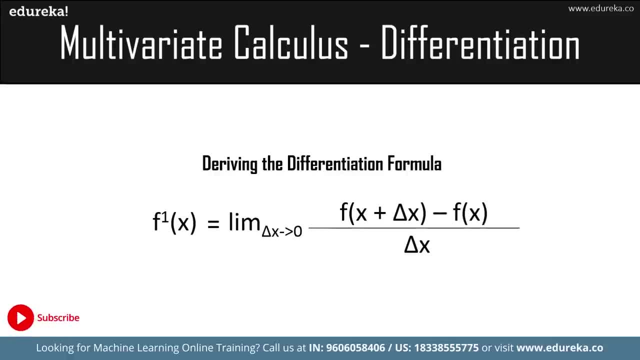 existence. This helps us find the rate of change between one point to the other. It is such an important concept As it plays a huge role in the optimization of machine learning models. You need to understand that this is the first order of derivation. only if we differentiate, the output of the first differentiation. 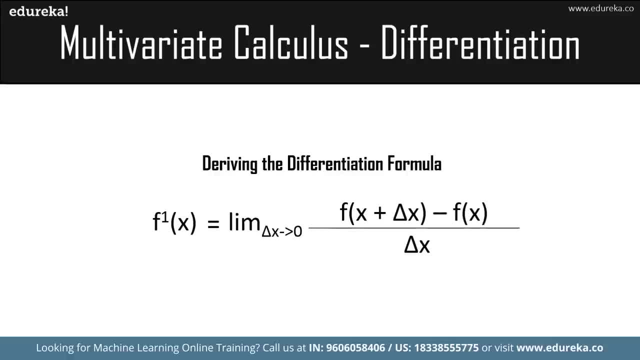 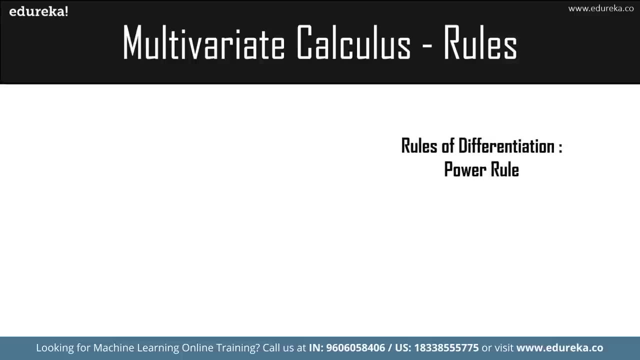 it becomes the second order, differentiation and so on, but that is all the introduction we need from differentiation. So now that we have the basic idea and formula of derivation, let's move over and understand some of the important rules that we need in differentiation. So the first tool that we will be talking about is the power. 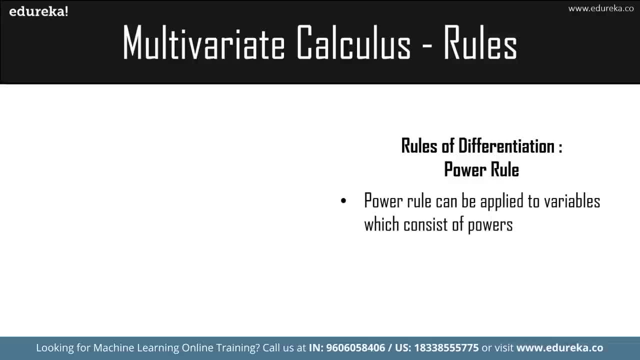 rule. So whenever you have a function which has a variable with some power, you can basically use this formula and solve the equation much more faster. So, for example, let's say that I had a equation called as f is equal to 3x square. 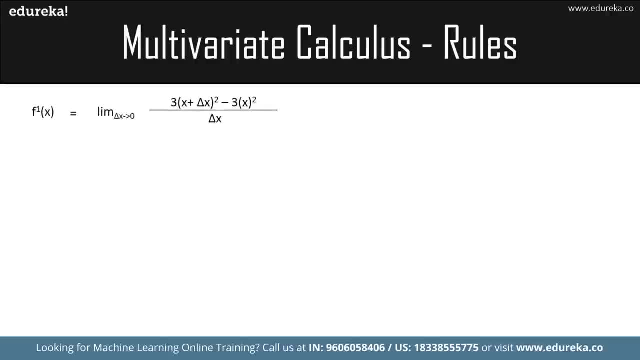 So let me put this into the formula. So I have f. dash of x is equal to limit, x tends to 0. 3 of x plus Delta x, the whole square minus 3x whole square divided by Delta x. So x plus Delta x, the whole square becomes a formula. 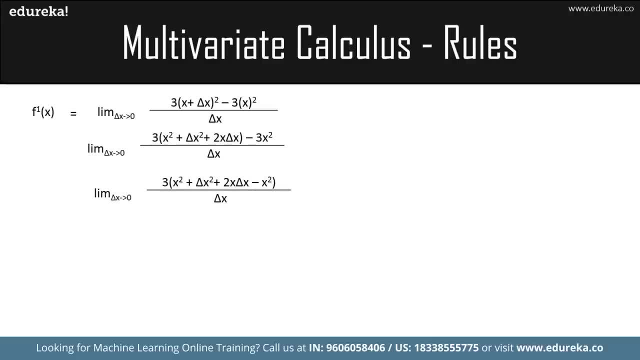 Let me expand it. and then this is what I actually get: plus x square and minus x square get cancelled. and then I have Delta x, which is being removed out of that. So Delta x and Delta x also get cancelled. Then I have 3 into Delta x plus 2x. 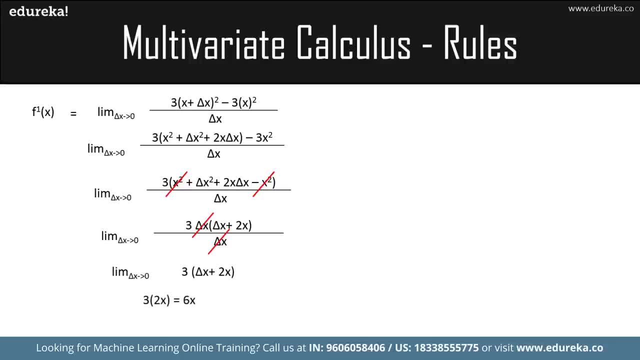 So I'm going to put the value of Delta- x is equal to 0- into the equation, which is not exactly 0 part- It is so small that I can ignore it. So I have 3 into 2x, which becomes 6x. 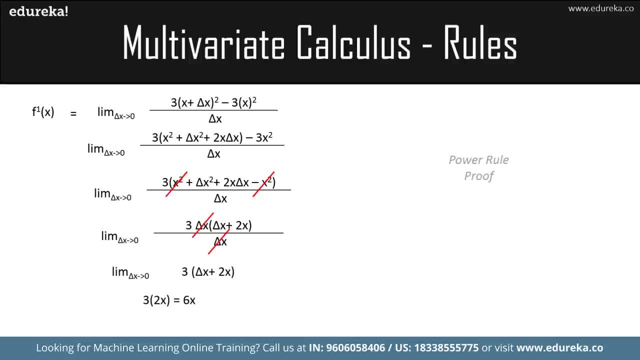 So that's how I had to solve the whole Entire equation, right? So what about the power rule? power rule is just 3 and whatever number I had right. So if it is a 3x square, let me take out 3, because 3 I am going. 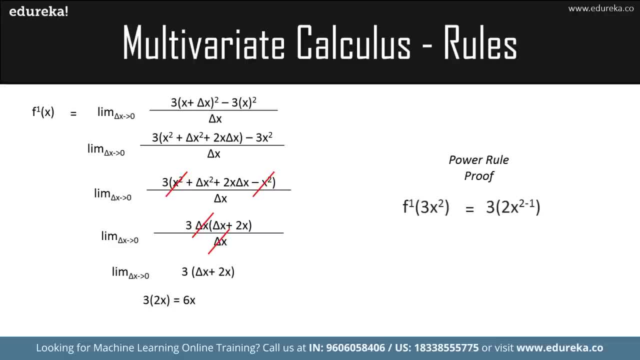 to treat it as a constant, So x square, so x to the power of 2.. So then, what I do? I bring 2 down, which is n, and then I have x of n minus 1.. So it is 2 minus 1, so it becomes 3 into 2x, which is equal to 6x. 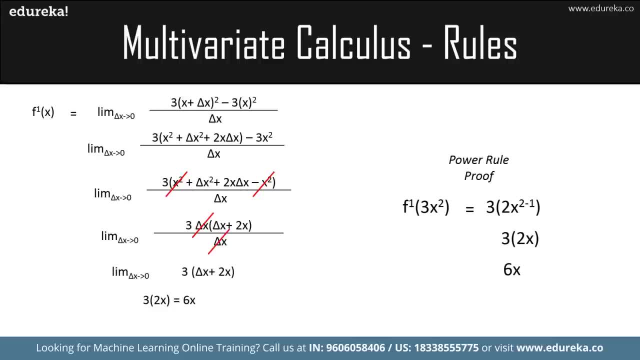 So I get the entire Same answer, but I just had to do it in three steps. I can actually do it either in one step, but just for simplification I've done it like this. The next rule that we are going to be studying is the rule of sum. 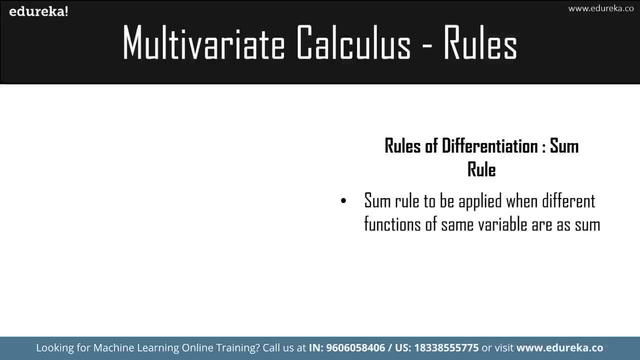 So if you have a particular function which is the sum of two variables, their differentiations, some also is the differentiation of the whole function. So if you have f of x1 plus x2, it will be x1 dash plus x2, dash, simple. 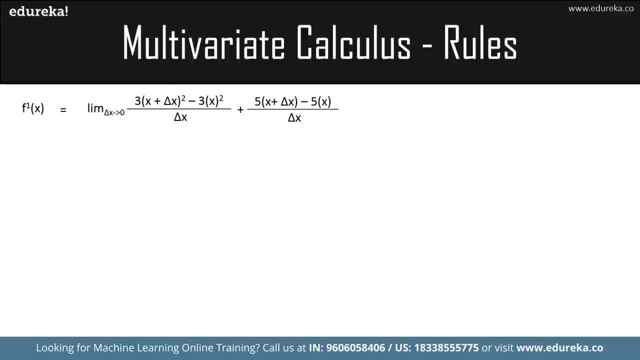 example will be 3x square Plus 5x. Okay, so I'm going to solve the equation right now. 3x square, I hope you remember. I just showed it to you before. and the same thing goes for 5x also. 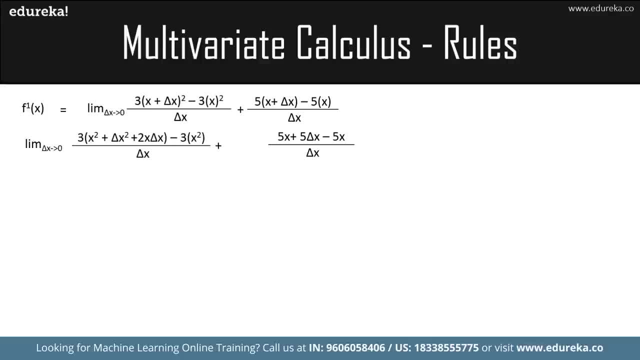 So so, 5x plus 5, Delta x minus 5, and then I'm going to just, you know, cancel out 5x is, and then I have Delta x being cancelled out, and then I have x squared minus x squared being cancelled out. 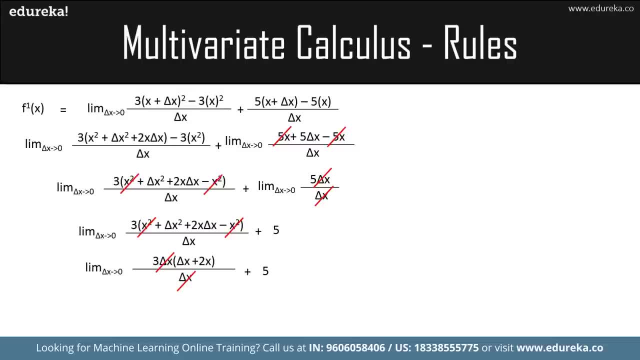 So the whole same process goes on. then Delta x gets cancelled, Then I have success with 5.. So I'm going to use The same rule that we learnt earlier- that was the power rule- and then I have 3 into 2x plus 5, so I get 6x plus 5.. 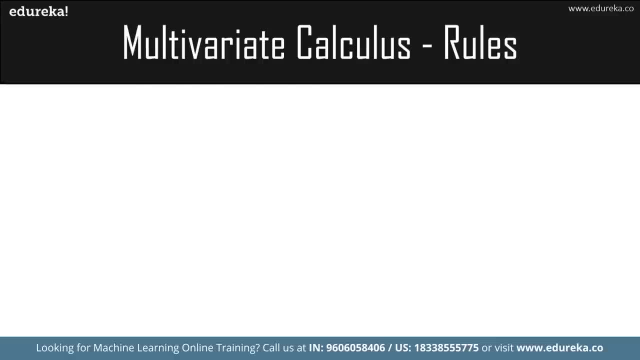 This is basically how the sum rule works. next, I have something called as the product rule tool. So if I have a function which is in the form of x into 2x or something like that, the differentiation is a very simple. This is how the differentiation looks. if it is f dash of x1 into x2, that 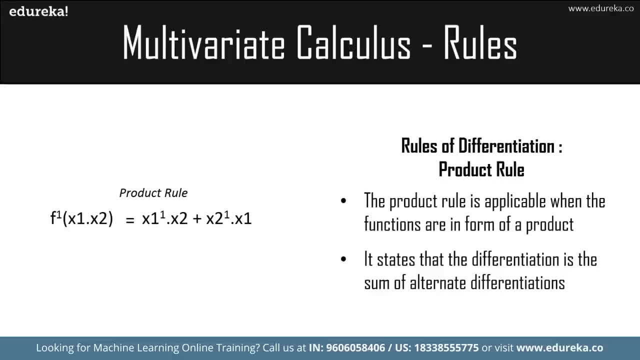 is equal to x1.. Dash into x2 plus x2 dash into x1.. That is how you're going to find out the differentiation. and the next rule that we are going to look at is the chain rule. So, basically, if I have f dash of g, dash of x, it will be f dash of g. 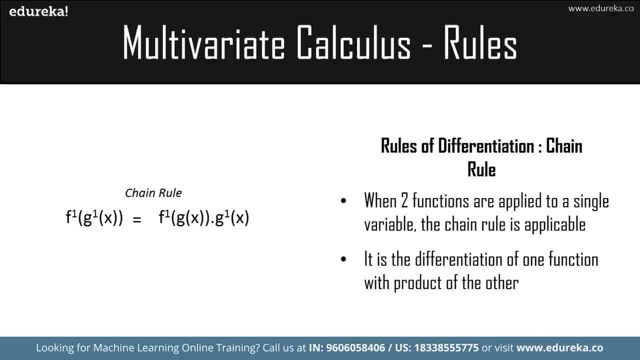 into x dot g, dash of x. This is a very simple example and it's really easy to understand. So if you want to learn more about the common functions, I have my blog, which is also put up in the description, and you can go ahead. 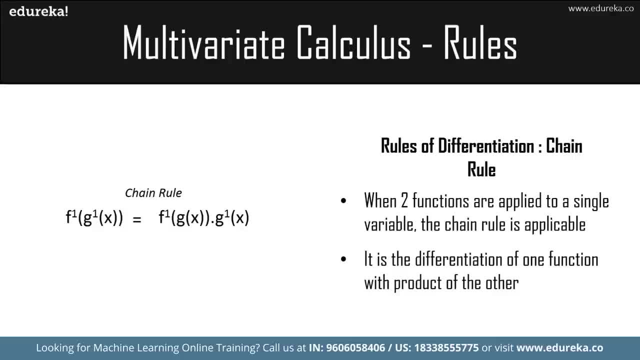 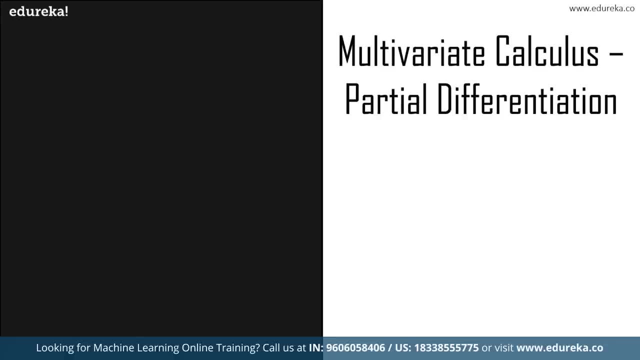 Click over there and learn more about the common functions. Okay, So now that we have understood all the basics that we really needed from differentiation, we'll now be moving over to partial differentiation. Partial differentiation is an important concept that most of us have ignored throughout our Academy. 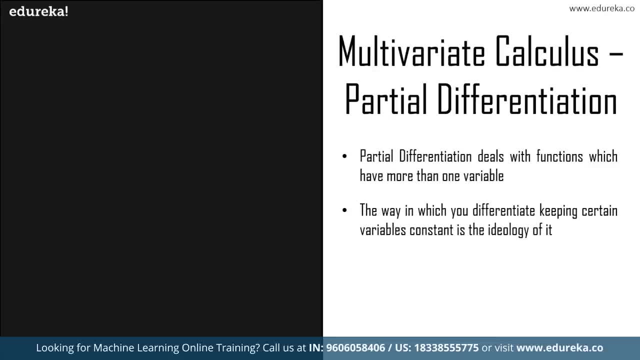 What has partial differentiation helped us achieve might be the question that most of you may be having right now. So let me give you an example so that you can understand its importance. Okay, Suppose you are A car designer who deals with the exterior of the car. only you have 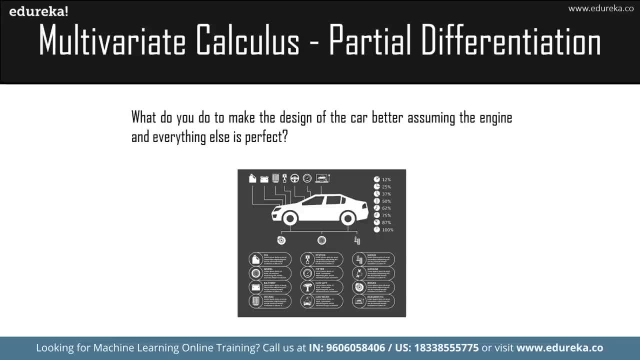 been given the task to maximize the performance of the car. So how do you do that? You do not go into the car, You do not take out the engine, You do not tune the engine. You are not supposed to do any of that. 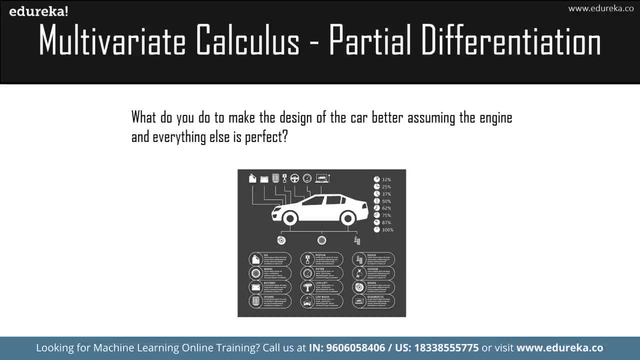 You just are going to change the particular exterior of the car. So what's happening over here? You know that even the engine and all the other tires and all that, all those are variables also that you know come to making the car better in its performance. but you are not going to do that. 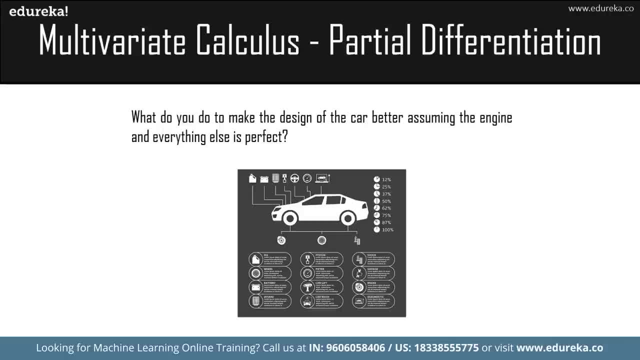 You're not supposed to do that, because you are only going to deal with the exterior of the car. those variables of the engine and all of that. Those are kept constant. If those are kept constant, that means that those variables will be performed by somebody else. 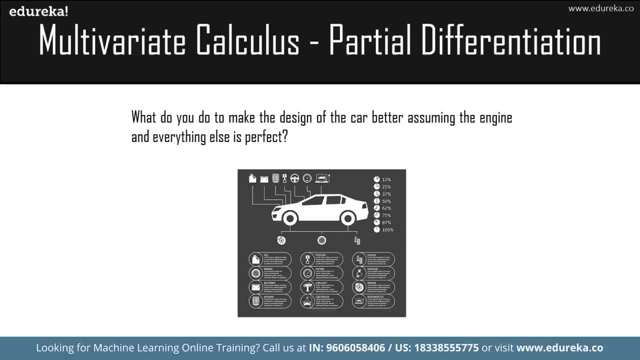 You are just going to look at your particular variable that you have to change, that is, the exterior of the car. So this is how partial differentiation comes into play. You are just going to change one particular variable. all the other variables become a constant. Okay, it's that simple. 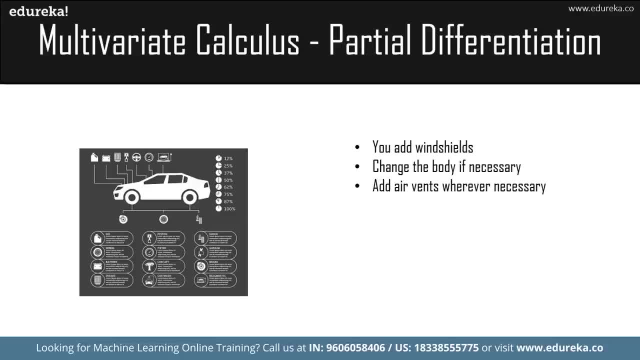 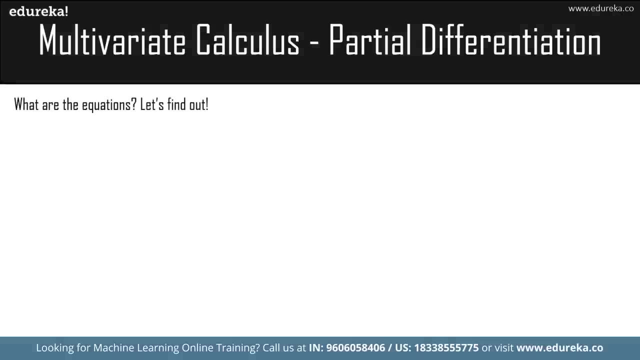 So what do you do? you would change the windshields, change the body if necessary, air vents and many, many more. I've just given whatever I could find. you are just changing What is necessary. that is basically what is partial differentiation. So what are the equations that partial differentiation goes according? 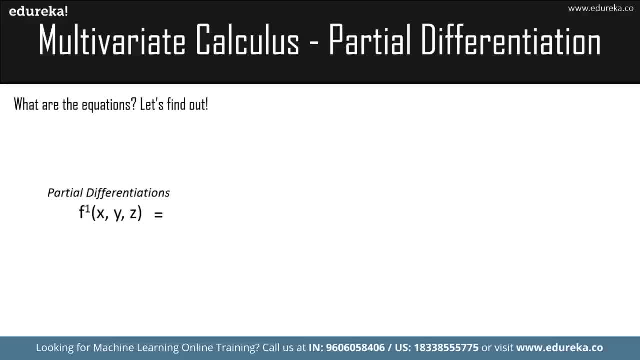 with now, If you can see, It is the F dash of X, Y and Z. If you remember the previous slides, we were just working on one variable, that is, X, which is X, 1, X, 2, which may be x squared, 3x, 5x. 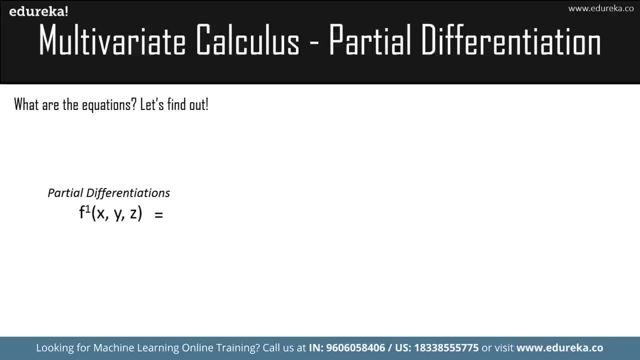 It was all all on X. partial differentiation is not like that. It is X, Y, Z, whatever variables it can find. So that is what makes partial differentiation much more realistic, much more easier to understand, because you are just going to change your factors, your variables. 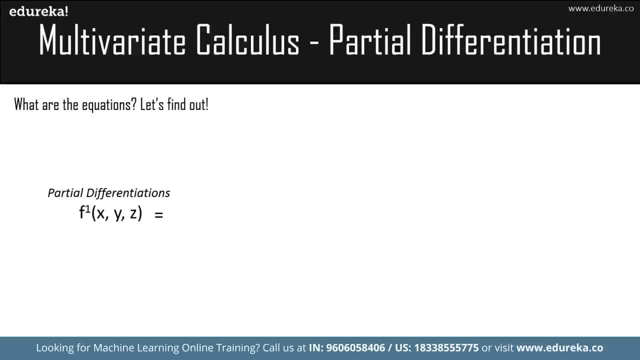 You're going to keep everything else constant. So let's say, for example, you have to find it with respect to Y, So Y and Z become a constant F dash of X. if you want to find it with respect to Y, X and Z become a constant F dash of Y. with respect to Z, X and Y. 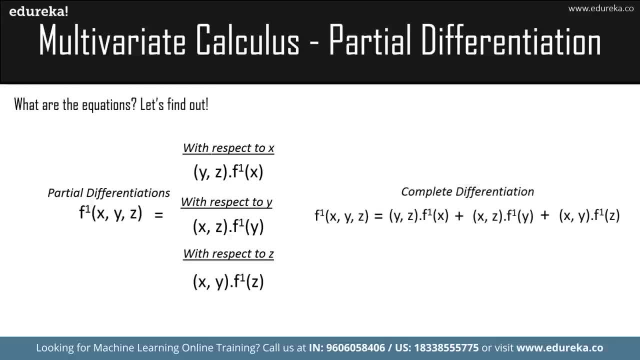 become a constant F dash of Z. So what is the complete differentiation? It is the addition of all the three differentiation that we've just found out. So this is how partial differentiation works. Let's show you an example. So if I have a function which is x square plus 3y plus 4x Z square, 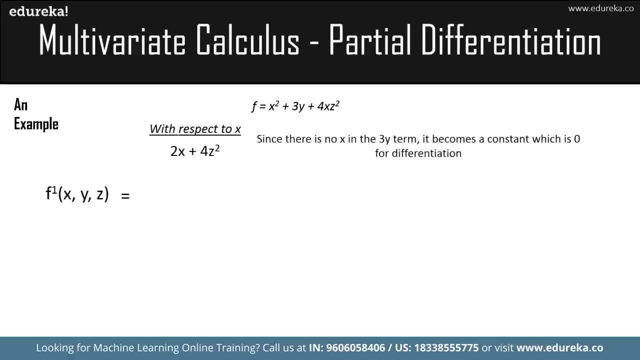 how am I going to find the differentiation of this? So, with respect to X, Y becomes a constant, So it is 0. and then you have a 2x plus 4 Z square. So with respect to Y, x square plus 4x, Z square become a constant. 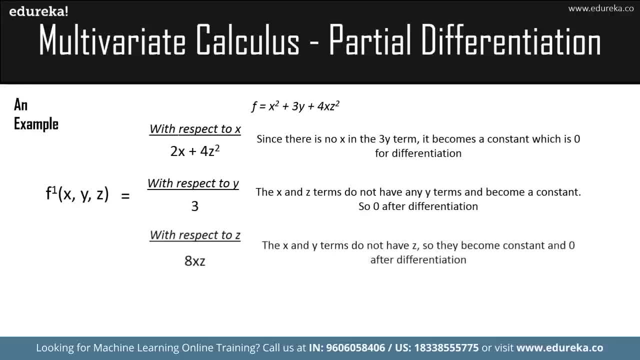 So I'll just have three. so with respect to Z, it will become x square, becomes a constant, 3y becomes a constant, and then 4x Z square is what I am going to differentiate. So I will have 8x Z. So what is the total differentiation? 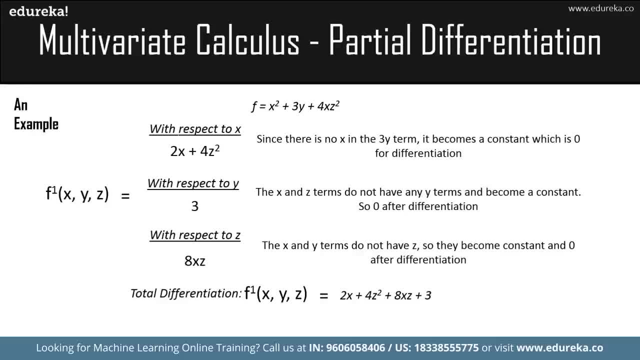 It is a 2x plus 4 Z square plus 8x Z plus 3.. So I hope you've understood this really simple example of it. So this is how partial differentiation works. So what are the applications that multivariate calculus comes into? 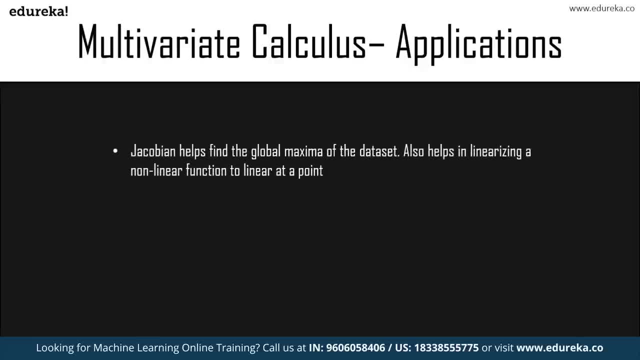 play. We have something called as the Jacobian vector. Now, what is the Jacobian vector? It is basically differentiating The vector once. Jacobian is basically differentiating the vector once and then putting it into the form of a matrix that becomes. 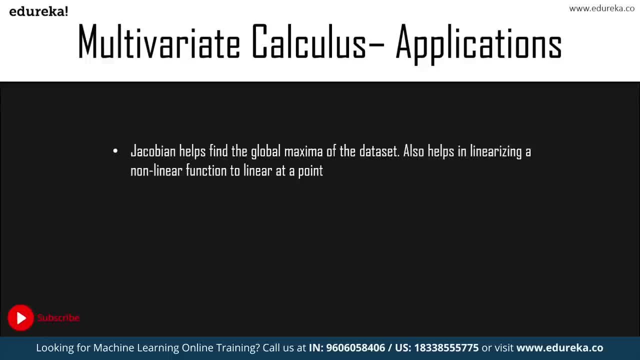 the Jacobian vector. It helps in finding the global maximum of the data set aside. It is pointing to the maximum data that is there in the data set and it also helps in linearizing a long linear function to a linear at a particular point. 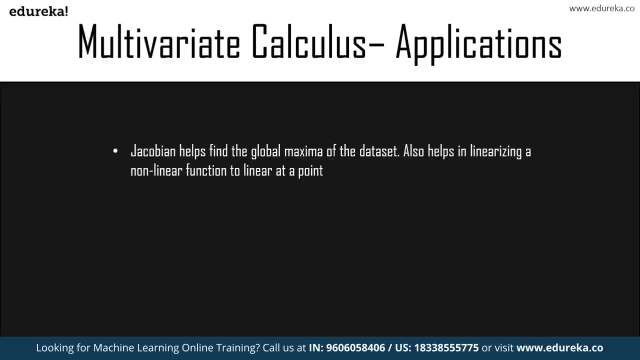 So that's how the Jacobian helps. So differentiating the Jacobian or differentiating the actual vector twice gives us the Hessian and it is used in minimizing the errors. It is used in deep learning models, gradient descent, for optimizing all the weights and all of that. 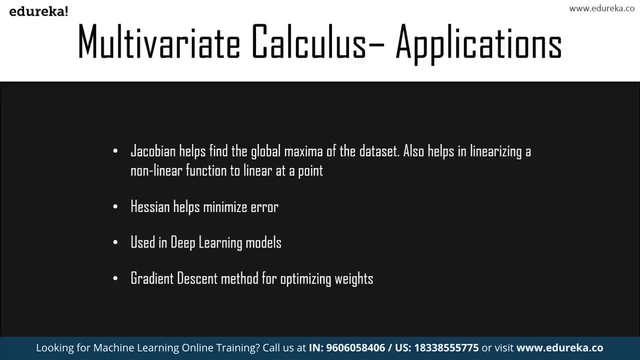 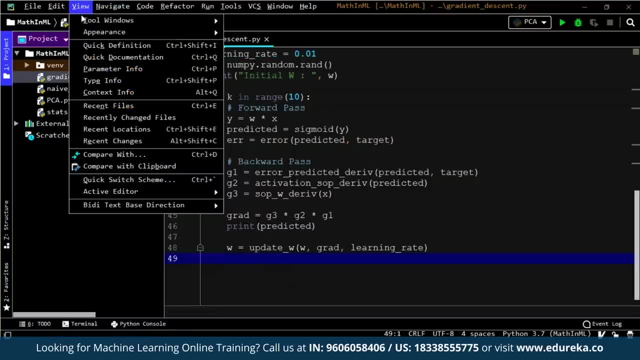 So that is how multivariate calculus helps us in real life. Let me show you how the gradient descent works. I already have code ready for you guys. Let me go back to the presentation mode. I have a particular import, which is the numpy, and then I have 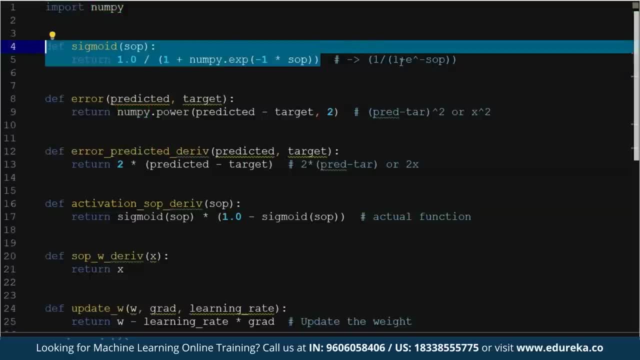 the sigmoid function, which is basically one Divided by 1 minus e to the power of minus SOP. So this is what I am going to return back to it. And then I have the arrow, that is, a predicted minus target whole square, or X to the power of 2.. 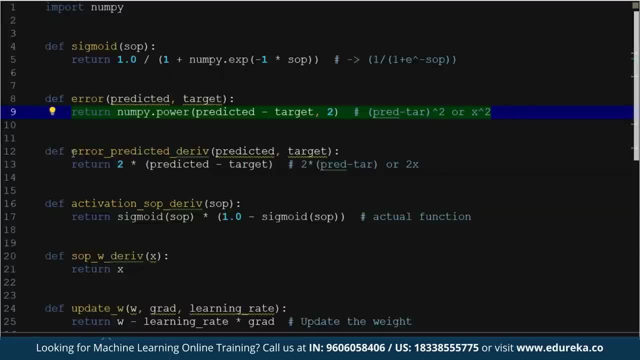 This is what the error is basically, and then I have the errors at derivation which I'm going to use over here. So that is basically 2x or 2 into predicted minus the target part, and then I have the actual function over here, which is sigmoid. 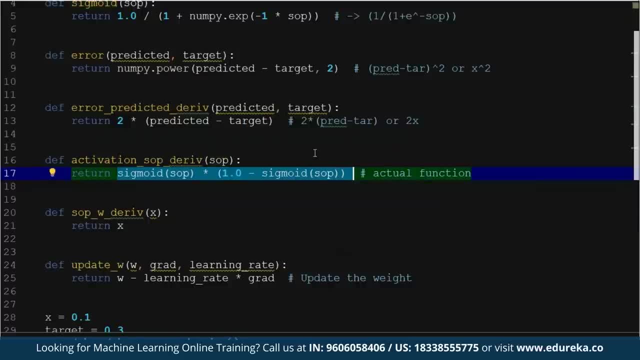 into 1 minus sigmoid, Which is the activation function, which is basically trying to find if my particular model is working or not, And then I have the derivation of it, which is just basically X, and then I have the updating function of the weight. 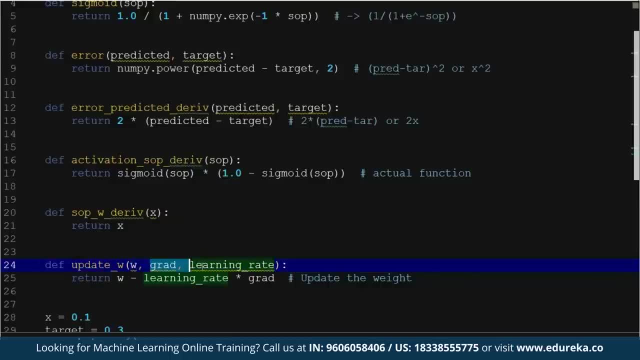 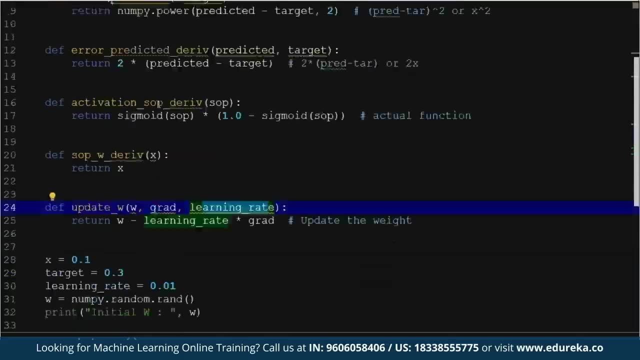 So I'm just going to get the weight, I'm going to get the gradient and I'm going to get learning rate and I'm going to basically keep trying to, you know, find out the best way that I can find my weight. So here's my function. 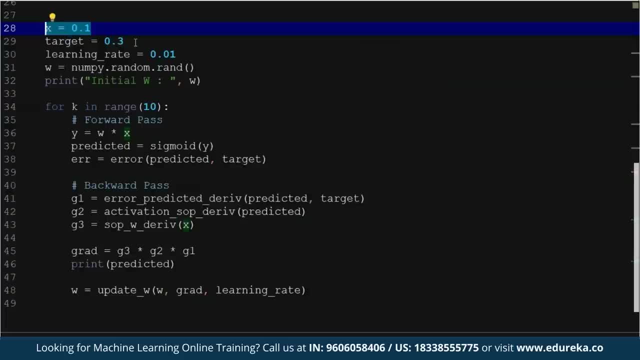 I have X is equal to 0.1.. Which is my input, and then I have the target, which is 0.3, and I'm going to have a learning rate of 0.01, and then I'm going to get a random number. 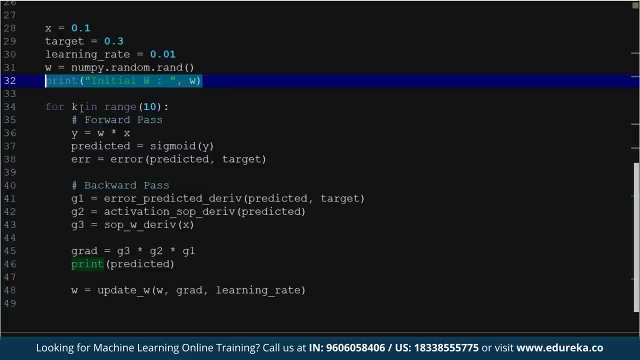 which is the weight of it, And then this is the initial weight. What I'm going to do, then, is I'm going to find the value of Y and X, and I'm going to find the errors also, and then I'm going to find all the gradients. 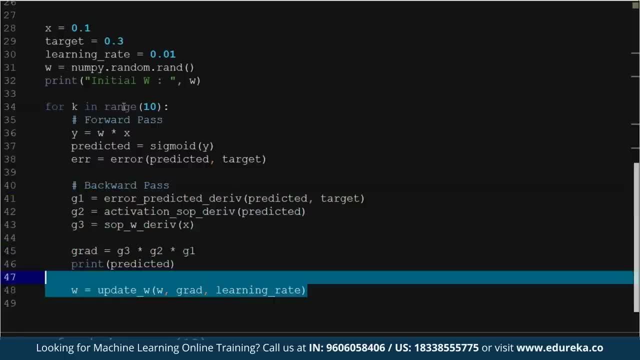 and then I'm going to pass the gradient into it and then update the weight. Let me show you an example now How increasing the number of steps is going to make me reach my Target much more better. So, as you can see, my initial weight was a 0.50 thing. 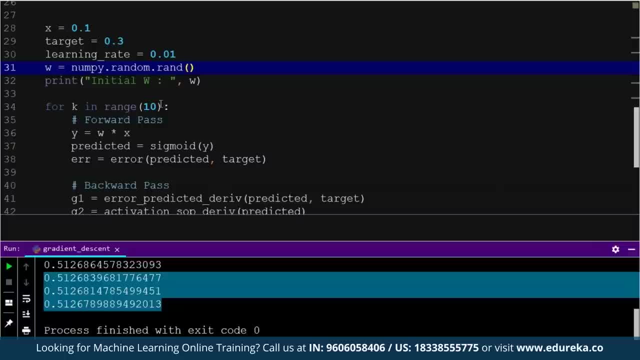 and all that, and I have just run this for 10 times. right, Let me change this to thousand. My input is 0.1 and this is 0.3.. I have to make 0.1 as 0.3, right. 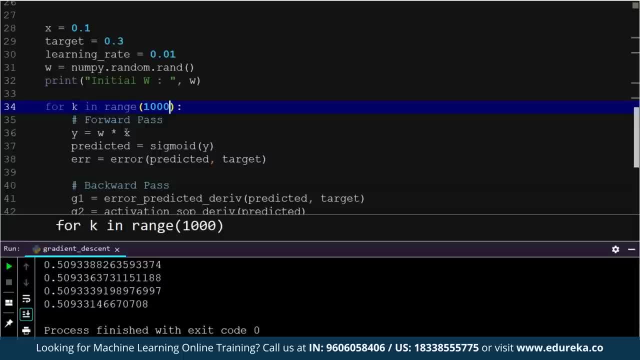 So let me run this again. It is still at 0.50.. Let me add another 0, which is 10,000 times. Let me run this So, as you can see, it has now become 0.47, which is much more better than what we were actually doing. 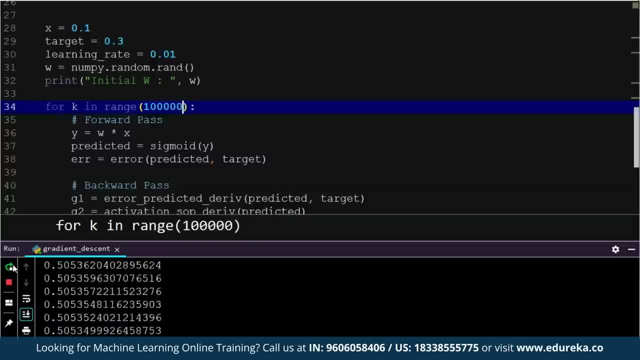 Let me add another 0 over here. So this is going to take a lot of time because the amount of you know steps to be performed a move. but as you can see over there, Which was 0.5 previously, has now come up to 0.36,. 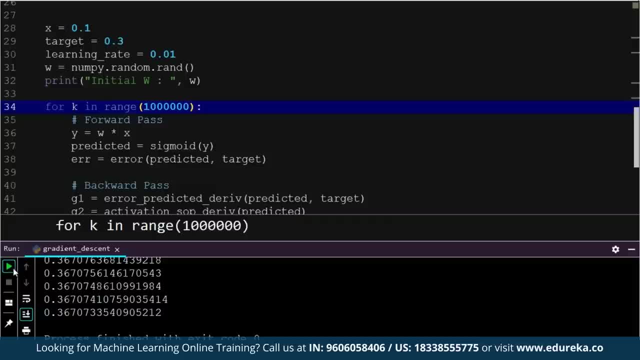 which is much, much better than what we were actually getting. Let me add another 0.. Let me run it again. You know, 4.6, 4.4, 4.0.. As you can see, it is reducing. It's just reducing the input. 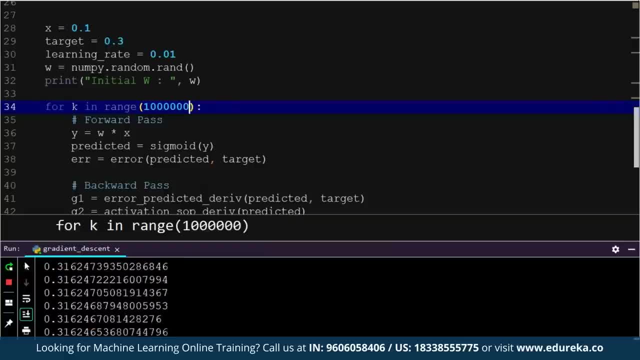 and our output is almost, almost close enough. What we really needed, the target, was 0.3 and, as you can see here we've already read 0.30 and all the numbers that are succeeding it right, If you remember, we had 10 steps. 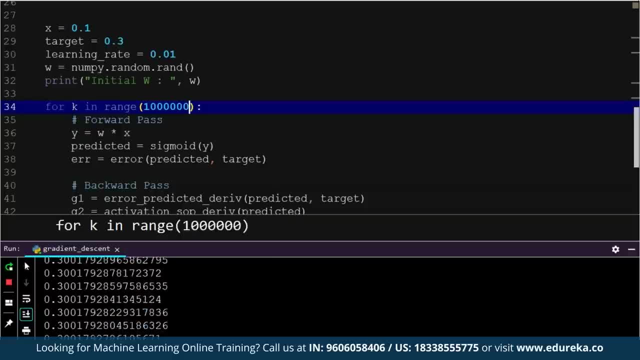 which would just give us 0.5, 0 or 5, 1 something. now, for the amount of times it has learned, it has become much, much, much better than what we have previously getting. So now it is 0.3, 0, 0, 0, 0, 2 something. it's still reducing. 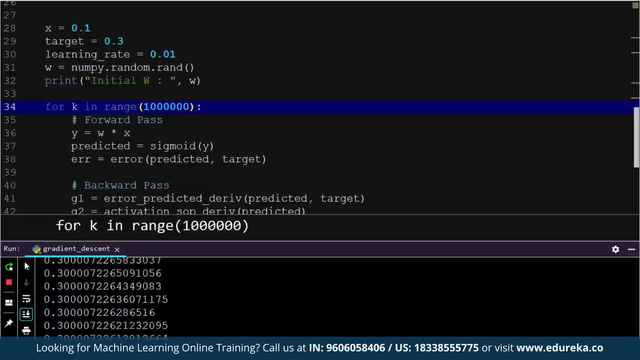 It is still reducing. So this is how the gradient design works: It keeps repeating, learning, learning. This is the final output that we've achieved: 0.3 0, 0, 0, 5, 7, 7, and it is much, much, much better. 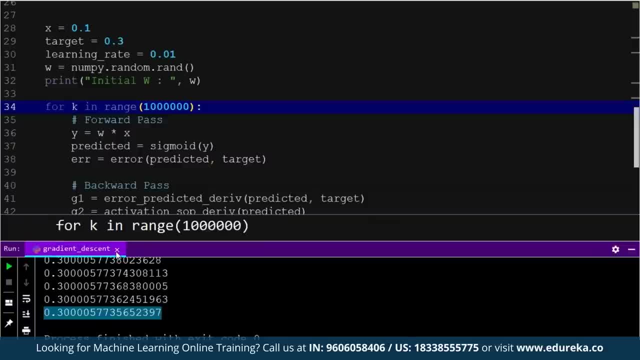 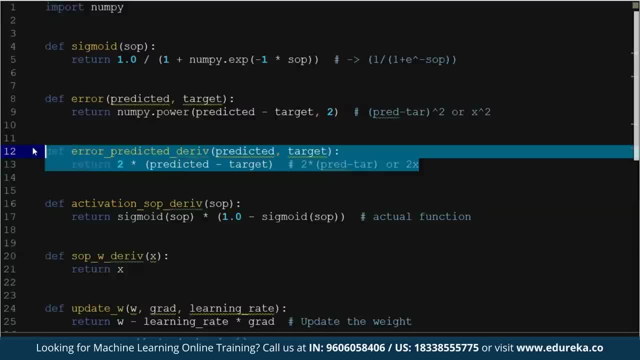 than what we were already getting from the output. So this is how the gradient descent works. It uses differentiation. Where is the derivation over here? This is my derivation function. This is my derivation function. So these derivation functions are what are helping me to get my new error. 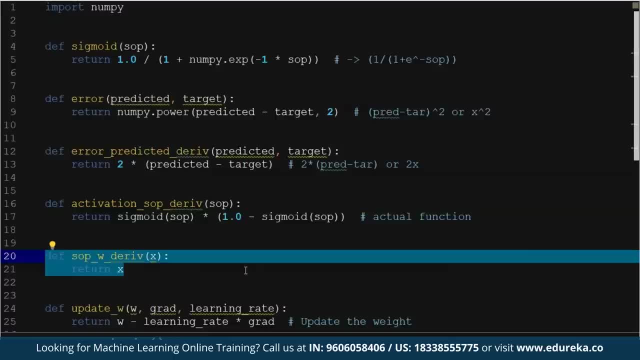 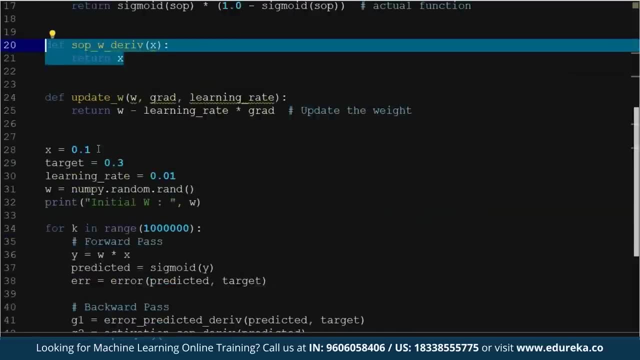 get my new error and then put that into the gradient descent function and then basically find and make my weight much more better so that I can get the output which is from my input, 0.1.. I have to get the target of 0.3. 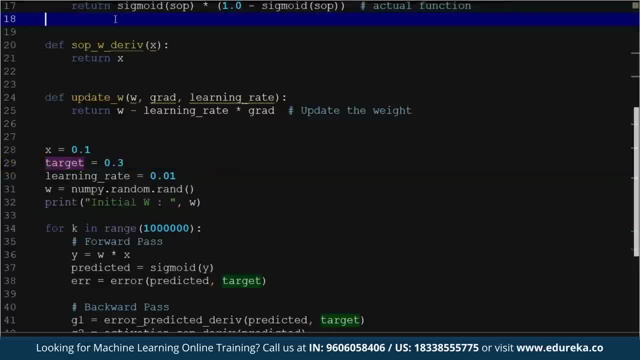 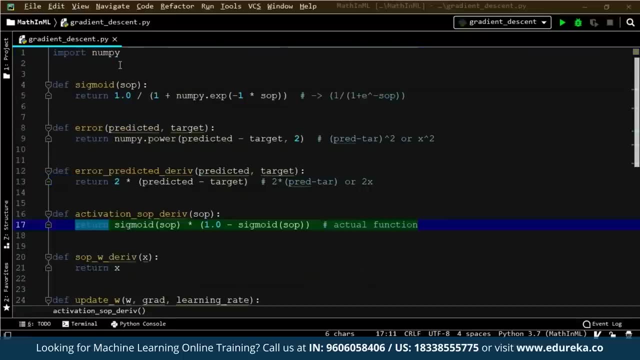 So I hope you've understood how the gradient descent works. It keeps going in and in and it uses a differentiation Lord. So I hope that was very easy for you guys to understand. So with that we have come to the end of all that was required. 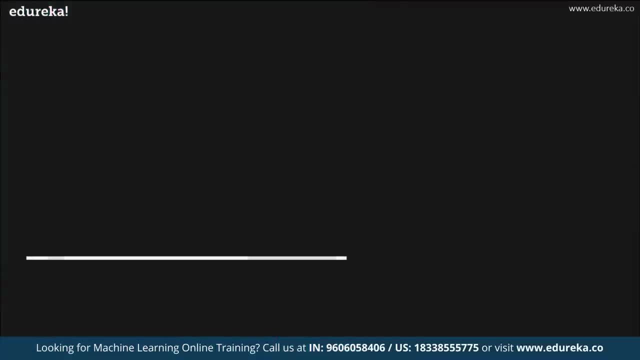 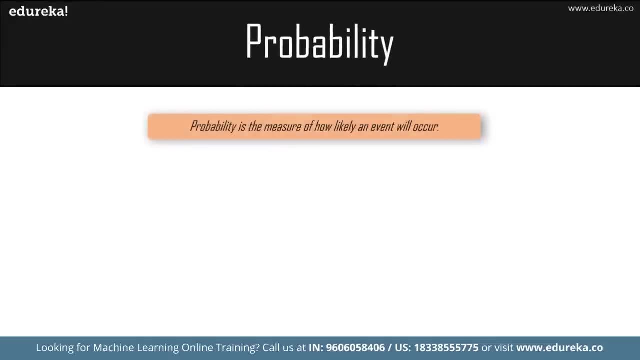 from multivariate calculus. Let's move over to the next topic, which is a probability. So what is a probability? probability is measuring how likely an event will occur. what this means is that how much are you sure, or how much quantity that you can give to your sureness. 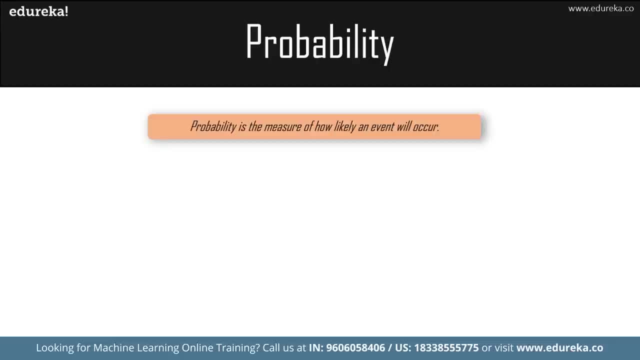 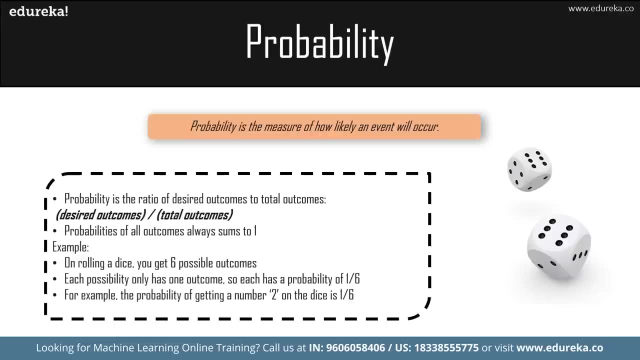 that this particular event is going to happen. So that is what is probability. It is the ratio of the desired outcomes by the total outcomes, right? So with that particular formula, you will be able to understand what is the probability. It is the desired outcomes by the total outcomes. 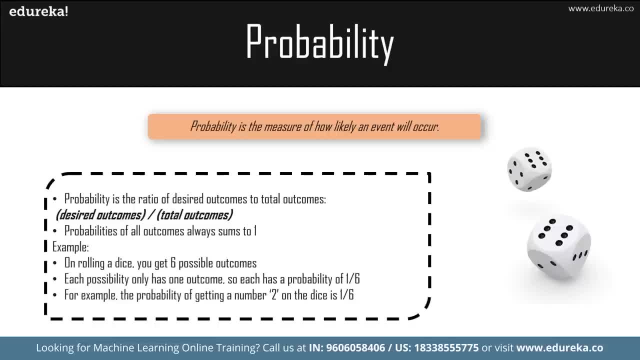 So always remember that probability is always come up to 1.. So if you have 0.6, that means you have a 60% probability that this particular thing will happen. If you have 0.6 of something happening and 0.4 of something not happening, 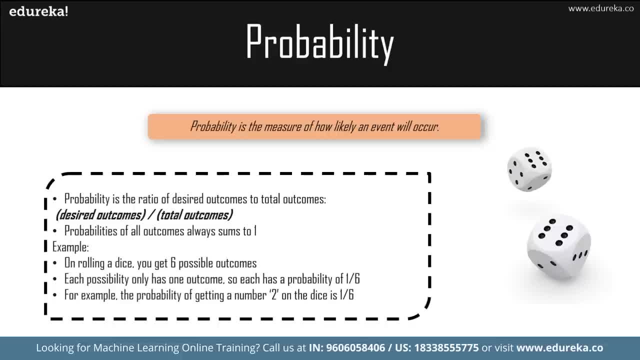 they always sum up to 1.. Remember, probability is always sum up to 1.. So some examples that I've given over here are rolling a dice. There are six possibilities, right? So every possibility, He has one outcome out of the six outcomes. 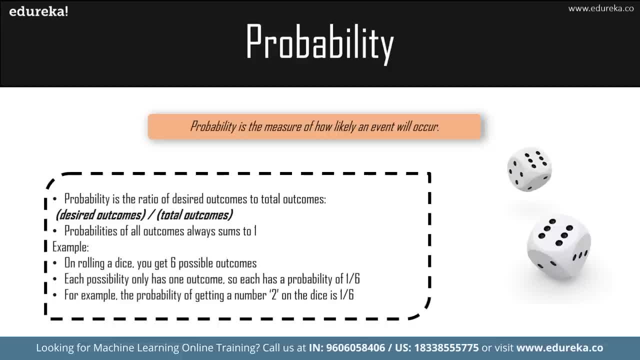 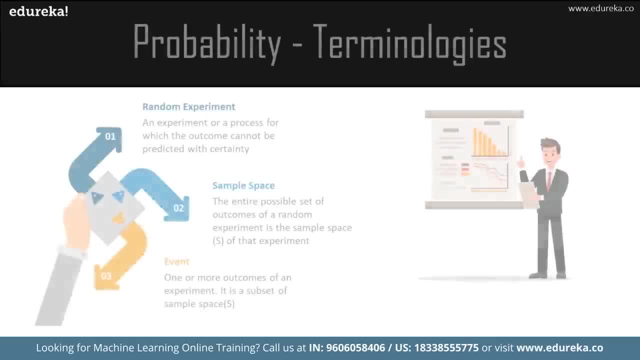 So, for example, the probability of getting a number two is 1 by 6.. So that is the probability of getting a number 2 by 2.. This is basically what is probability. So what are the terminologies that you need to understand when it comes? 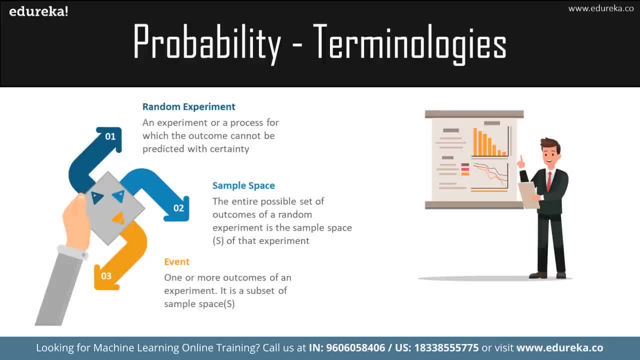 to probability. There are three things. Okay, you need to understand what is a random experiment, What is a sample space and what are the events. Let's understand all of these terminologies one by one now. So what is a random Experiment? 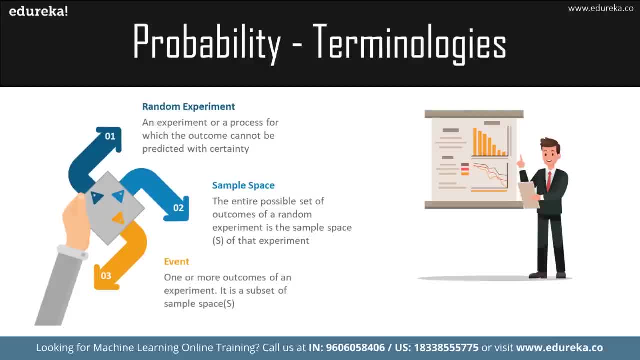 It is an experiment or a process for which the outcome cannot be predicted with certainty. So, for example, if I give you a dice, okay, and I tell you to roll it and tell me the number that you're going to get it- You are not sure because that's a random experiment. 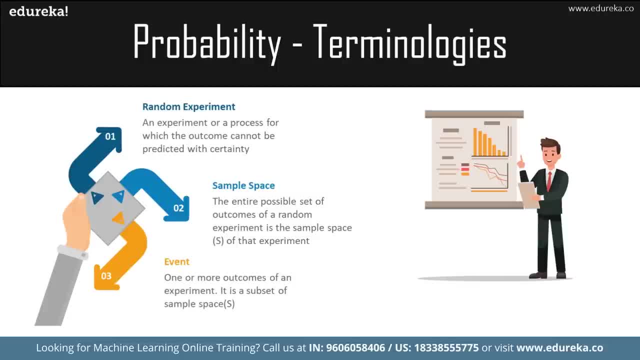 You have this uncertainty whether this particular event will happen or not. Okay, so that process where you roll a dice and all of that, that is a random experiment. So what is the sample space? the entire possible set of outcomes of a random experiment is the sample space of that experiment. 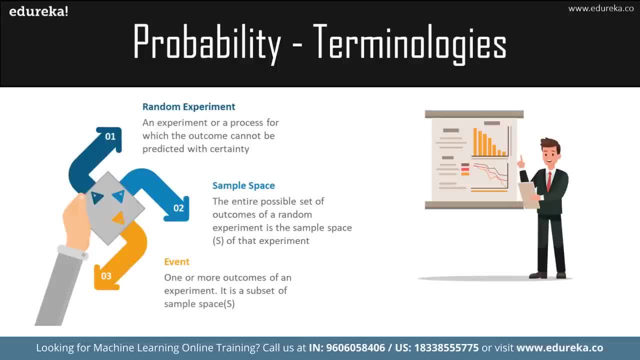 It's really simple, right? I tell you to roll a dice. There are six outcomes, So it can be the 1, 2, 3, 4, 5, 6, that particular range of 1, 2, 3, 4, 5, 6. 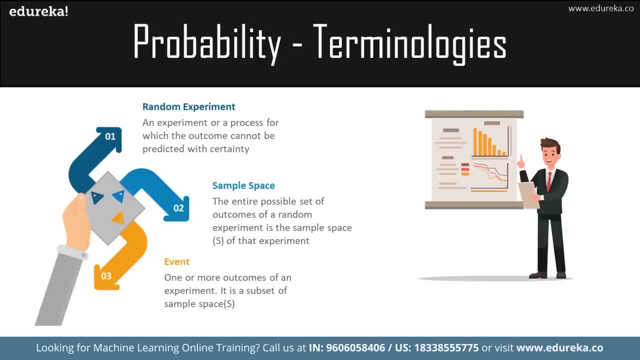 is the sample space. It is all the possible outcomes for the random experiment that you've been doing. simple enough. So what is an event? and event is one or more outcomes of the experiment. So if I told you, roll the dice, you get a number one, that is an. 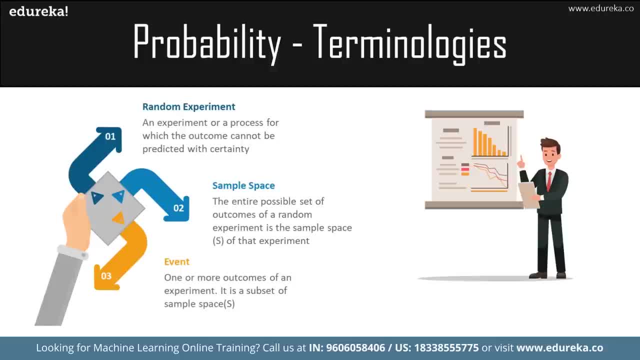 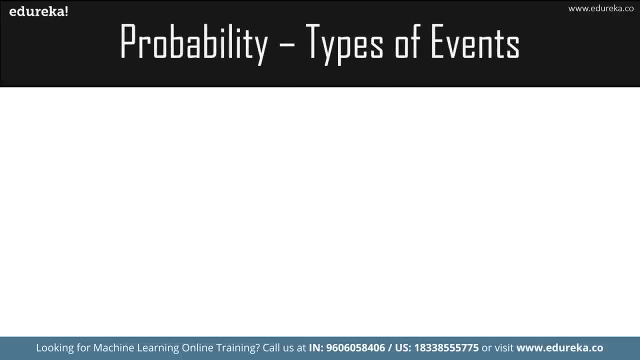 event. you roll the dice again. You get a number 6. that is an event. So what outcome you get from your random experiment is called the event. There are two types of events. There are joint events and disjoint events. Let's understand both of these. 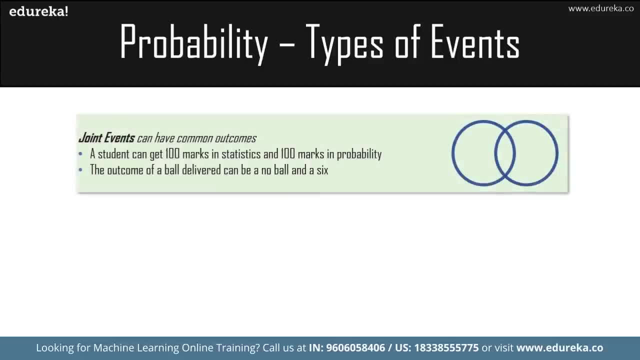 So joint events have common outcomes. right, joint events can be together. That is what is a joint event. For example, you have a student who can get hundred marks in statistics and hundred months in probability outcome of a ball that can be delivered can be a new ball also, and it can be a six also. and 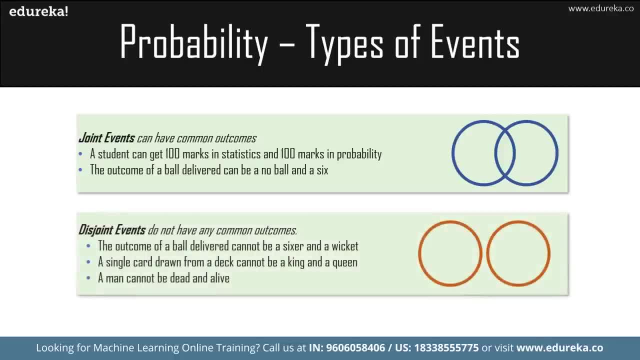 it can be possible are called joint events. disjoint events do not have common outcomes, So the outcome of a ball that is to be delivered cannot be a six and a hit wicket or something like that. Okay, so a single card cannot have be a king and a queen together. 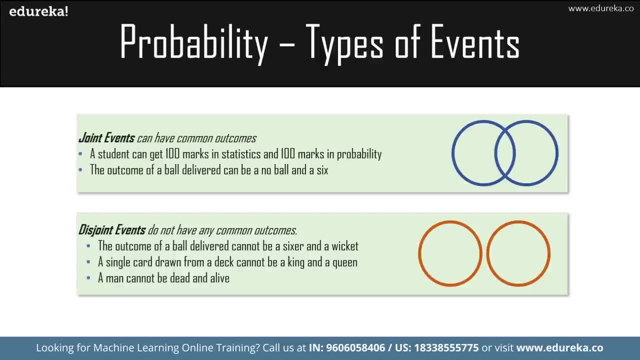 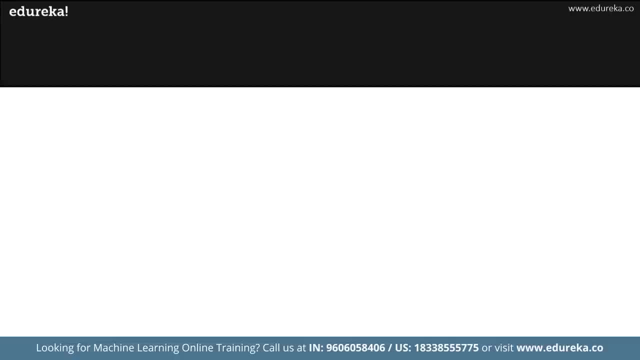 and a man cannot be alive and dead at the same time. So those are disjoint events. Those are not at all possible to happen. now that we've understood all the types of Events, we need to understand the distributions. So now we have a three distributions that come under probability. 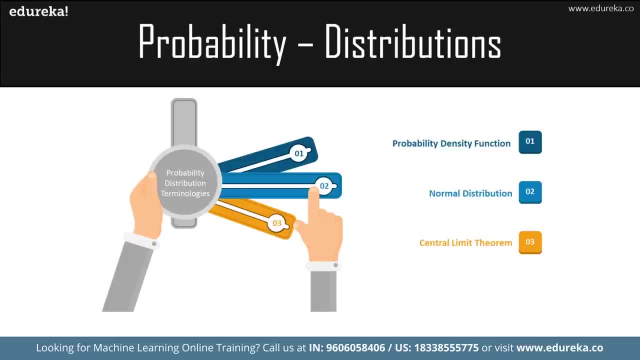 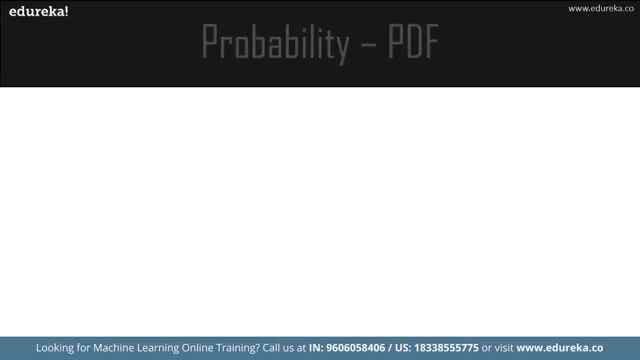 We have the probability density function, We have the normal distribution and central limit theorem. So let's understand all of these distributions one by one. So the first one is PDF: probability distribution function. So the probability now can be described using an equation, the equation that describes a continuous probability distribution. 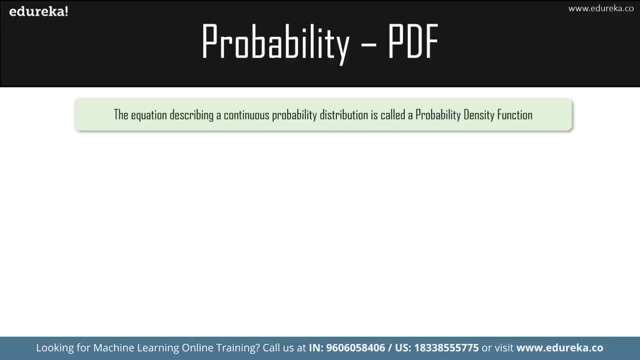 is called the probability Density function. I hope it's very clear to you. If it is not, let me just simplify it even more. you have a function which is going to describe the probability of something happening in the form of a graph. It's that simple enough to understand. you have a function which 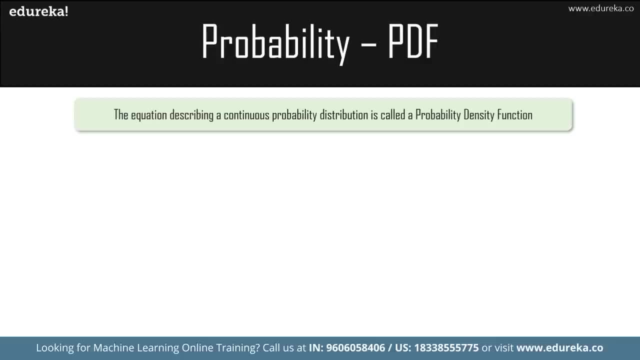 will give you the probability which you can plot a graph on on. so that is the reason it is a continuous probability distribution. Okay, as you can see, here you have a and B. between the range of A and B is the most likely that something is going to happen. 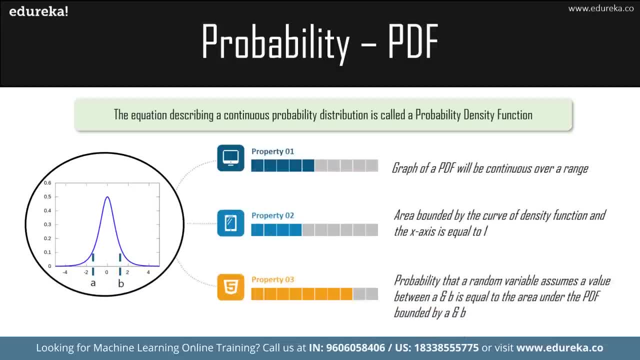 So now that you've understood what a PDF is, let's understand the properties of the PDF. the graph of the PDF will always be continuous. It's simple enough to understand that. then the area bounded by the curve of the density function and the x-axis is always going to be one. 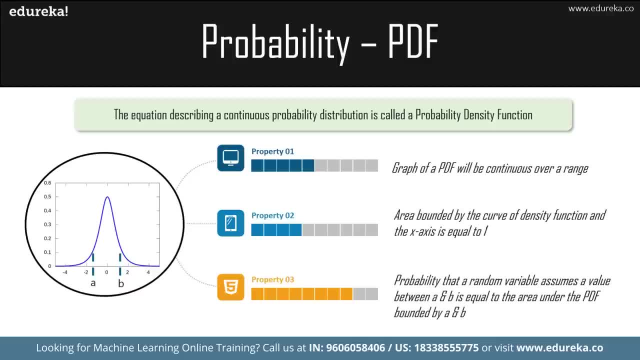 and the probability that a random variable assumes a value between A and B is equal to the area under the PDF bounded by A and B. what this means is basically: if you have any particular value or any particular probability That is between A and B, It is going to be equal to the area that is bounded by A and B. the 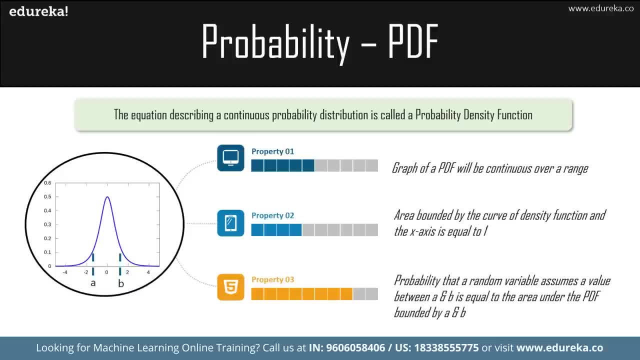 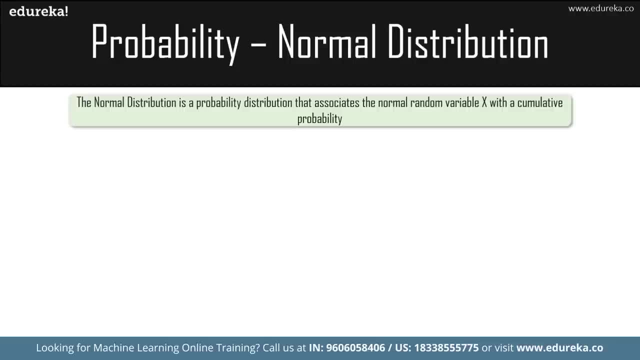 probability value. So that is basically what a probability density function is. So next we have the normal distribution. So what is a normal distribution? It is a probability distribution that associates the normal random variable X with a cumulative probability. So how do you find this particular cumulative probability? it is: 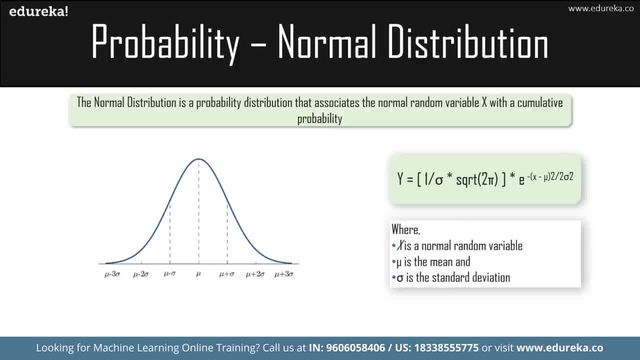 using this formula, which is: y is equal to 1 by 7.. Sigma into the square root of 2, pi into e, to the power of minus X, minus mu, into 2 divided by 2. Sigma 2 where X is the normal random. 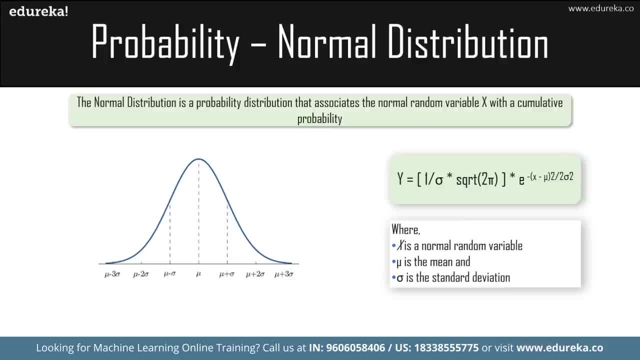 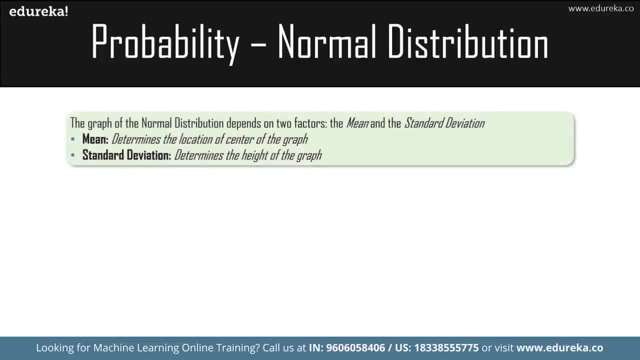 variable that we have just taken up, then mu is the mean and Sigma is the standard deviation, and this is how the normal distribution looks like. the graph of the normal distribution depends on basically two factors, which is the mean and the standard deviation. So the mean determines the location of the center of the graph and 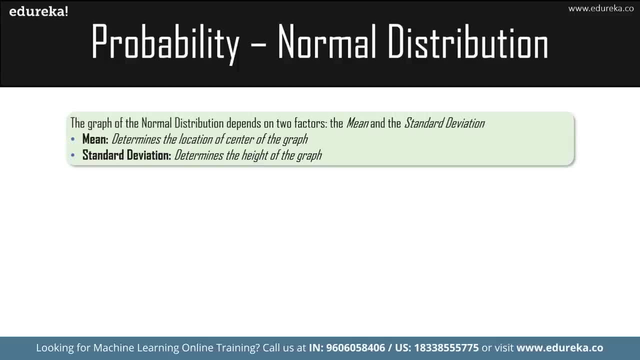 the standard deviation determines the height of the graph. So if you have a very big deviation between you know your variables, it becomes a very short graph and very wide graph, Whereas if you have a good deviation, which is you know very less, you will have a tall graph. 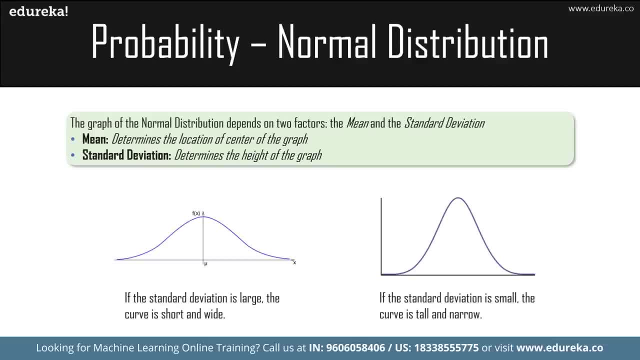 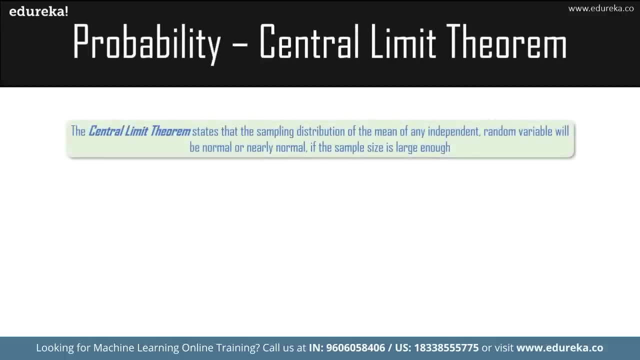 That is basically what's going to happen over here. That is all we have from normal distribution, then the central limit theorem. So this is basically a theorem which is stating that the probability is always going to be in the center of the graph. Let me tell you the statement of this: the central limit theorem. 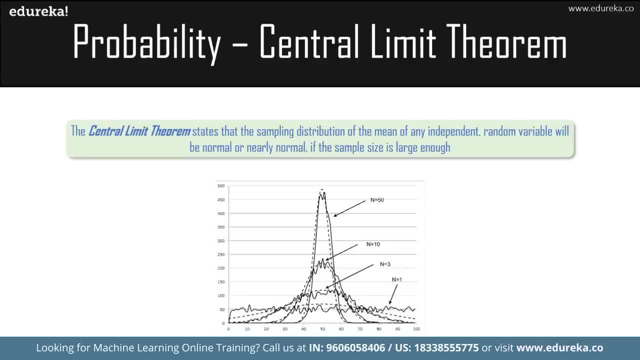 states that the sampling distribution of the mean of any independent random variable will be normal or nearly normal if the sample size is large enough. So what this basically means is that the distribution of your mean or your samples are always going to be near the center, or always. 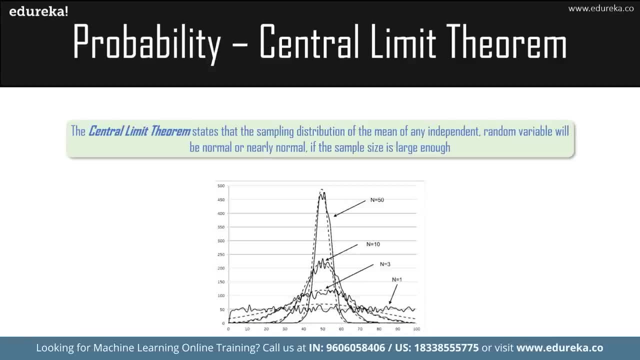 going to be near the mean of your graph if your sample size is much, much large enough enough. So what this means is that if your sample size is very, very big, it is going to be a normal distribution. It is as simple as that. 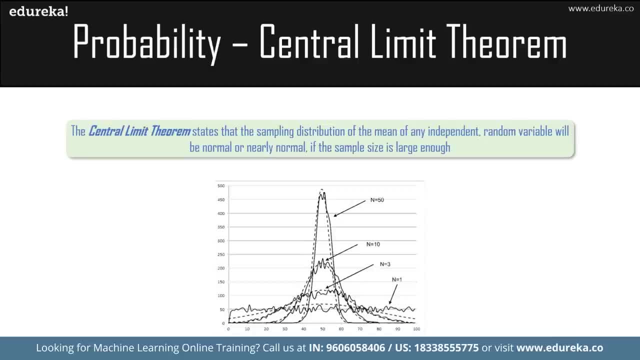 So, as you can see, if I have, n is equal to 1 component. you can see the graph as it increases to 3, as it increases to 10, as it increases to 50. So, as you can see, it almost becomes nearly identical to a normal. 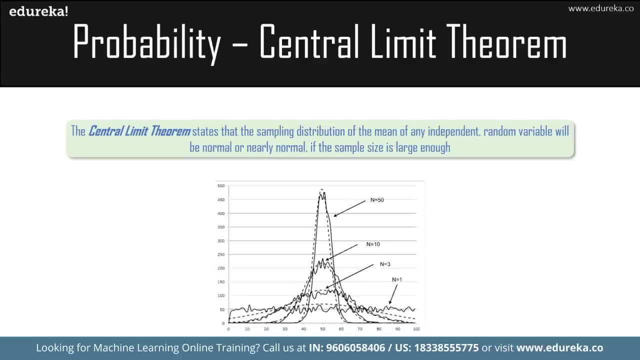 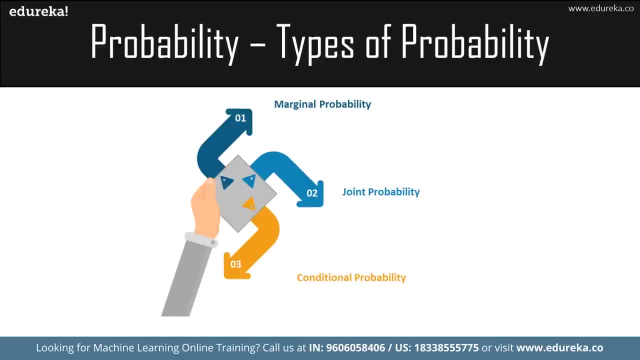 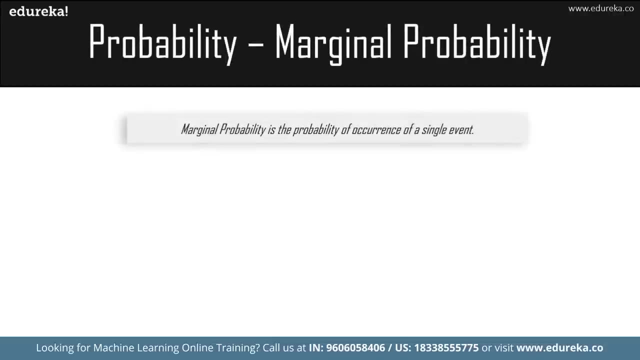 distribution. So that is what the central limit theorem is. So once we are done with that, we will look at the types of probability between. we have marginal probability, joint probability and conditional probability. Let's understand each of this. So what is marginal probability? marginal probability is the probability. 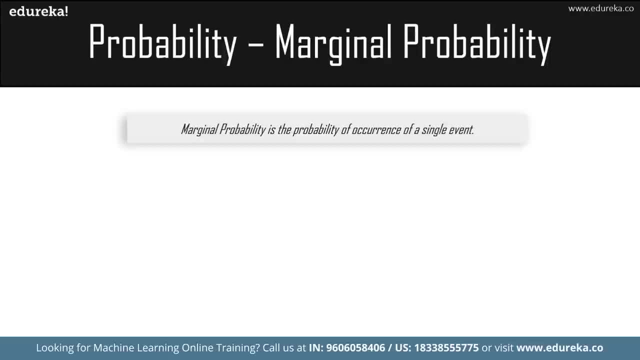 of occurrence of a single event. If I flip a coin it is going to be the head or a deal. that occurrence of that single event is called as a marginal probability. So, for example, I have a deck of cards here and I randomly take out. 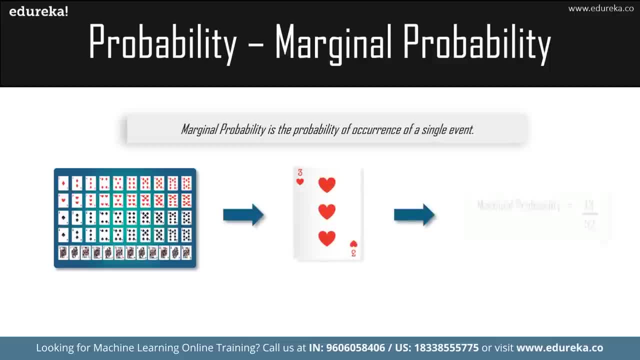 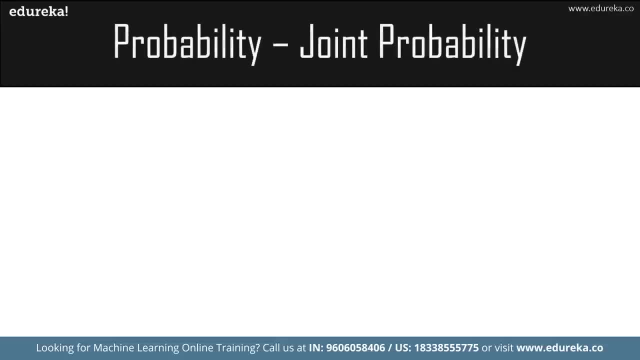 a card from there and I want it to be a hard card, right? So that will be the probability, which is 13 by 2, and it can be expressed by this particular formula. So once we are done with marginal probability, let's go to the next. 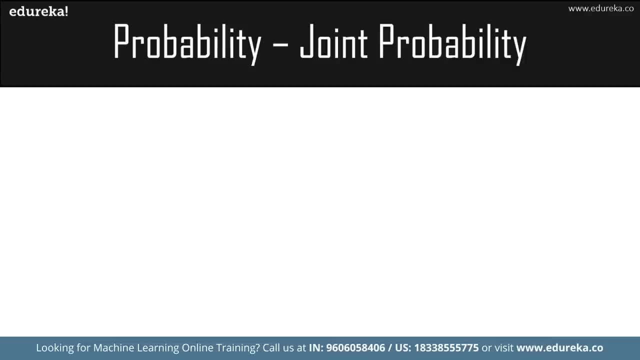 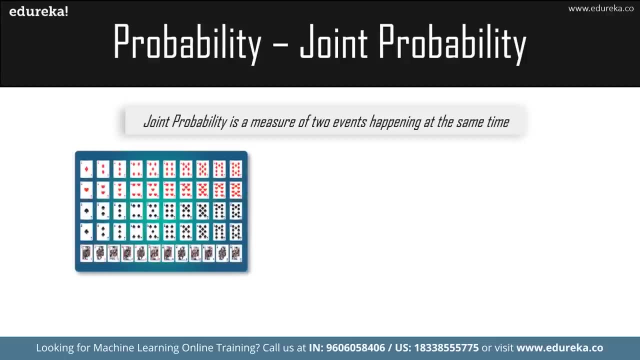 one. So once we are done with marginal probability, let's go to the next one: Join probability. What is joint probability? It is the measure of two events happening at the same time. So the same example. over here, I have a deck of cards out of which I want to take out the Ace, which 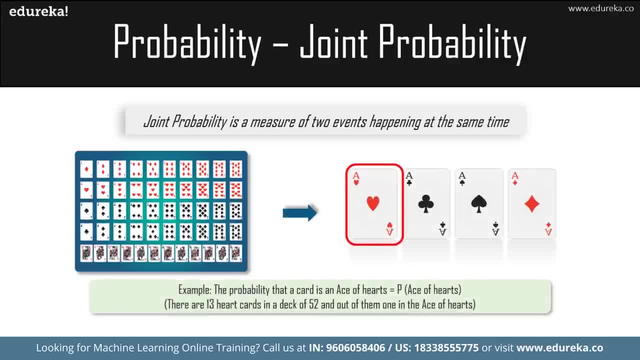 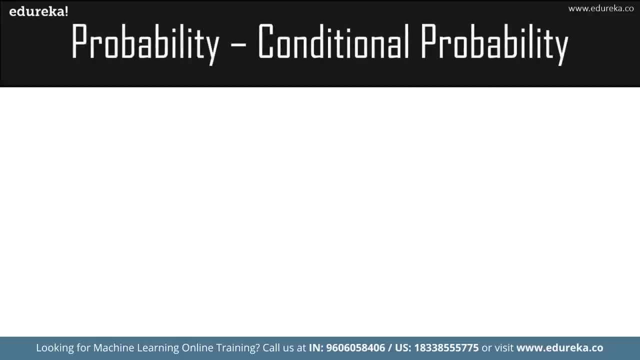 is a hearts, So it has to be a Ace card and it has to be a hard card, which will be the probability giving me 1 by 52.. So now that we've understood what is joint probability, let's understand what is conditional probability. 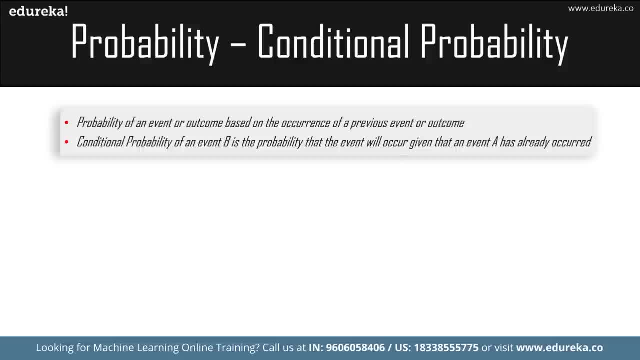 So the probability that depends on something already happened Is called as the conditional probability. It is basically the outcome of the event is based on the occurrence of a previous event or an outcome. conditional probability of an event. B is a probability that an event will occur. given that a event has 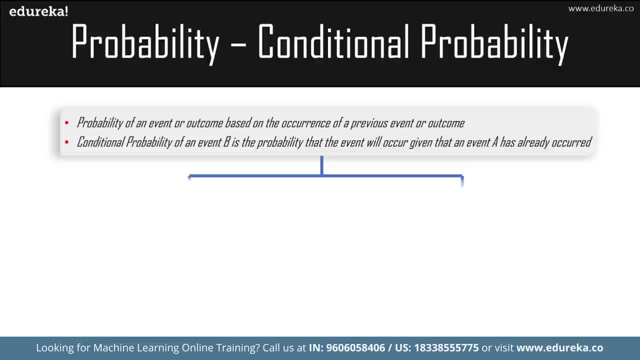 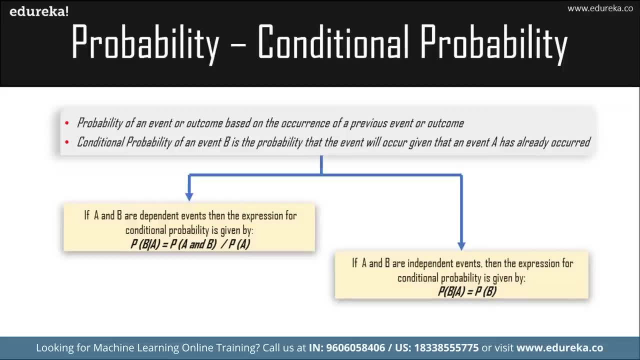 already occurred. What are the two types of formula that we have in conditional probability? if a and B are dependent events, then the expression for the conditional probability is given by P of B, by a is equal to P of a and B divided by P of a. if a and B are independent events, 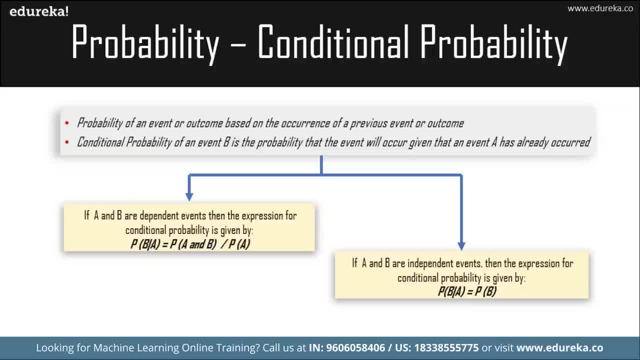 That means the expression will be P of B only, So it is just the probability of B occurring, Whereas if they are dependent events means that if you want to find the probability of B, a already has to be occurred. So it is a probability of a and B divided by the probability of a. so 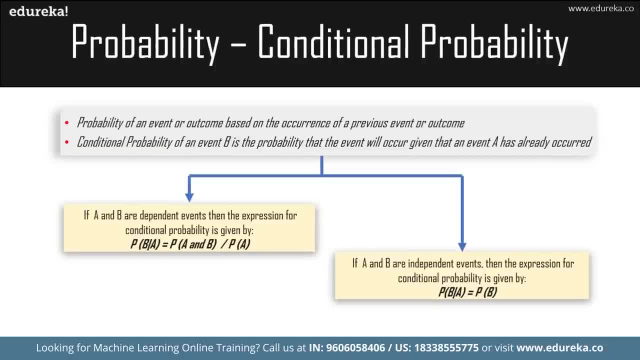 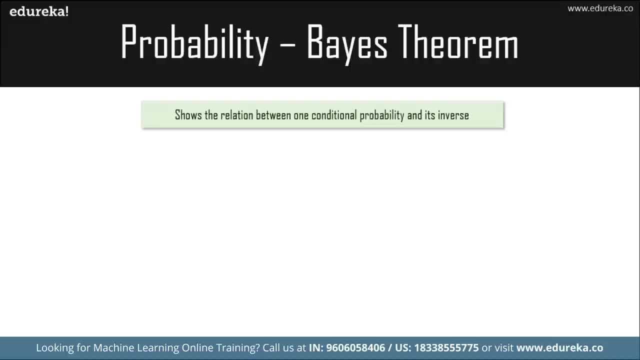 that is basically all the introduction that was required from probability. We now have base theorem. So what is base theorem? It shows the relationship of one conditional probability and its inverse. What is base theorem? It shows the relation between one conditional probability and its. 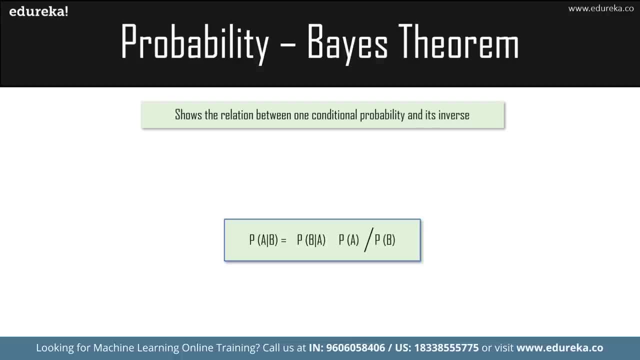 inverse. So this is the formula, that is, P of a by B is equal to P of B by a, into P of a divided by the P of B. So what does this particular thing mean? So what we are trying to find out is the probability of the occurrence. 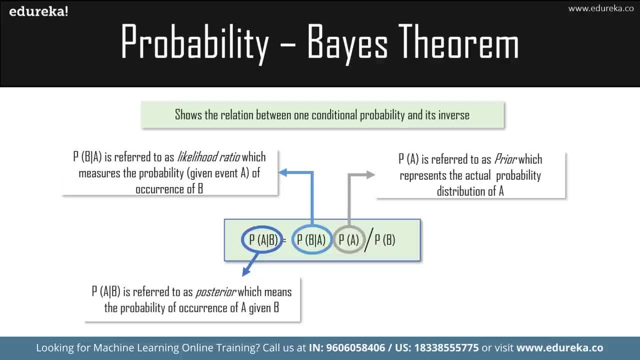 of a, given that B has already occurred, is equal to the probability of B occurring when a is already there, and the P of a, which is the prior probability, which is something We already think of, and then the probability of B occurring. So this is basically what the base theorem is. 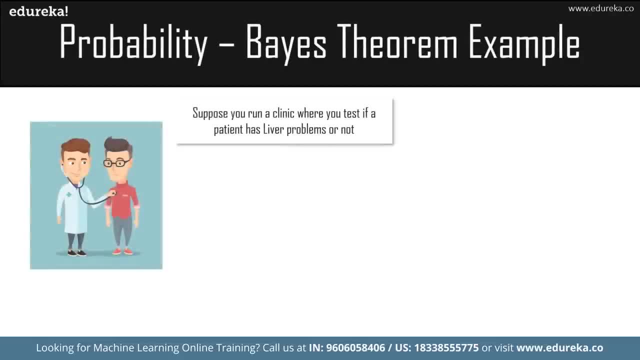 Let me give you an example for it. Okay, Suppose you are a doctor and you are running a clinic where you test if a patient has a liver problem or not. all the previous patient that had come to you- out of them, 10% of your patients- had liver problems. 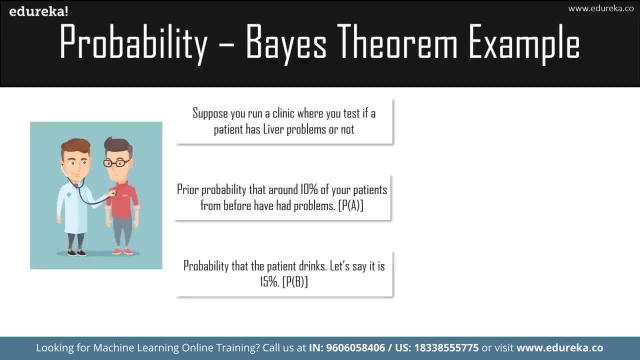 Okay, So all the patients that had come before they had around 15% probability that they would drinking. So now we have found out the probability of a and probability Of me, the prior probability and the probability of B. So what was the probability that out of all of those patients, even 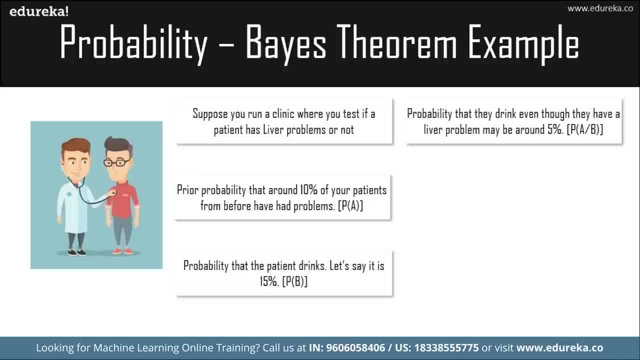 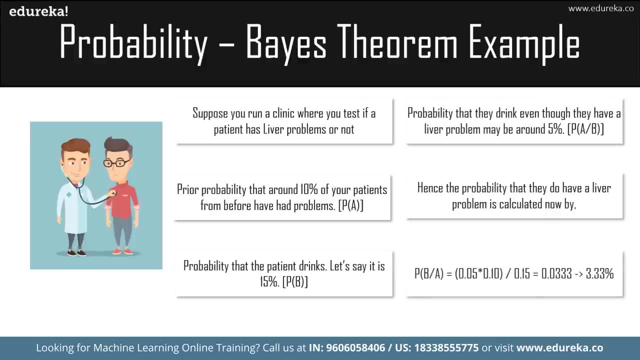 though they had a little problem: they were drinking. it is 5%, which is P of a by B. Hence the base theorem sees that the probability that a new patient, whoever's entering, will have a particular liver disease is calculated by 0.05 into 0.10. divided by 0.15 is equal to 3.33%. what this means? 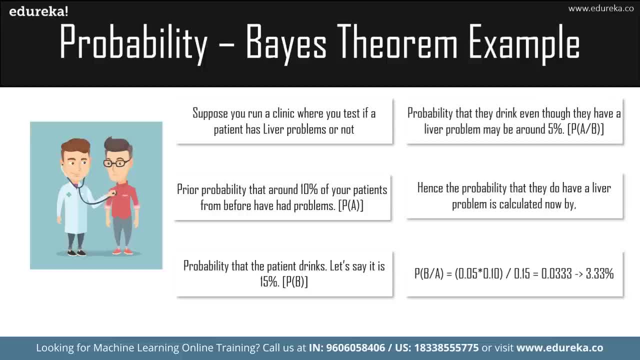 is that If a new patient is going into the clinic, there is a chance of 3.33% that that particular person is also having a liver problem. This is basically how the base theorem works. So what are the applications of probability? probability helps you to. 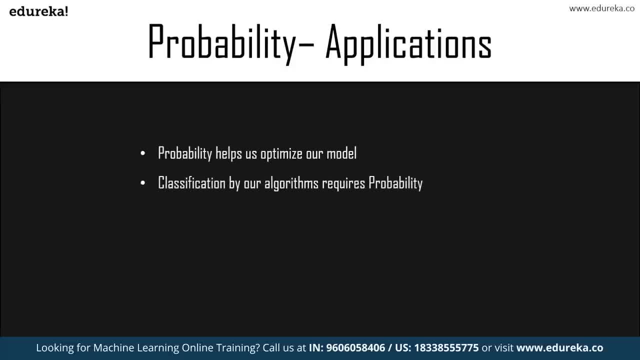 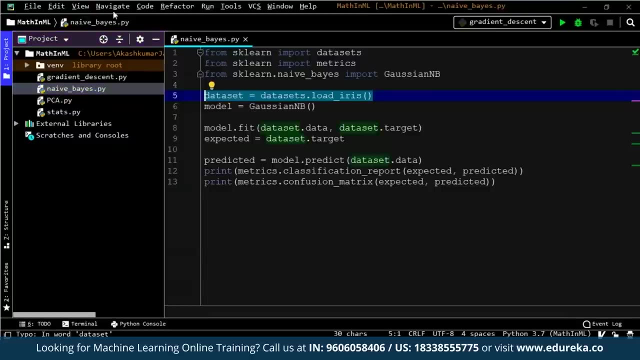 optimize your model. classification of our algorithms also requires probability. the loss can also be calculated using a probability. then models are built on probability. So let me show you how the knife based classifier works Over here. So let me go to knife base. This is the knife based classifier. 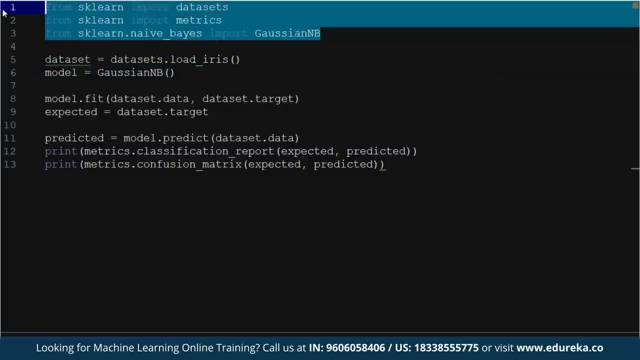 So let me tell you what I have done over here. I have imported the data sets, the metrics and all the required knife based classifier and I've imported the Gaussian knife based classifier. The Gaussian is also another name for the normal distribution. Okay, so normal distributions are called, also called as the Gaussian. 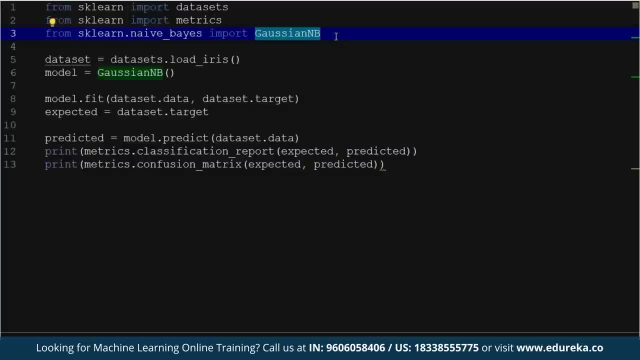 knife based classifiers. and why have done this? is because I had visualized it and I came to know that it was a normal distribution. Okay, so I load the iris- that is the load iris data set- and I load a model, and then I'm just going to fit the model. 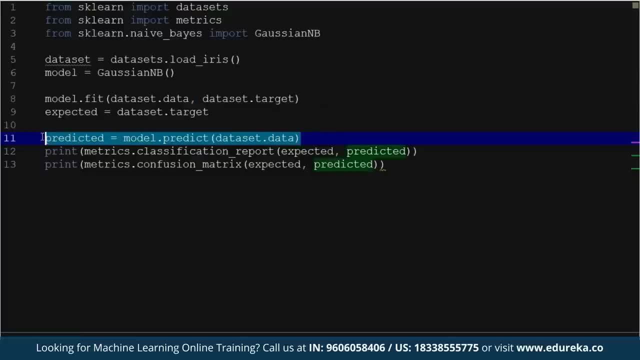 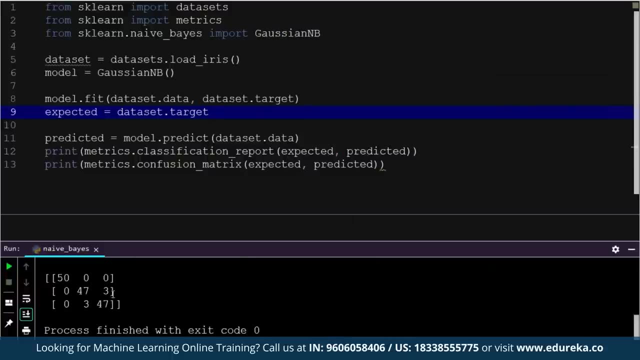 Okay, then I'm going to get the predicted model of it and then them just going to, you know, basically find all the metrics of it. So basically let me show it to you. What is the precision recall of all of that? So this is all the accuracy. then my model has an accuracy. 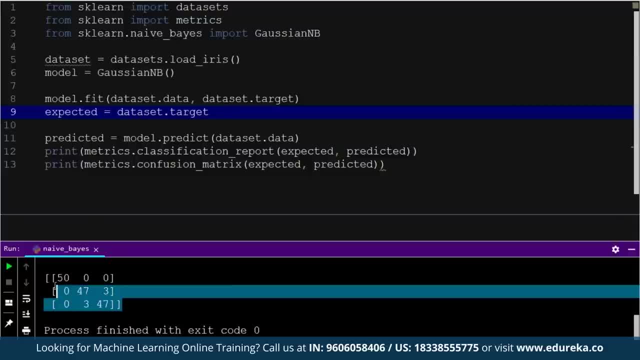 It's an accuracy of 96% and this is the confusion Matrix, which means that out of 50, it was able to classify all the 50 correctly. then, out of 50, it classified 47 correctly and three were wrong. and then, out of 50- again over here, three were classified wrong. 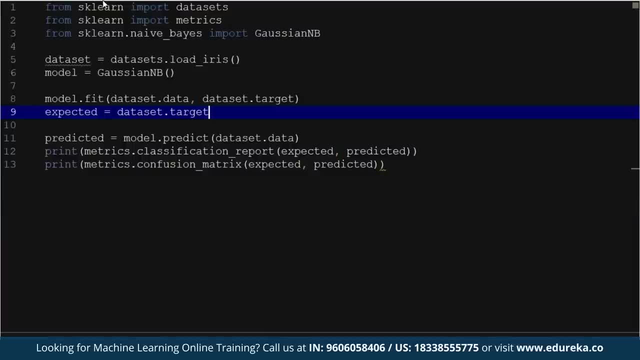 and 47 were classified correct. So this is the knife based classifier. So, as you can see, probability is actually being used in all of this. the Gaussian and a base classifier already does all of that, So we do not need to, you know, worry about it much more. 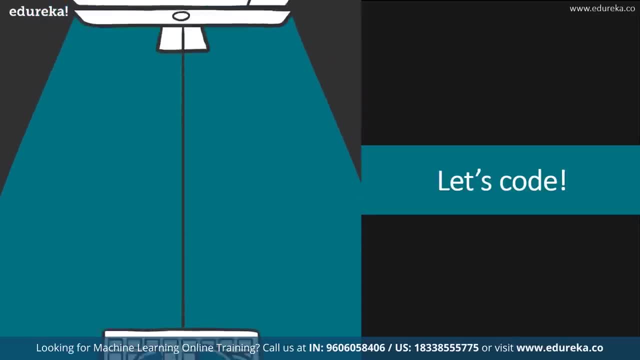 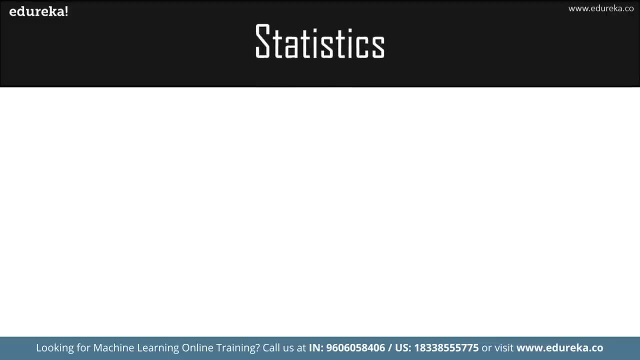 So, now that we have finished up everything that we needed to do from probability, let's move over to the last topic for today: statistics. What is a statistics? statistics is an area of applied mathematics concerned with data collection, analysis, interpretation and presentation. What this means is that you are going to analyze, understand all the data. 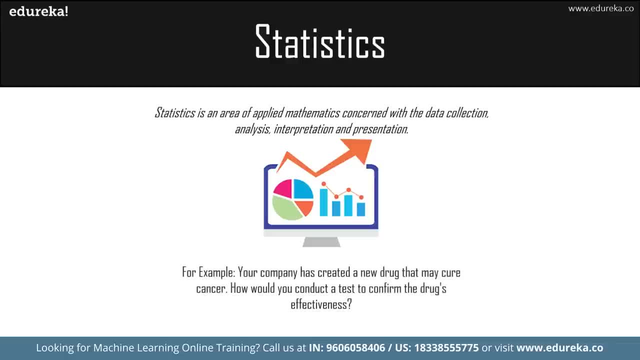 that you've collected and how you're going to present it. So, for example, your company has created a new drug that make your cancer. How would you conduct a test to confirm the drugs effectiveness? What are you going to do? You are basically going to collect a large amount of people around. you're going 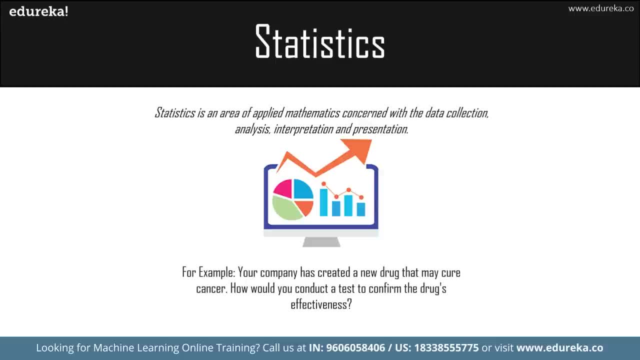 to take all of those people you're going to, you know, give them the, basically the new drug that you have created, and then you're going to interpret all the results that you get from it and then you're going to present that out of, let's say, thousand people around 900. 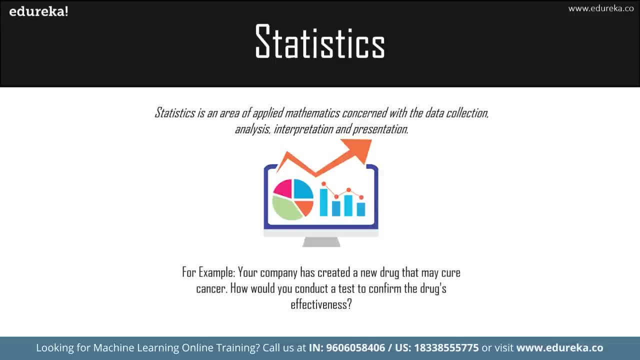 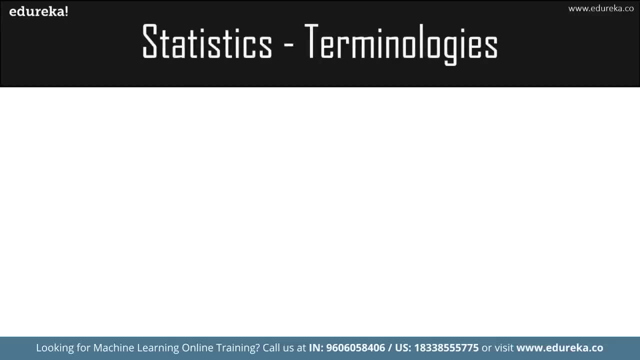 of them were cured or 950 record, So all of those parts come under statistics. Okay, so I hope you've understood that. what are the terminologies that you need to understand when you work with statistics? there is population and there is some. so what is population? it is the collection. 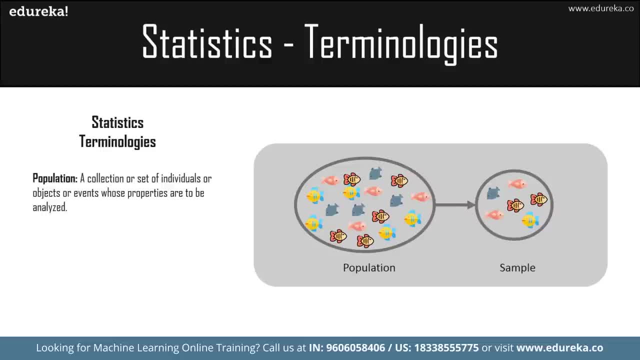 or a set of individuals or objects whose properties are to be analyzed. all the data that you have collected is called as the population. So out of all the data that you've collected, you take out a set of data for your analysis. That set of data is called a sample. 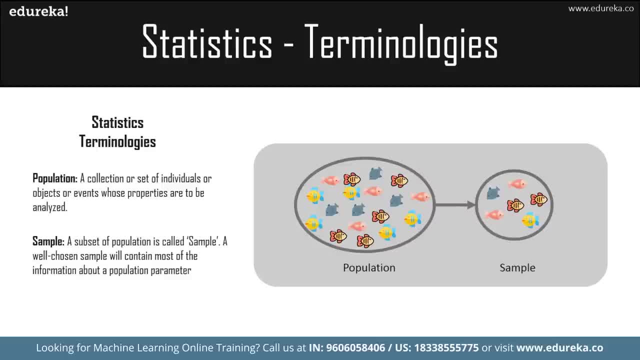 So what is the sample? a subset of the population is called as a sample, So a well-chosen sample will contain most of the information about the population parameter. So how do you choose the sample? The sample needs to be chosen such that all the data that the population is trying 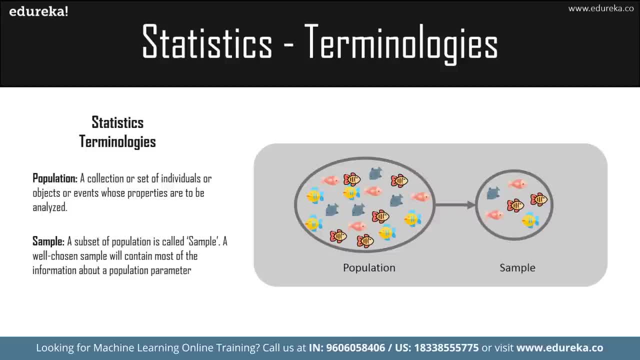 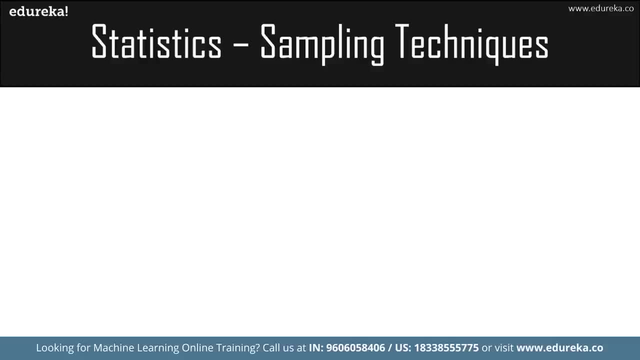 to convey can be conveyed through the sample itself. So that is what is: population and sample. now that we've understood the basic terminologies, Let's look at some of the sampling techniques that we have Have in statistics. so sampling can be classified as probabilistic. 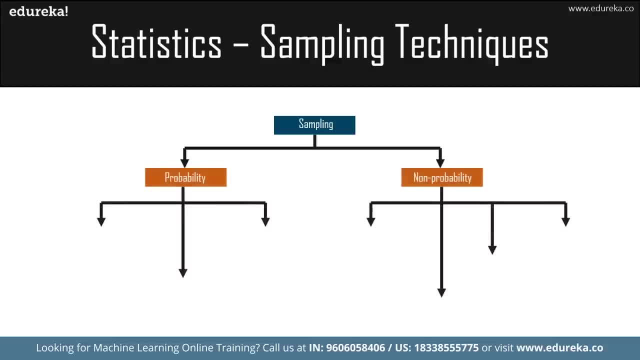 and non-probabilistic type of approaches. So in probabilistic sampling we have a random sampling, systematic sampling and stratified sampling. in non-probabilistic one We have snowball quota judgment convenience and all of that. Okay so, but for machine learning we do not need to take a look at the 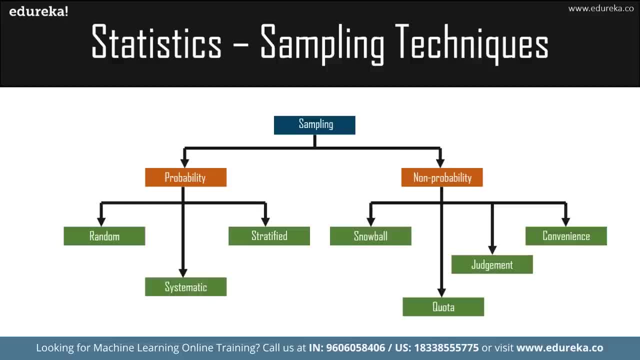 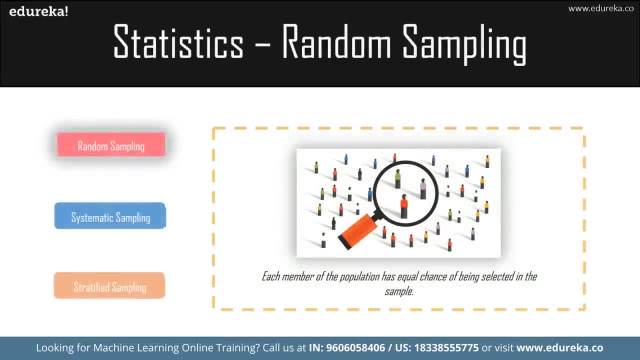 non-probabilistic approach. We just need the probabilistic approach. So we will be now covering about random sampling, systematic sampling and stratified Sampling, So let's go ahead with that. So what is random sampling? you take out a sample randomly out of the population. 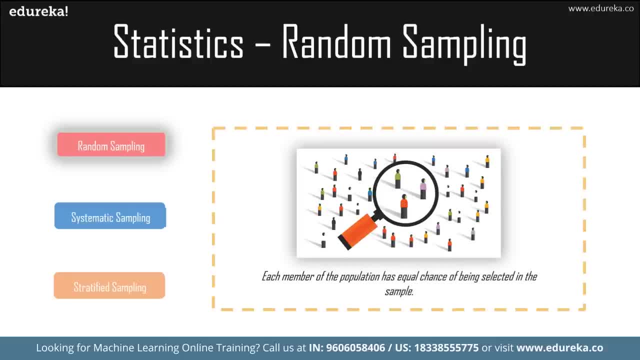 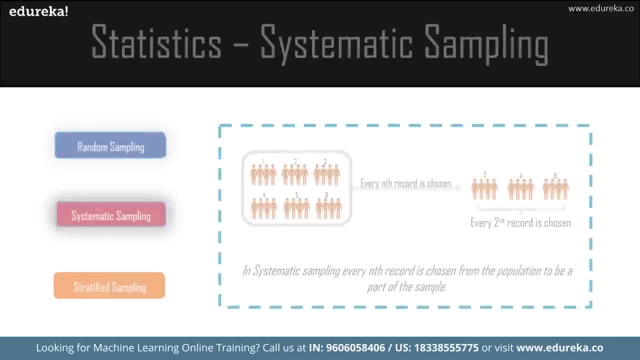 that is basically what is random sampling. each member of the population has an equal chance of being selected in the sample. So that is what is random sampling. So what is a systematic sampling? systematic sampling is basically you follow a particular order, out of which how the sample has to be taken, taken as. 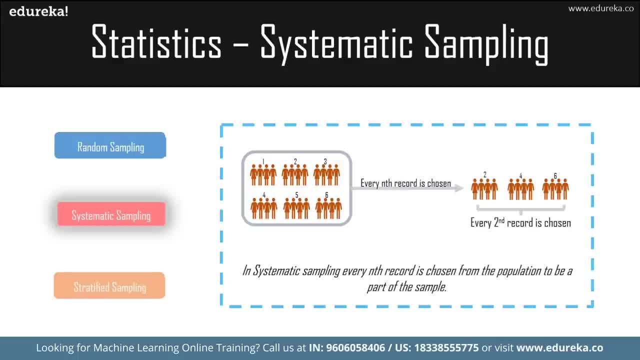 you can see here I have six particular groups. now from this six particular, I'm going to take all the even ones right. So that will be two, four and six. that is basically how the systematic sampling works. I follow a system, I follow an order of how I'm going to take the sample. 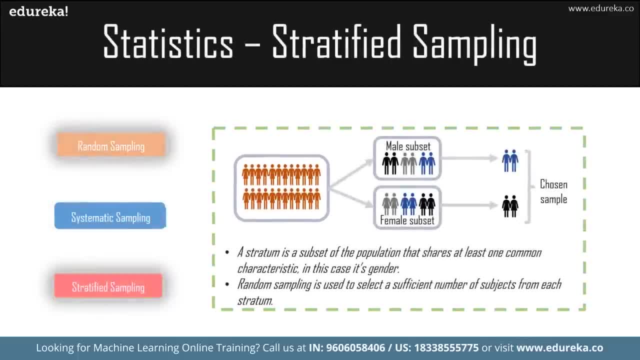 So, once we are done with that, what is stratified sampling? What is a stratum? first of all, a stratum is basically a subset of the population that shares at least one common characteristic, which is the gender, which I have taken over here here. 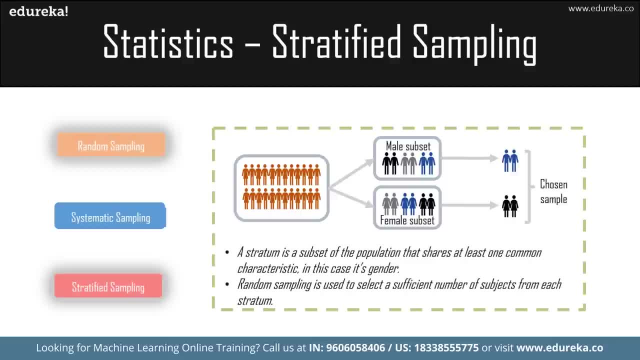 So, as you can see, here I have the whole population, Out of which I have found out one property that is common between all of them, that is, gender. They are either male or female, So I'm going to break the whole population based on that. 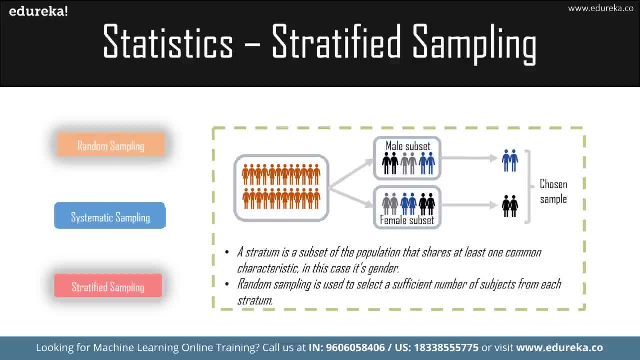 I'm going to break my population into the male subset and the female subset. So after that, I'm going to apply the random sampling and I am going to take out all the samples that I am going to be needing. Okay, So, once I have now broken down my particular subsets, now I'm just going. 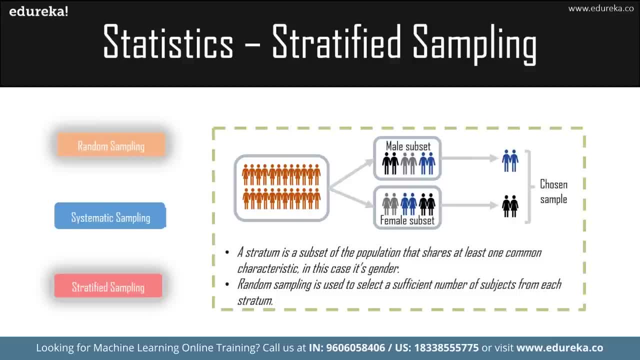 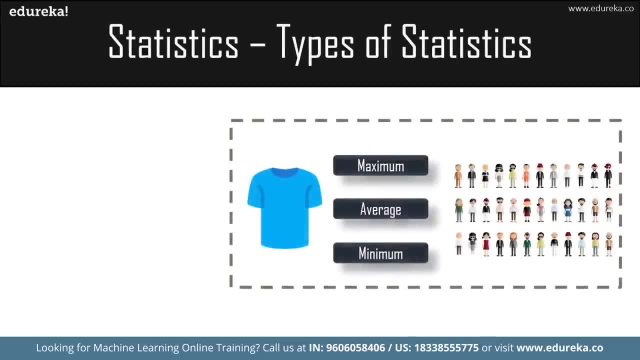 to be using random sampling And take out all the samples that are required by me. So this is what is stratified sampling. So what are the types of statistics that we need to infer from from? we have descriptive statistics and inferential statistics, So let's understand each of these right now. 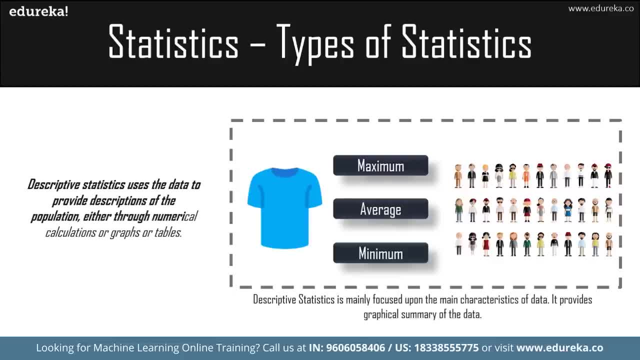 Okay, So what is descriptive statistics? descriptive statistics is mainly used to focus upon the main characteristics of the data. It provides the graphical summary of the data. So, as you can see over them, Descriptive statistics uses the data to provide descriptions of the population, either through numbers or calculations, or graphs or tables. 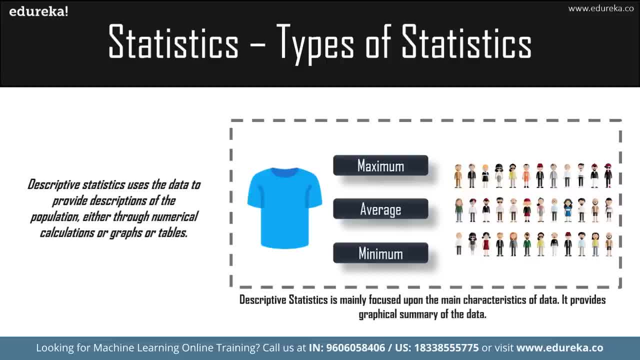 Okay. So, as you can see, here I have my short and there can be either three particular sizes that can be the most minimum one, the most average one and the most maximum one, and all of that is based on the weight of the person. suppose, for example, if a person weighs 60, he's going to get the 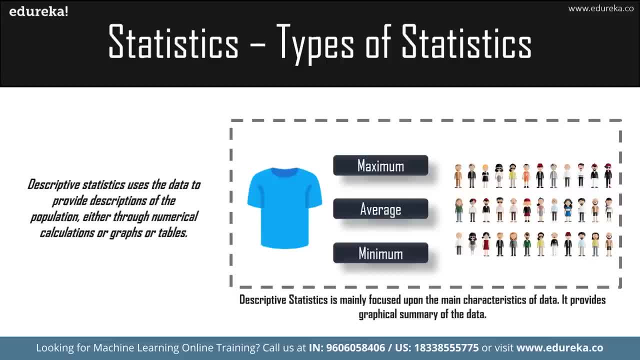 maximum one. If the person weighs 40, he's going to get the average one. the person weighs 20, he's going to get the minimum one. So that is how I am describing my data and I'm going to infer data from it. So that is descriptive statistics. 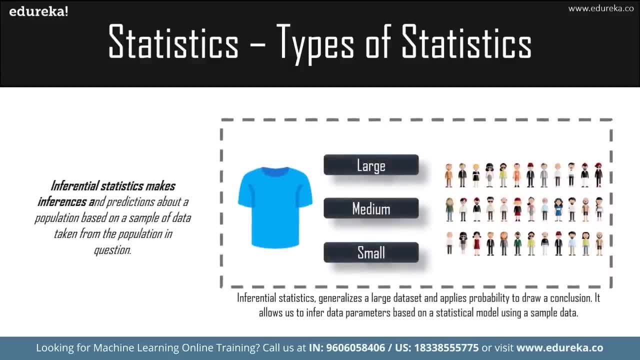 So what is inferential statistics? inferential statistics makes inferences and predictions about a population based on the sample that is being taken from it. So what this means is basically I'm going to generalize a large data set and apply probability and draw a conclusion to it. 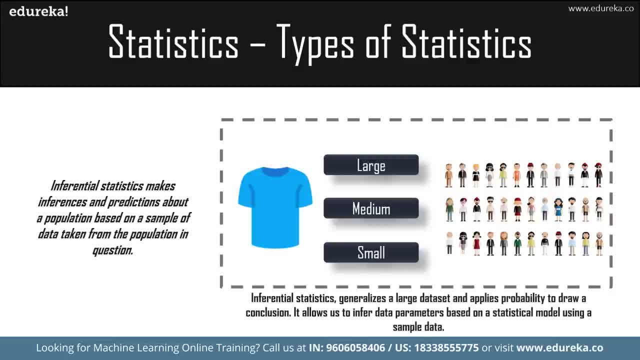 So it allows me to you know inferred data parameters based on the statistical models, which is using the sample data. I have a whole bunch of population out of which they can tell me they have either the large size or the medium size of the small size is so. 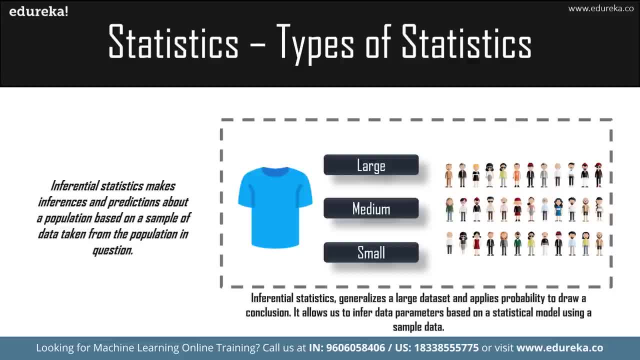 according to their sizes. I'm going to supply them the t-shirts. So this is basically what are the two types of statistics? there are descriptive statistics and inferential statistics. descriptive statistics: What does it do? It describes the data, whereas inferential statistics takes information. 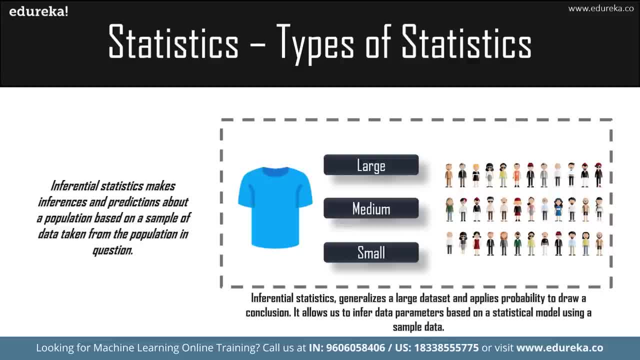 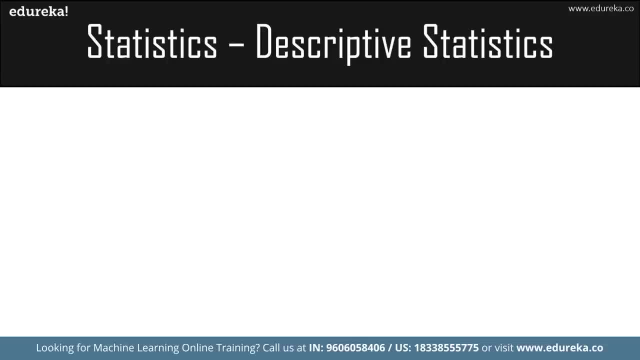 from the data and then analyzes accordingly to our we wanted to. so these are the two types of statistics. Let's go in depth with descriptive statistics. What is descriptive statistics? it is used to describe and understand the features of a specific set of data. So what is descriptive statistics? 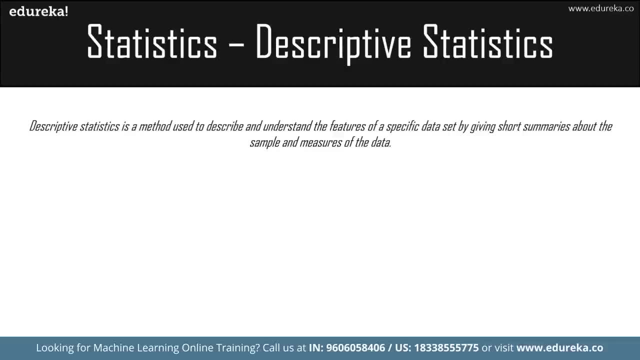 It is a method used to describe and understand the features of a specific data set by giving short summaries about the samples and measures of the data and descriptive statistics. It is broken down into the measures of Center and the measures of variability. So what does measures of Center have? measures of Center has the mean. 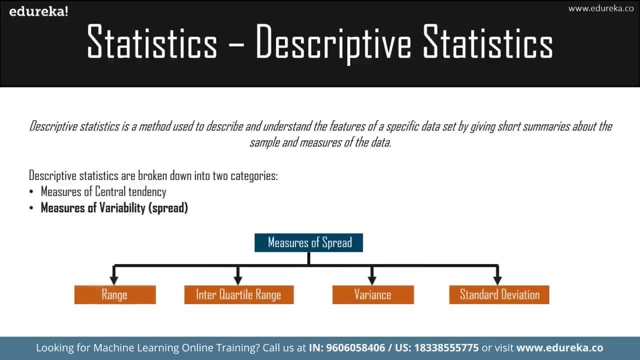 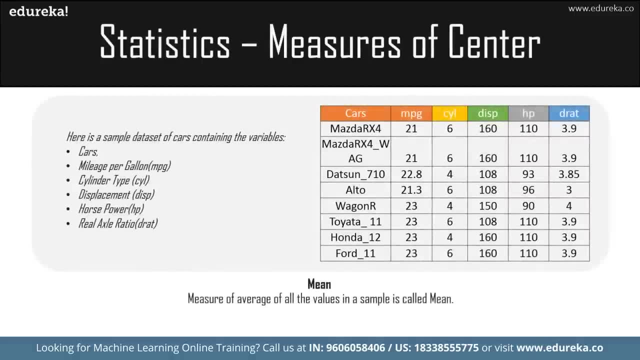 median and the mode, whereas the measures of Center have the range, interquartile range, variance and standard deviation. So let's understand all of this right now. So, for example, here you can see that I have a data set of a car which contains the variables, the car, 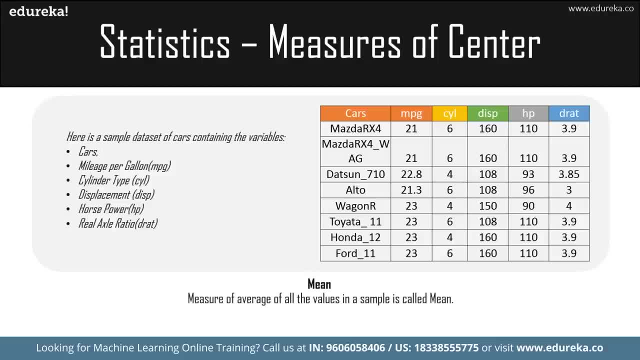 The mileage, the cylinder type, the displacement, the horsepower and the real lax ratio. So I'm going to find out the mean. so what is a mean? mean is the average of all the samples. So, for example, if I want to find the mean of the horsepower, I'm going 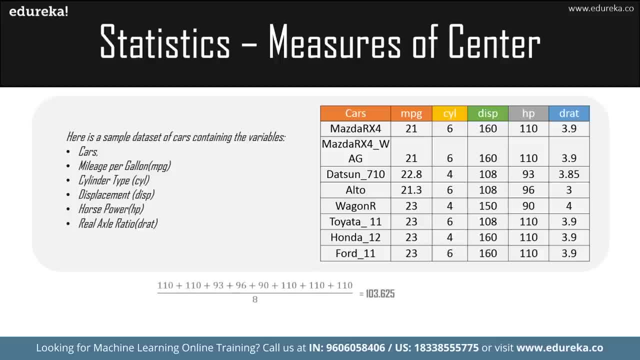 to just add the values and divided by the number of values. So I get a hundred and three point six to five. This is the mean of the horsepower. So what is the median? It is the measure of the central value of the sample set. that is what 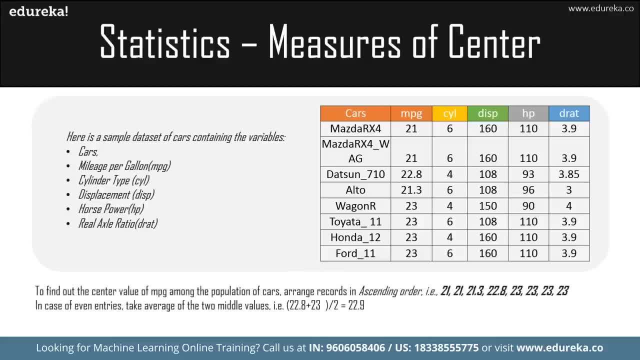 is a median, So let me show you how to find it for the miles per gallon. to find the order of the center value, You have to basically arrange it in the ascending order. Okay, So you have 21, 21, 21.3, 22.8, 23, and accordingly, now I have to take the. 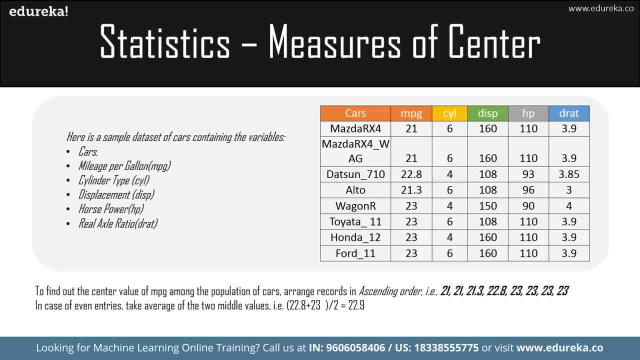 two middle values. Okay, Okay, so that will be 22.8 plus 23. divided by 2, that becomes 22.9.. So that is the median of my sample. next Let's move over to more, the value which is most recurrent in the sample. 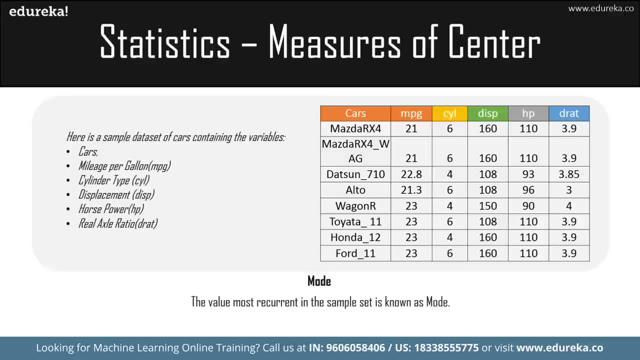 set is called as The mode. So let me find the mode for the cylinder type. What is most reckoning, the six-stroke or the four-stroke? I can see here that there are one, two, three, four, five. So there are five times that the cylinders type of six-stroke has been. 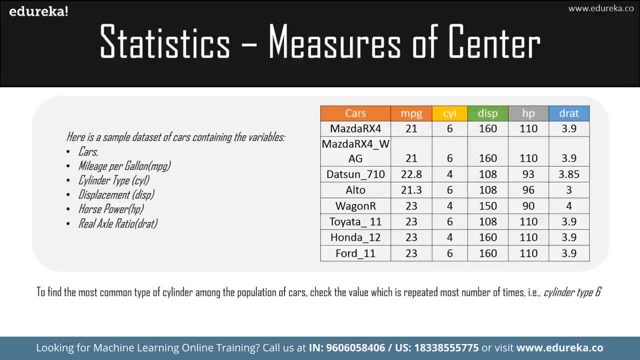 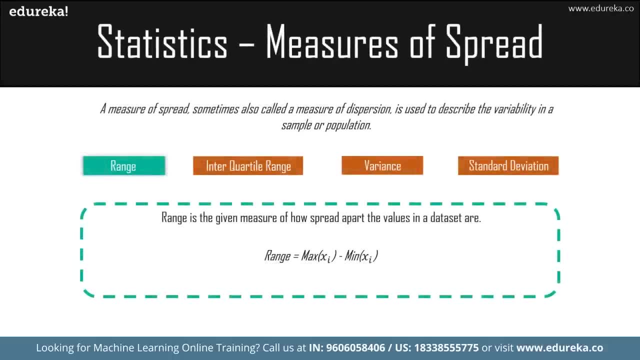 repeated, and three times cylinder type four-stroke has been repeated. So six becomes the mode of the data. Okay, So now that we have understood all that is required from measures of Center, Let's move over To the measures of spread. so a measure of spread is also called as a. 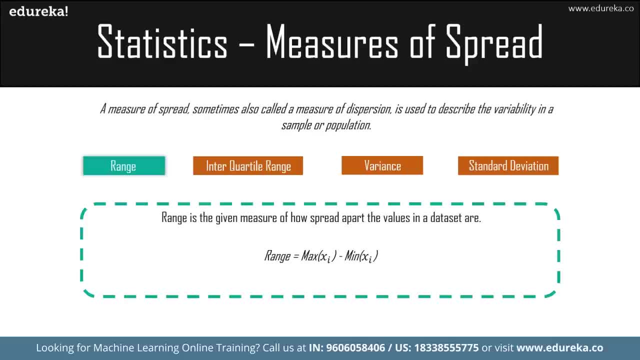 measure of dispersion is used to describe the variability in the sample or the population. Okay, So the first one is a range. range is the given measure of how spread apart the values are in a data set. So it is the maximum value minus the minimum value which gives us the 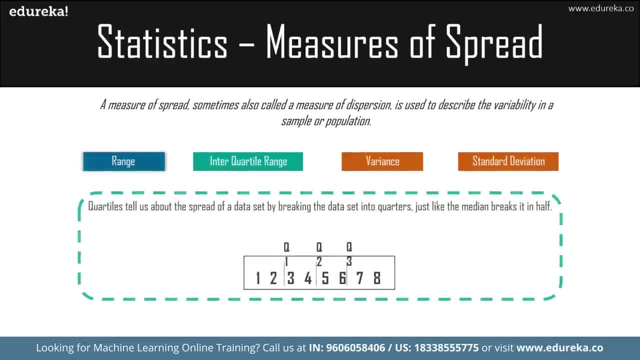 range. So what is an interquartile range? quartiles tell us about the spread of the data by breaking the data into many, many quarters, Just like the median breaks itself. So, for example, if I have eight data's over here, I can break it down. 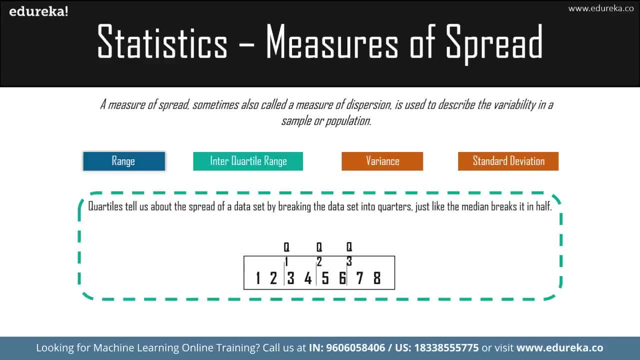 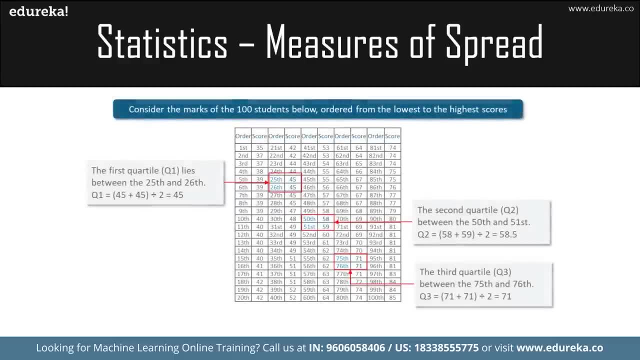 into three quarters, where I have a 1, 2, then I have 3, 4, 5, 6 and 7, 8, which become different, different samples accordingly. Okay, How do I find what is the interquartile range? So how will I find the interquartile range of this? 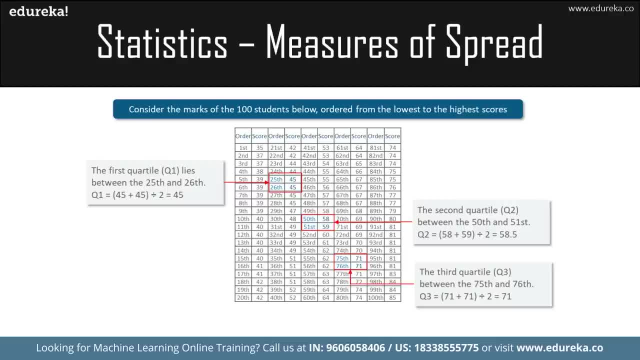 Okay, So the first quartile, q1, comes between the 25th and the 26th, So it will be 45 plus 45. divided by 2, that becomes 45. The second one comes under 50 and 50 first, and that will be 58 plus. 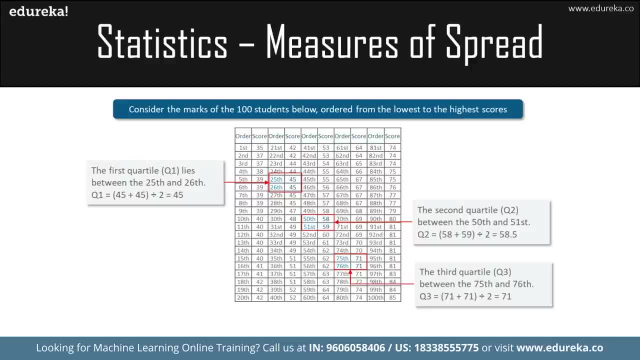 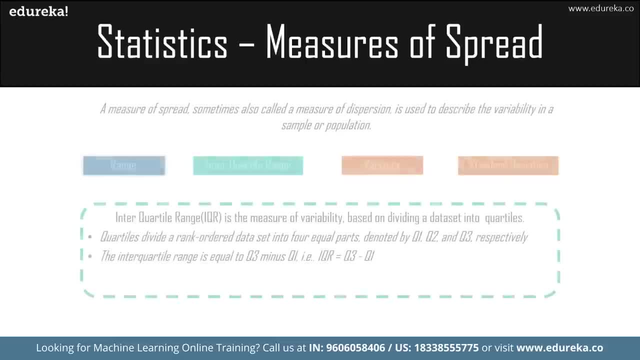 59 by 2, that will be 58.5, and the next one comes at 75 and 76. that is 71 plus 71 divided by 2, which is always 71. So that is basically what is an interquartile range. 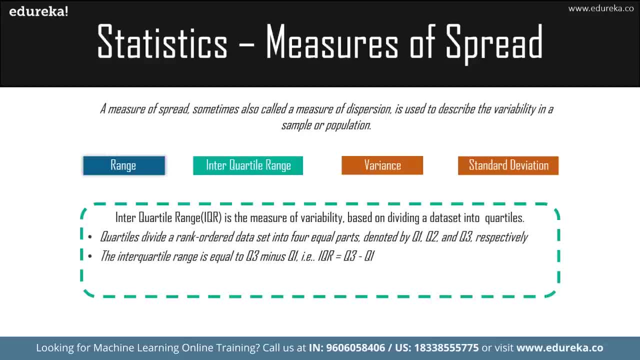 It is the measure of variability based on the dividing set into the quartiles. So that is basically how you break down the interquartile range and it is the measure of variability based on dividing the set into quartiles. So quartiles divide a rank order data set into four equal parts. 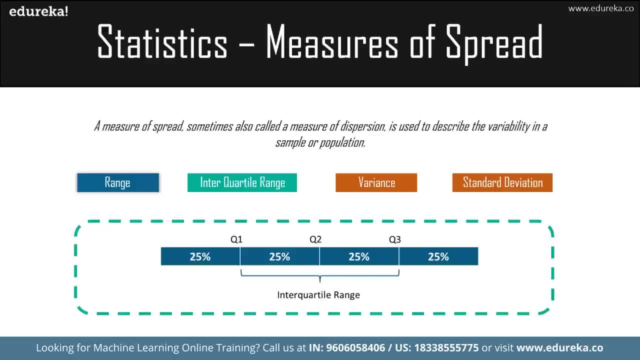 which will be q1, q2 and q3 respectively, and the interquartile range is measured by q3 minus q1.. So, if you can see this, you have the whole data, which is 100%, and you have broken down the data into 25% each. 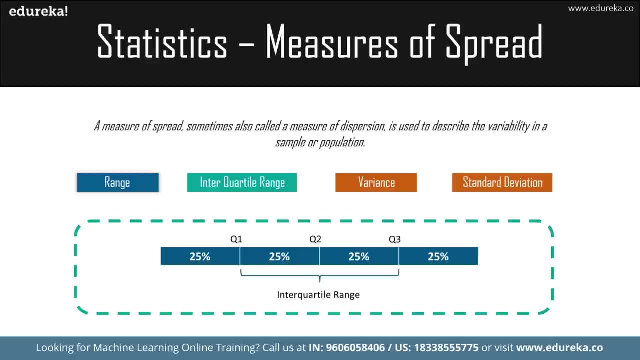 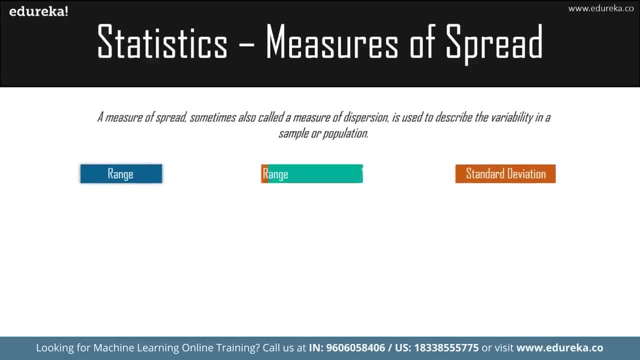 So the quartiles come in between the first q1, q2 and q3.. So those are the interquartile ranges. So now that we've understood that, let's move over to Variance. so variance describes how much a random variable differs. 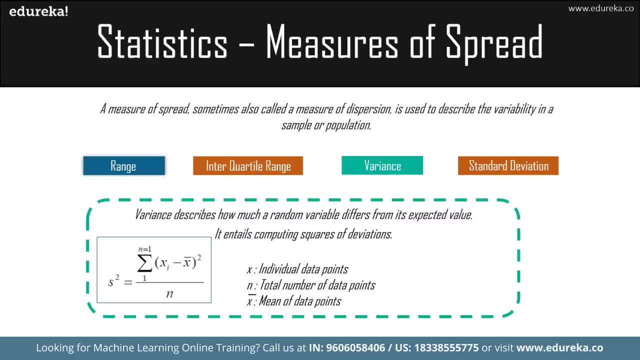 from its expected value. It entails the computing squares of the deviations. So that is how you find the variance, which is: s square is equal to the summation of 1 to n, is equal to 1, X I minus X, bar the whole square divided by n. 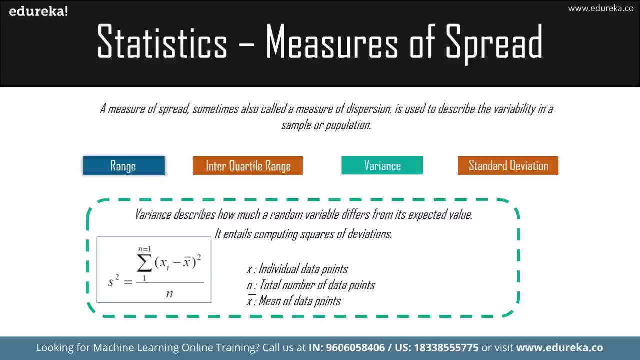 So X I is the value and X bar is the mean. I hope that simple for you to understand. What is a variance mean? it means the difference between the data, which it should have Actually been. so what does the variance actually try to tell you? 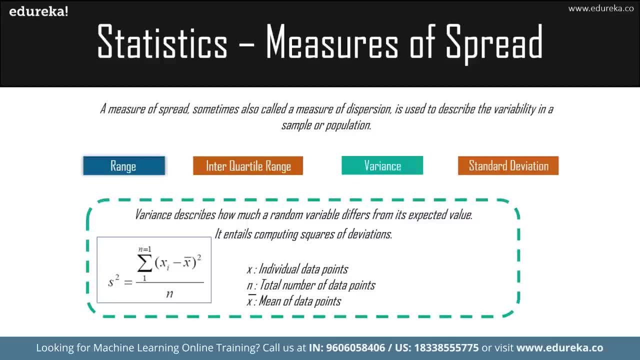 Okay, it basically means that the data, which should have been something, and what it really is. What is the difference between them? How much it differs from each other? So that is what is the variance? So what is a standard deviation? deviation is the difference between: 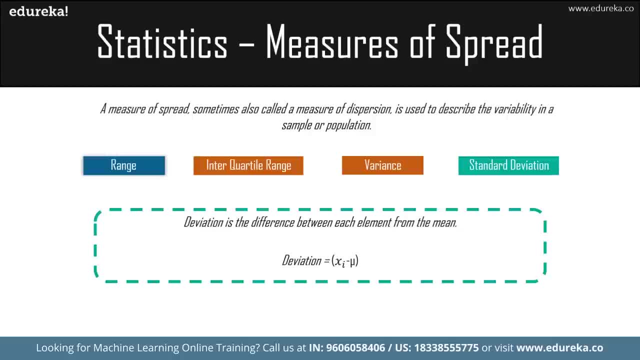 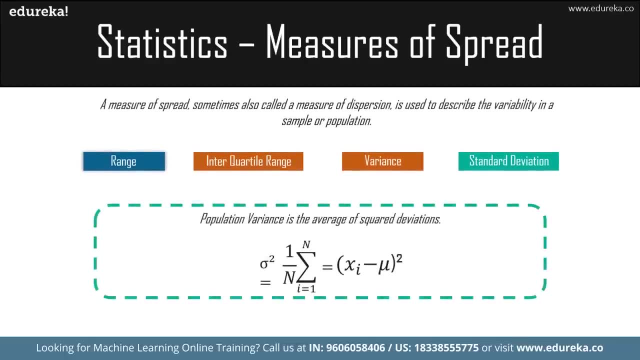 each element from the mean. so I have X, I and I have the mean. what is the difference between each of them? is the deviation. So what is the population variance? The population variance is given by this particular formula, that is: Sigma square is equal to 1 by n. the whole summation of I is equal. 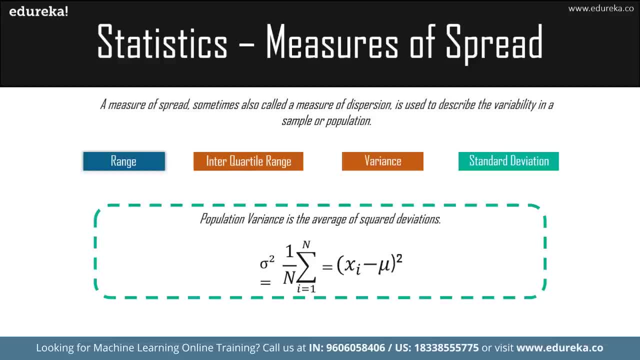 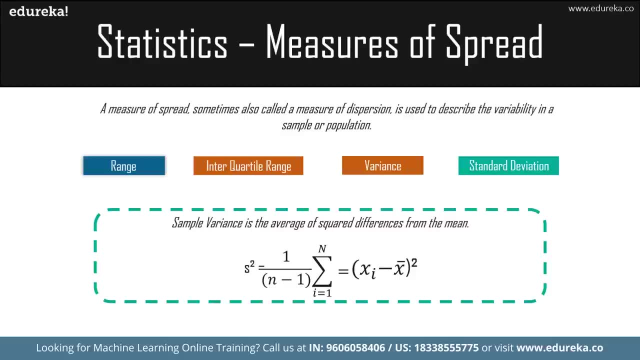 to 1 to n is equal to X I minus mu, the whole square. once we have found out the population variance, What is the sample variance? So it is s square is equal to 1 divided by n minus 1, the summation of I equal to 1 to n and X I minus X bar the whole square, that is. 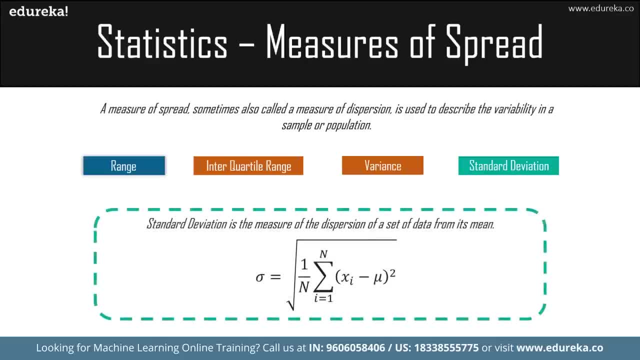 the sample variance. So what is the standard deviation? Standard deviation is the measure of the dispersion of a set of data from its mean. what the standard deviation is trying to tell you is basically that how much this data is trying to disperse from its actual data. 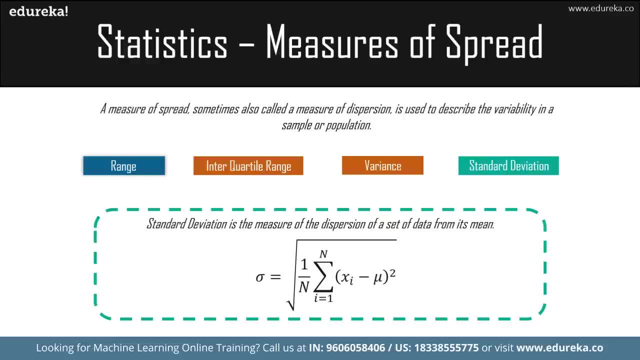 So how is that? given by? it is given by 1 divided by n, summation of I equal to 1 to n, X, I minus mu, the whole square, which is basically the variance, is square root. So that is standard deviation. So how do you find the standard deviation? 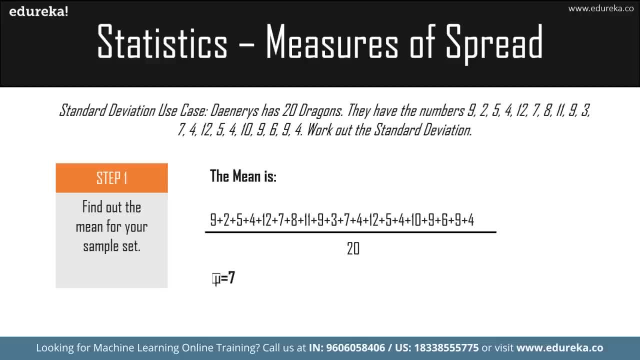 I'm just going to give you an example Over here. So see, for example, Daenerys has a 20 dragons and they have the numbers accordingly. So how do you work out the standard deviation? So the mean is given by adding all the numbers, dividing it by 20.. 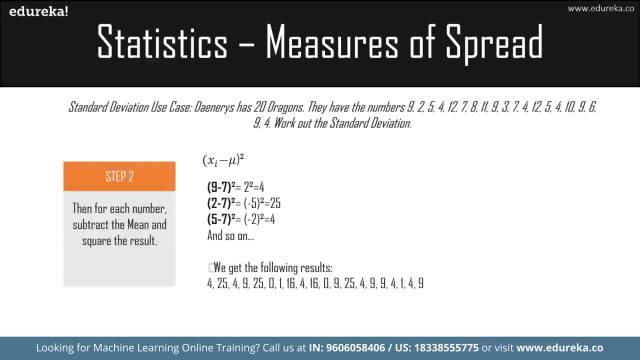 So mu is equal to 7. and then what is the standard deviation? So it will be X, I minus mu, the whole square. So it will be 9 minus 7. the whole square is equal to 2, square is equal to 4 and you have 2 minus 7, you know all. accordingly, you keep. 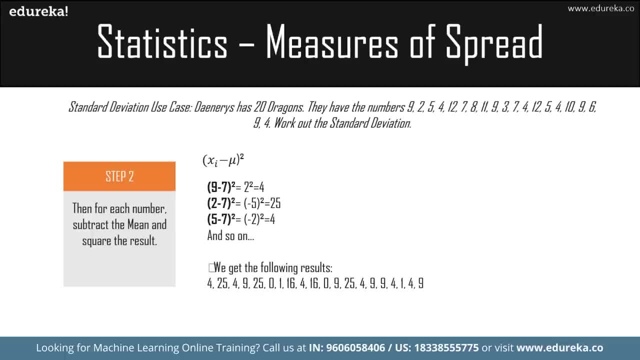 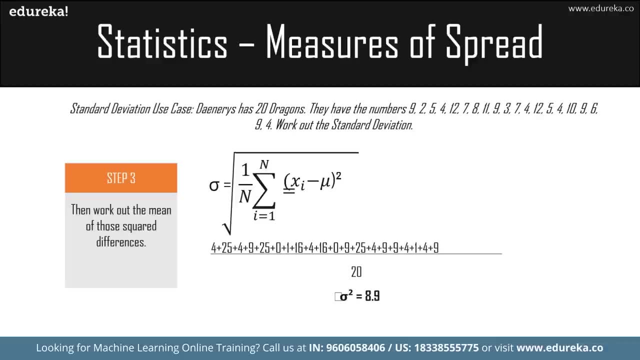 on going and you get the following results: Which is 4, 25, 4, 9, 25, 0. accordingly. Once you have done that, put that into the formula, So you have this formula accordingly, So we get. the variance square is equal to 8.99 and the standard deviation. 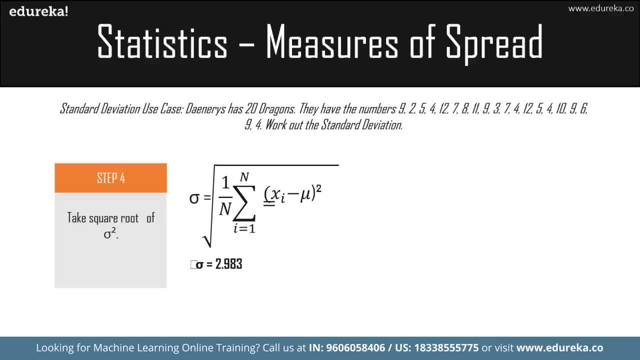 will just be the square root of 8.9, which will be 2.983.. What this means is that with the value of 2.983, the values are differing from the mean. So if you are trying to add 2.983 to all the other values, you will. 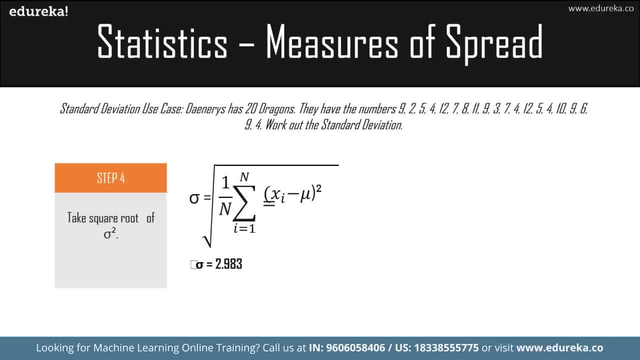 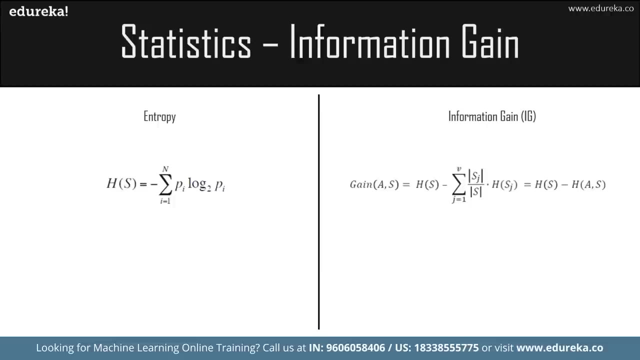 be getting something which is much more similar and much more realistic and much more, you know, closer to the mean of the. so that is how standard deviation works. now that we've understood all of that, We have a very classic example of information gain. So what does information gain help us with? this is an ideology. 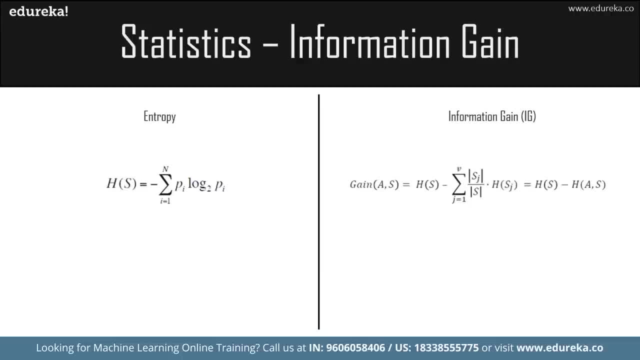 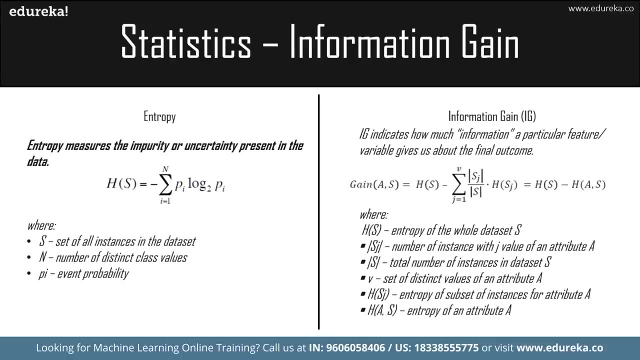 that comes into picture for decision trees. So let's understand the basic concepts of what we require in information again. So the first topic that we need to understand is information Entropy. So what is entropy? entropy measures the impurity or uncertainty that is present in a data and it is given by the formula HFS is. 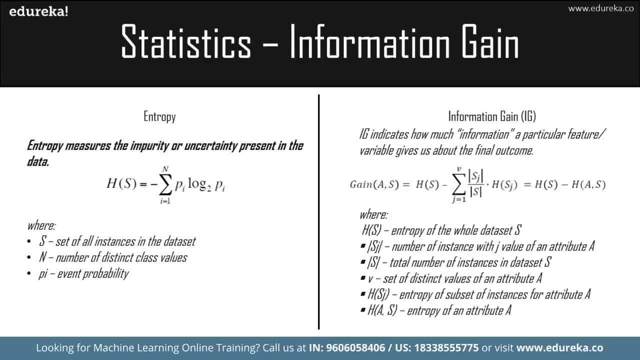 equal to minus summation of minus 1 to the power of n. P of I. log base to P of I, where S is all the instances in the data set and is the number of the distinct class values and P of I is the event probability, because entropy is the impurity that a data has. 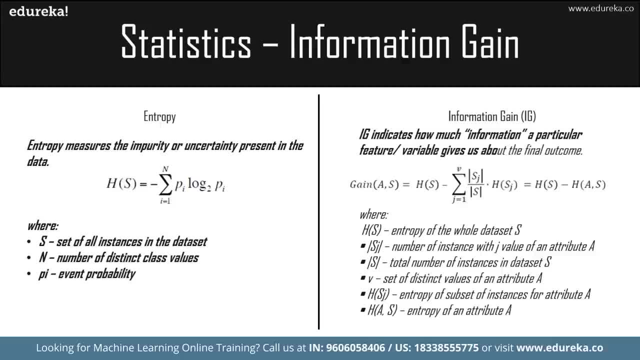 So what is information gain? information gain is how much information a particular feature will give to the final outcome. So that is given by: gain of A of S is equal to HFS, which is the entropy minus summation of J is equal to 1 to V s of J divided by. 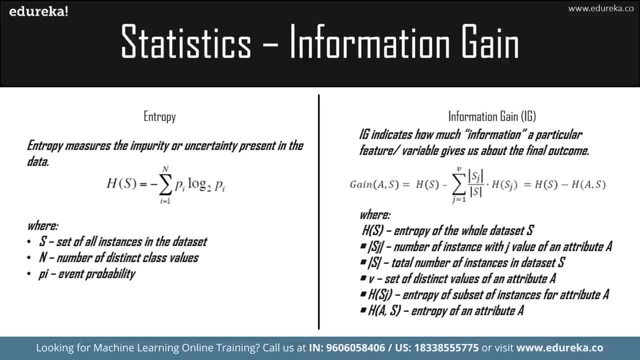 J into H of S of J is equal to H of S minus H of A by S. H of S is the entropy of the whole data set. S of J is the number of instances with J and a value of attribute a. s is the total number of data sets. 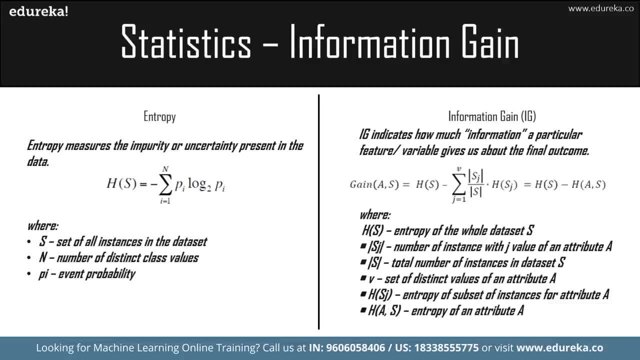 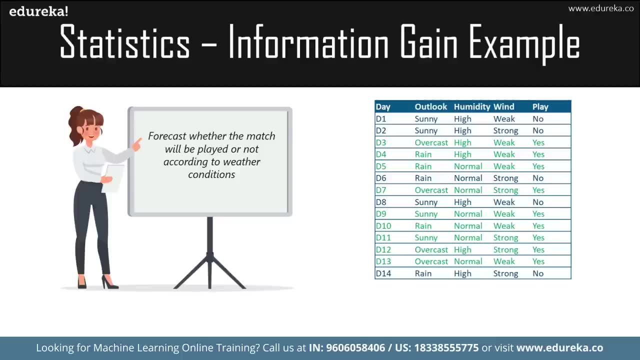 B is the distinct value of attribute A, H is the entropy of the data set with value a and entropy of attribute A. so these are all the requirements. So let me give you an example of information gain. You can see the data set over here, which is for 14 days, and the 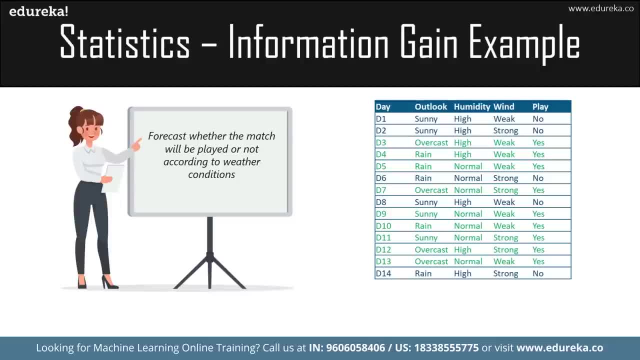 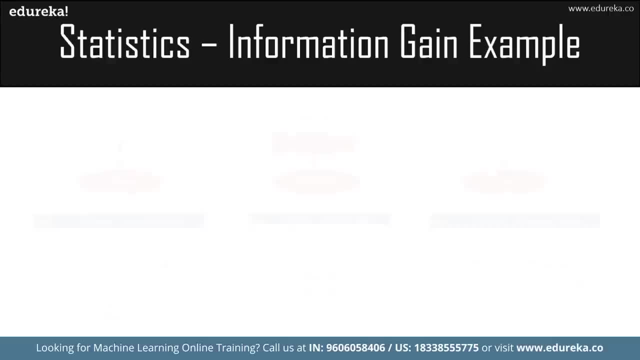 particular, you know attributes that are given to it. So the forecast is to find out whether the match will be played or not, according to the weather conditions. So this is what we are trying to find here. We have Five knows and nine yeses. 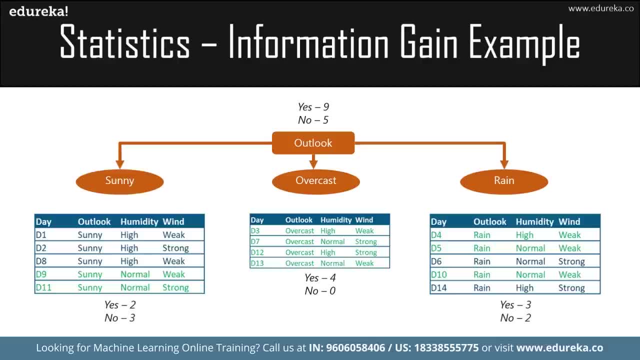 So we have the outlook, and then we have a sunny, overcast and rainy. So in sunny we have three nose and two yeses. in overcast We have a four yeses and zero nose, and in rainy We have three Yes and two nose. 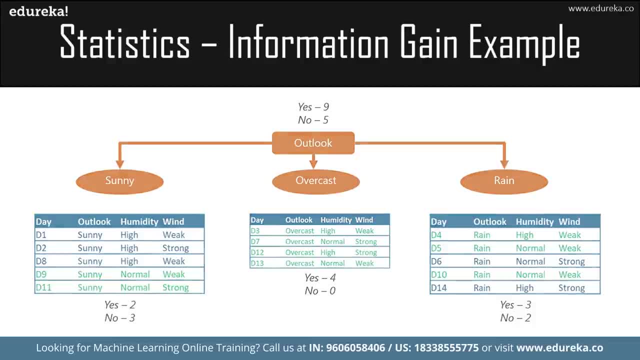 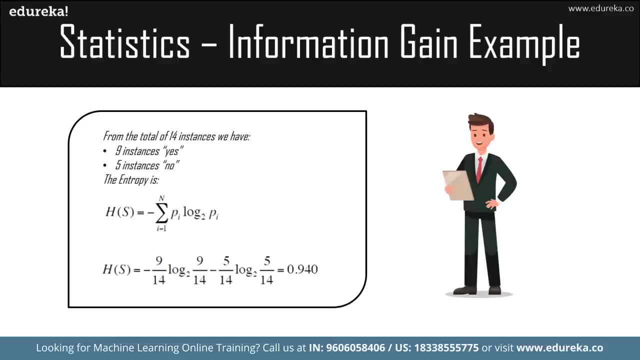 So how are we going to find out which particular node is going to, you know, attribute the most of it? So let's find out the entropy first for the whole data, which is nine instances Yes and five instances say no. So we have a minus 9 by 14 log base 2 of 9 by 14, minus 5 by 14 log. 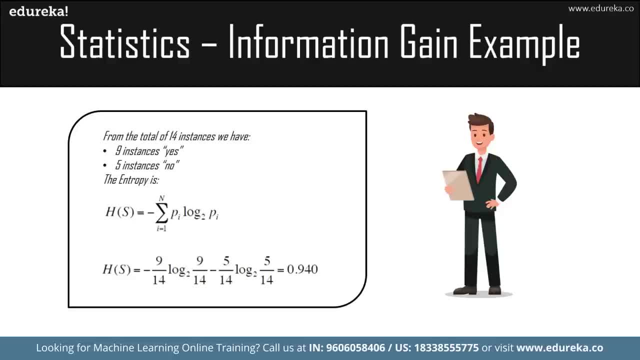 2 of 5 by 14 is equal to 0.9 for zero. So what this means is that the data that we have has 0.9 for 0 times. bad data means it cannot give us much information. that is much more impurity in the data. 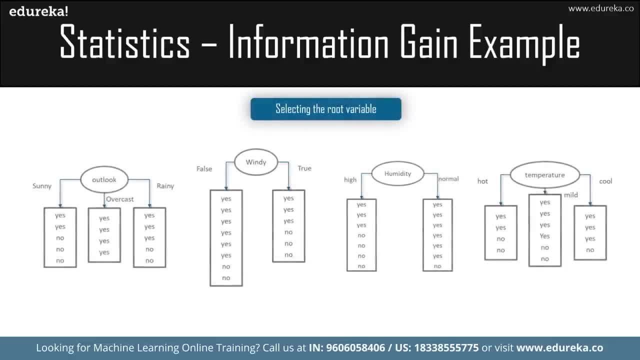 So let's move over. the first step in information gain is to find the root variable. So how are we going to find the root variable? We are going to take all of the attributes and find the information gain from them. We have Outlook, we have windy, humidity and temperature. 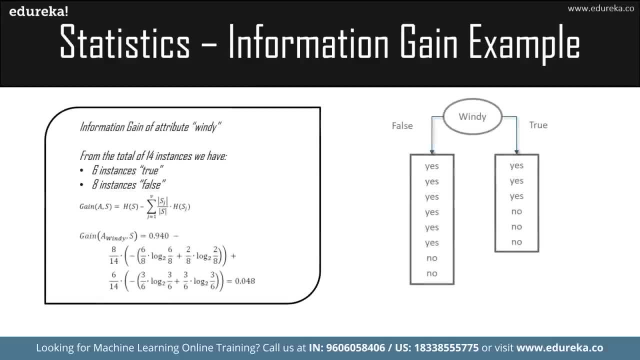 So let's find out the information gain gain. So for information gain of windy, we have six instances true and eight instances false, right? So HFS is equal to 0.9 for 0 minus 8 into 14 and as you can. 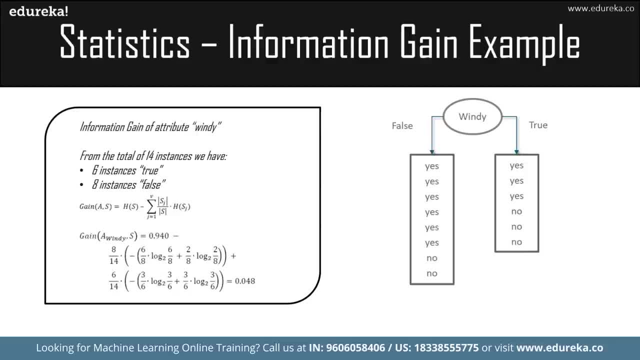 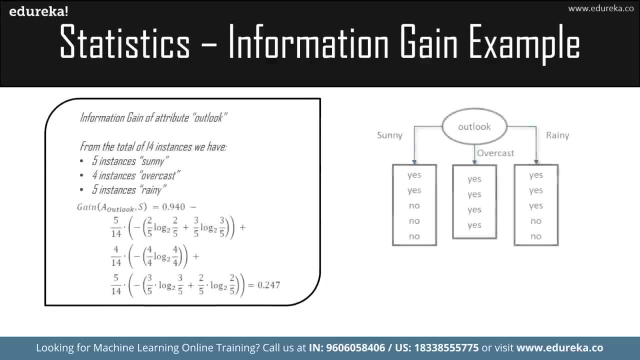 see all the other variables. So the gain that we have achieved from windy is 0.048, which is really really less So for Outlook, the same thing happens over here. We have the information gain that is being passed by. it is 0.247.. 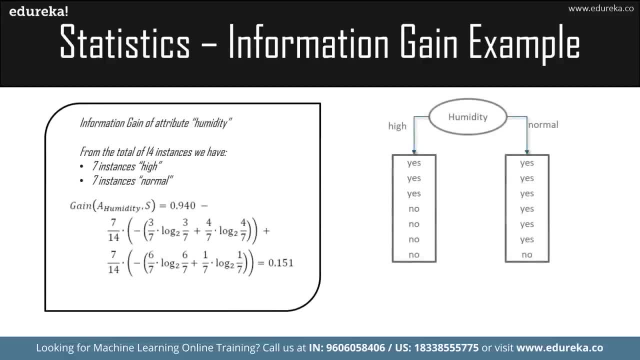 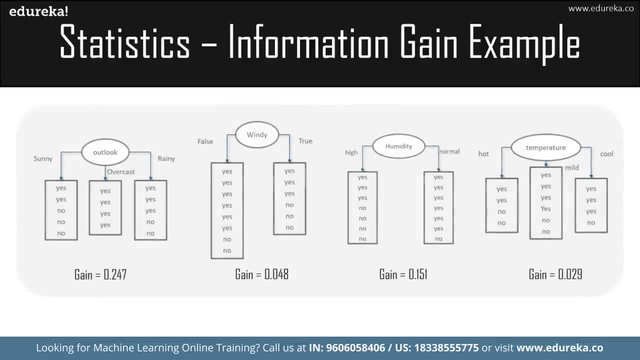 Then we have the information gain from humidity, that is 0.15, which is also really good, and then we have temperature, which is 0.029.. You can pause and look at the steps if you want to. out of all the gains that we have, the variable with the highest information. 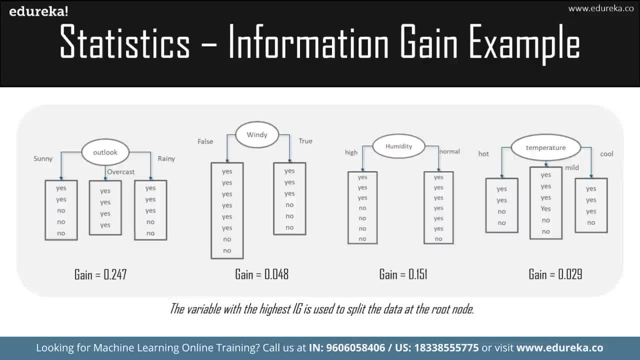 gain is used to split the data. So Outlook has 0.247.. Windy has 0.048, gain has 0.151 and gain of temperature is equal to 0.029.. So what are we going to choose? We are going to choose Outlook. 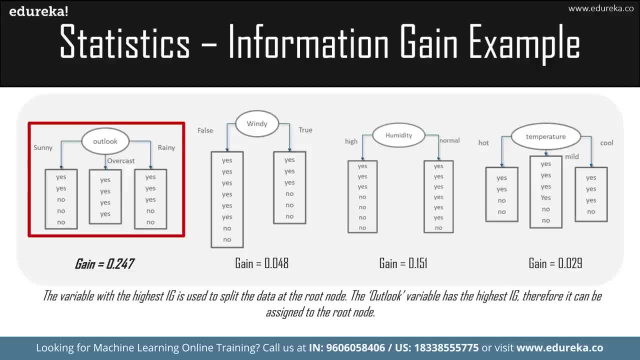 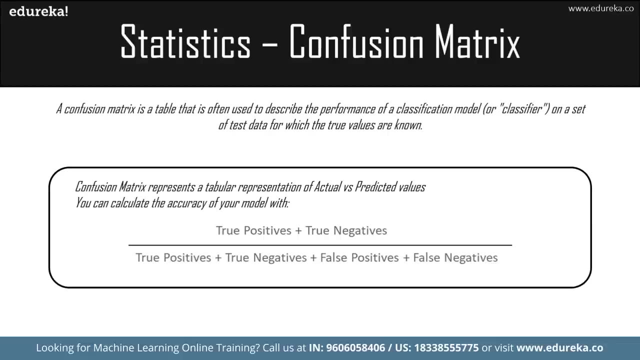 Look, why is that that? it's because it has the highest information gain. so that becomes our root node. That is a simple example of how statistics is used in the information gain. next Let's move over to the confusion Matrix. So what is a confusion Matrix? confusion- 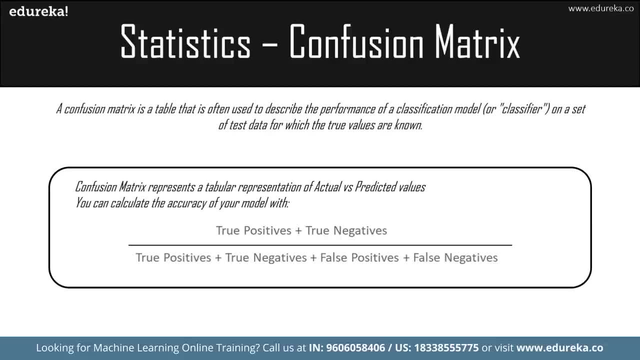 Matrix is a table that is often used to describe the performance of a classification model. So it is a table that is used to describe the performance of a classification model on the set of test data. So how are you going to calculate the accuracy of this? 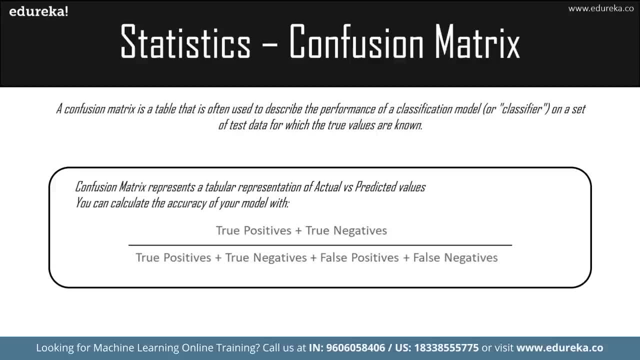 It will be two positives plus two negatives divided by two positive, two negative, false positive, false negatives. So if you are confused with port is two positive, two negative, false positives, false negatives. Let me explain that to you right now. Let's see, for example: 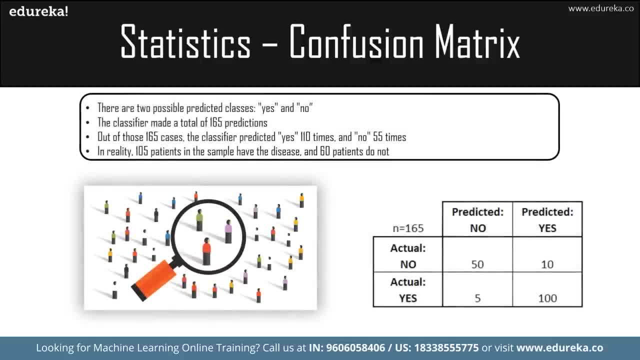 There are two possible predicted classes, which are yes or no. the classifier made a total of a hundred and sixty-five predictions. That means a hundred and sixty-five predictions were total. So out of the hundred and sixty-five cases, the classifier predicted Yes 110 times and no 55 times. 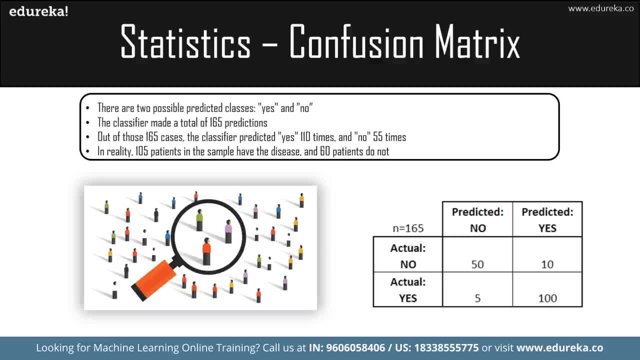 So in reality a hundred and five patients only had the disease and 60 patients did not. so how are we going to put this into the table? So, as you can see, here in the table we have, n is equal to hundred and sixty-five. then we have predicted no and predicted. 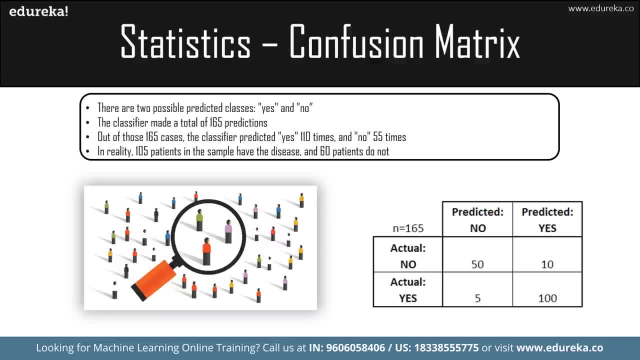 Yes, actual no and actually yes. So if our classifier predicted it no and it was actually no, that is the correct output. but if it predicted yes and it was actually yes, that is also the correct output. but it predicted it as yes and it was actually no, that means it has made a mistake and it 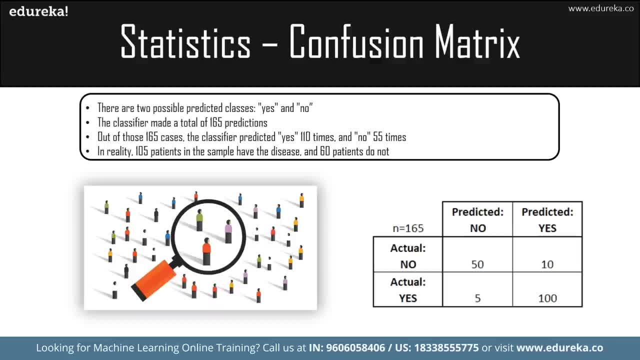 predicted no, but it was actually yes. It has still made a mistake. What are the correct values over here, which is a 50 and 100? so 50 and 100 are the correct values and 10 and 5 other wrong values. 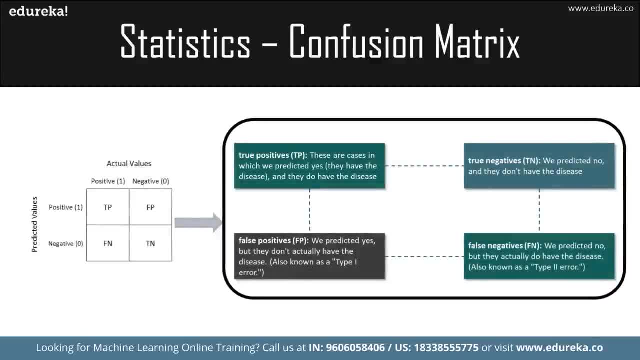 What is a true positive? to positive are which it was predicted as yes and they actually have the disease. to negatives are predicted No and they did not have the disease. false positives are classifier predicted as yes but they did not have the disease and false. 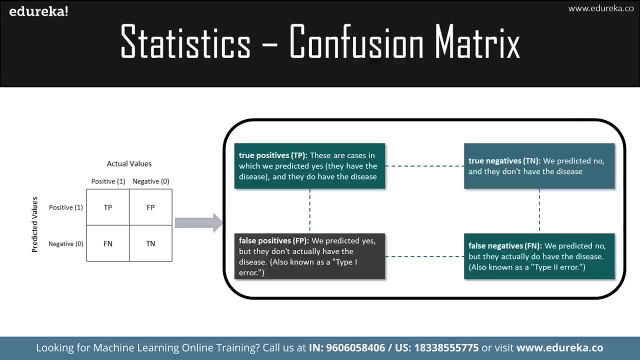 negatives be predicted? No, but they also had the disease. So this is basically what a confusion Matrix is, and it is helpful in finding out the performance of the classifier that you are working with. so that is what is a confusion Matrix. next comes inferential statistics. 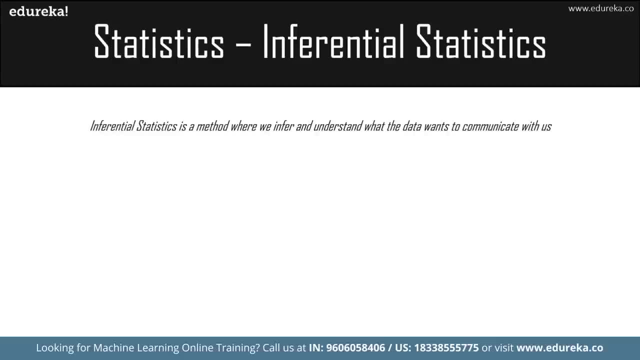 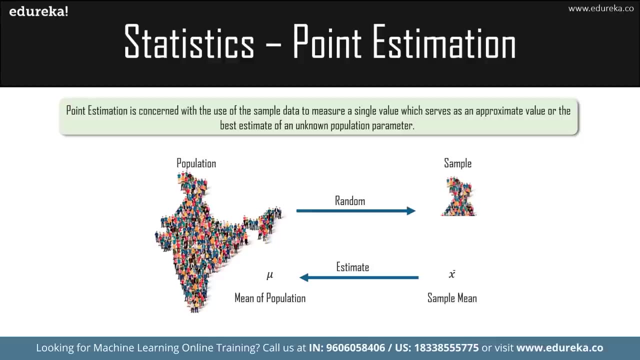 It is a method where we infer and understand what the data is trying to communicate with us. So it is broken down into two points: It is a point estimation and interval estimation. So let's understand about point estimation. point estimation is concerned with the use of a sample data to measure a single. 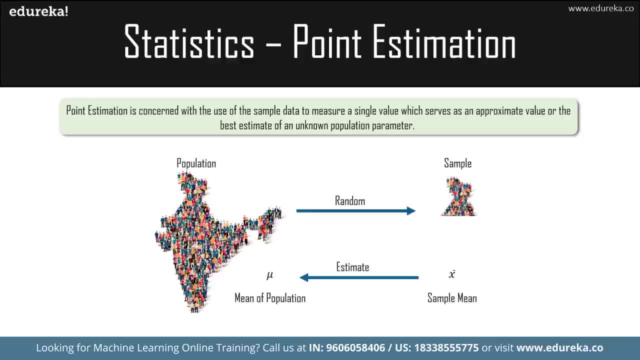 value which serves as an approximate value Or the best estimate of an unknown population parameter. So we have such a huge population of India right out of that. You're just going to randomly take out some sample of it. You're going to find out the sample mean and this sample should. 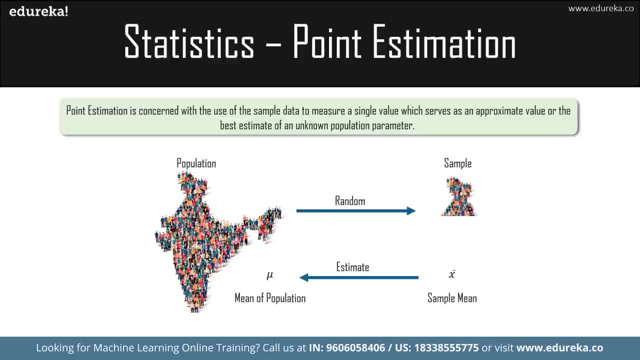 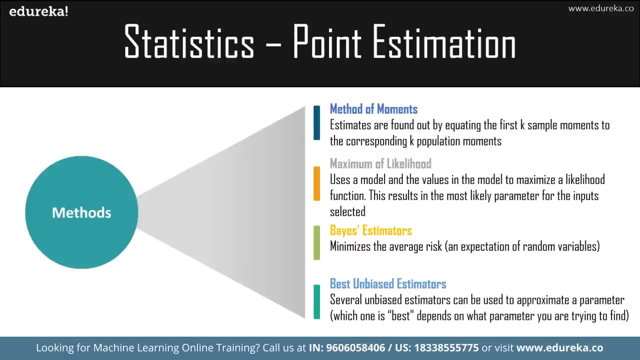 be so good enough that it is going to estimate the whole mean of the population. So this is how you use point estimation and try to approximate it for the whole, you know, population. So what are the different methods? we have methods of moment, methods of likelihood, base estimator and, best and best, 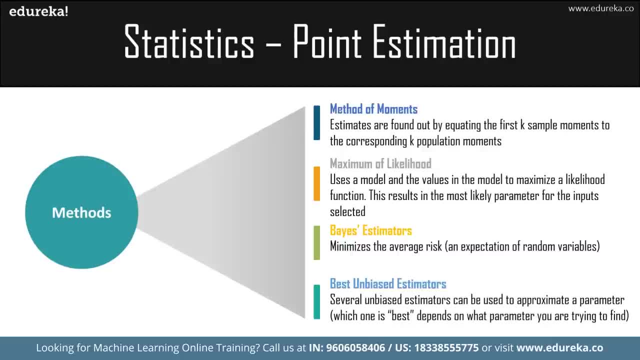 estimation. So estimates are found out by equating the first case sample moments to the corresponding K population moments, which is the method of moments, and then we have the maximum of likelihood, which uses a model to maximize a likelihood function. base estimator minimizes the average risk and it is an expectation. 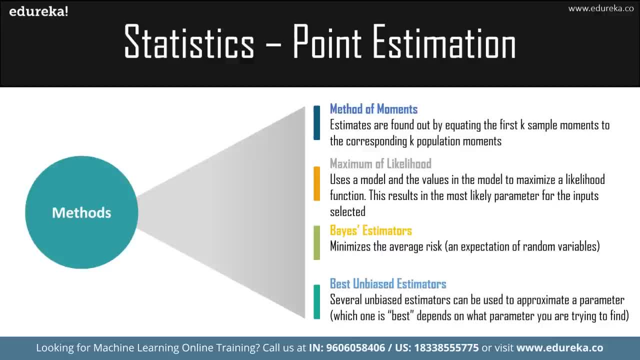 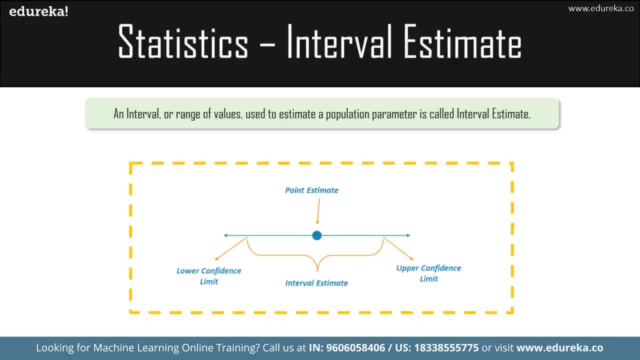 of all the random variables, and then we have the best unbiased estimators, which is used to find out the best depending parameter. So that is all that we require. from point estimation. Let's move over to interval estimates. So an interval or a range of values is used to estimate the 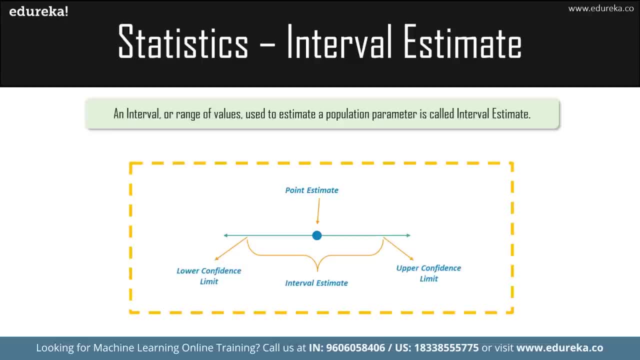 population parameters. So we have a point estimate and we have an interval which gives us the low confidence and the high confidence limit. How is this going to happen? There are three things that you need to remember. there is something called as the confidence interval, and it is: 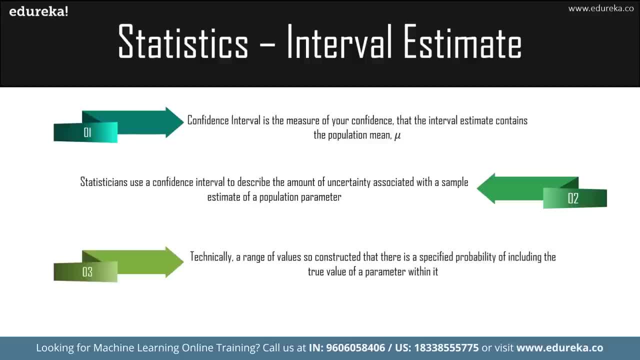 the measure of your confidence that the interval estimate contains the population mean you. so statisticians use a confidence interval to describe the amount of uncertainty associated with the sample. technically, a range of values are so constructed that it is specified probability of including the true value of a parameter within. 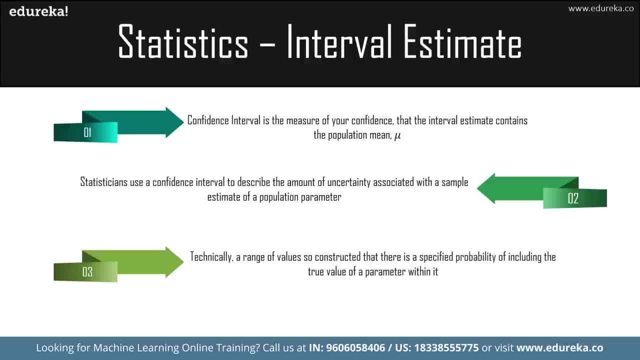 it. So, for example, let's take a sample where we have 10,000.. So let's say that we have something called as a supermarket. so out in that supermarket We have collected a lot of data and in that data I am seeing that this particular items. 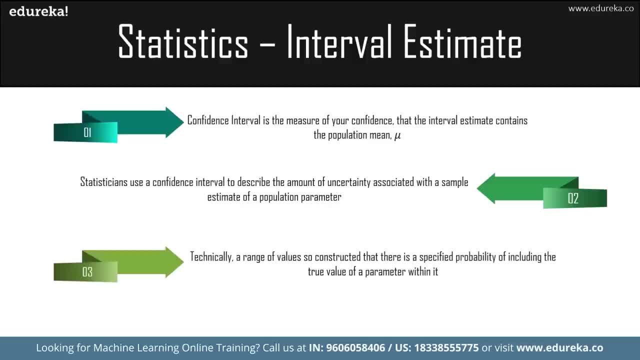 Okay. so item 1 and item 2- 2- if they both are kept together, they are going to be sold together, and I say that with 90% confidence, so that 90% confidence, Okay, is what is my confidence interval? It can be in between this range. 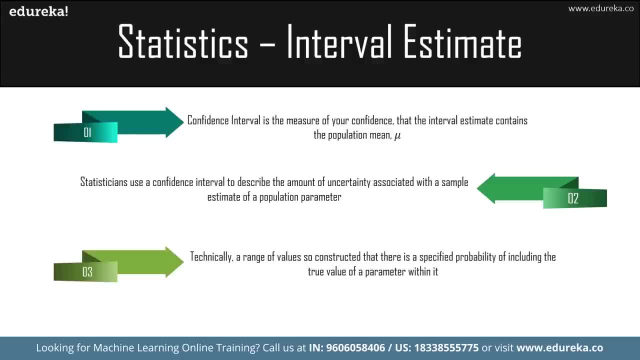 It can be between 90 to 95%, and between 90 to 95% it is highly likely that that particular thing is going to happen. So that is my confidence interval. So what is the sampling error? It is the difference between the point estimate. 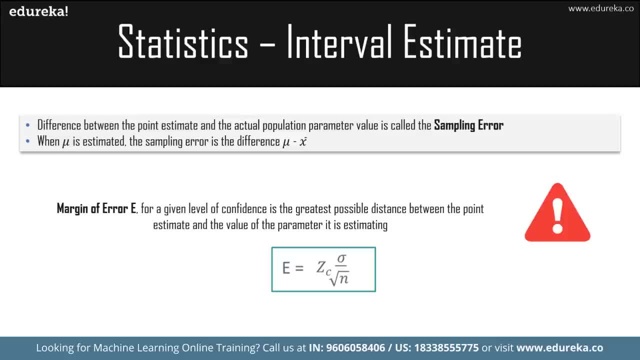 and the actual population parameter, which is the sampling error. Okay, so when you is estimated, the sampling error is mu minus X bar. it is mean minus the point. What is the margin of error? So for a given level of confidence, it is the greatest possible distance between the point estimate. 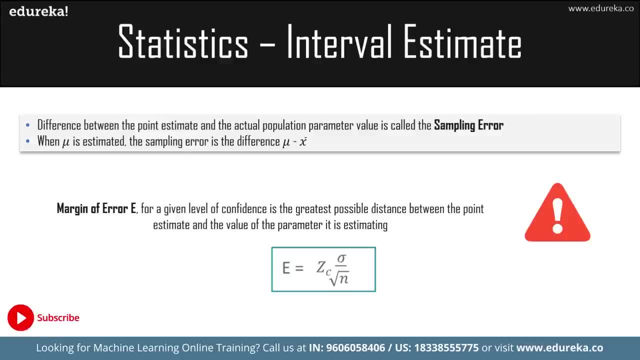 and the value of the parameter It is estimating. what this basically means is that it is the greatest possible distance between what you have predicted and what it actually is and what level of confidence you are giving to it again. So that is the margin of error, how much error you can allow. 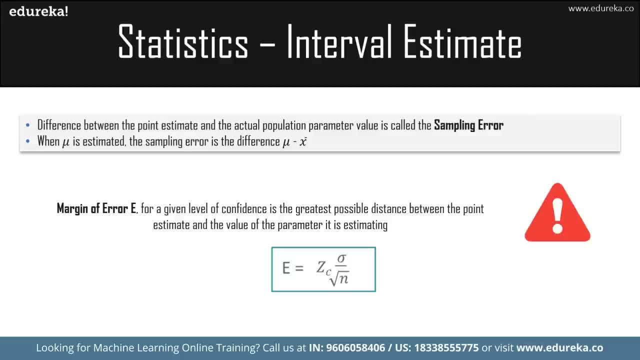 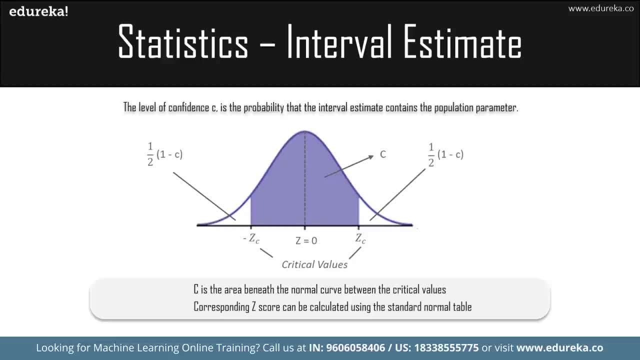 for the predicted model is: what is the margin of error? So I hope you have understood that. so the level of confidence is the probability that the interval estimate contains the population parameter. So, as you can see here, all the parameters that come under C right are what we are allowing. 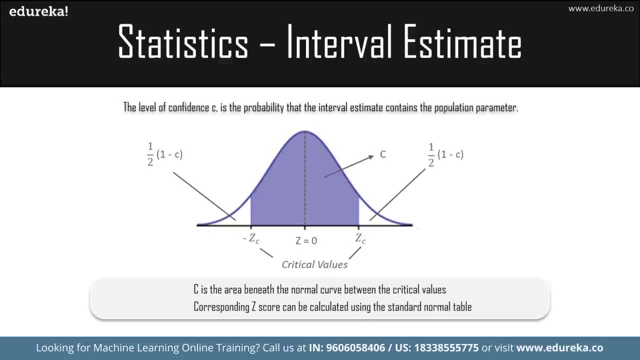 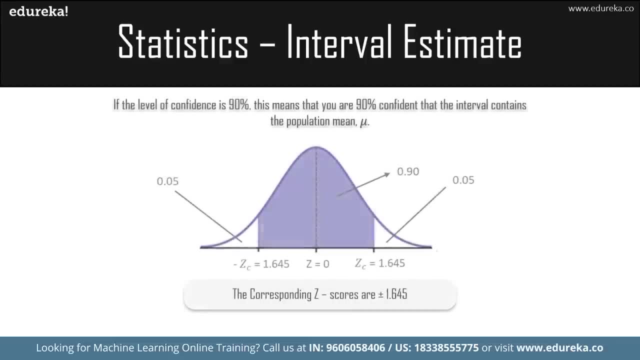 Okay, that is the margin of error that is allowed. But whatever comes in- minus Z C and plus Z C, we are not going to take that. those are the interval estimates. So finding these intervals is what is our probability. So finding these interval estimates is what is our work. 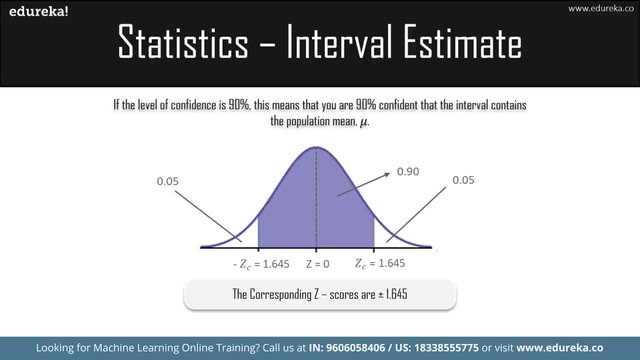 over here. Okay. So, for example, if the level of confidence is 90%, this means that you are 90% confident that the interval contains the population mean 0.05 and 0.05 of minus Z C and plus Z C. 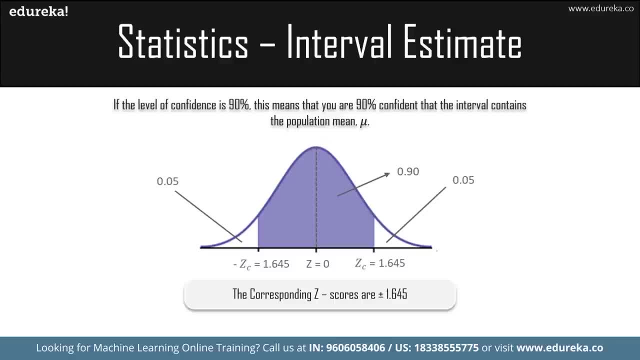 Is equal to plus 1.645 and minus 1.645.. Those are the Z scores. anything minus or plus of 1.645 is not allowed. So those are the values that we are concerned with when we are working with interval estimates. 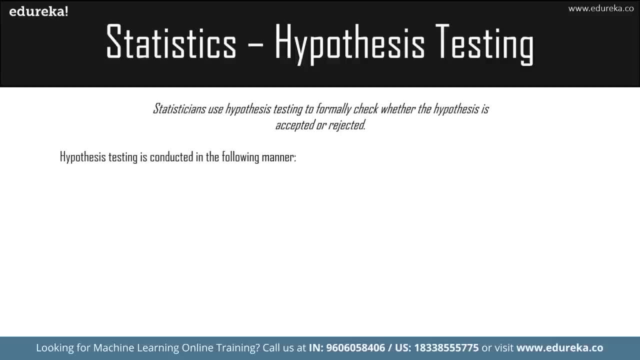 So now that we have understood everything we needed to from inferential statistics and descriptive statistics, let's move over to hypothesis testing. So what is a hypothesis? first of all, it is some event that you have made up which may have the probability of happening. 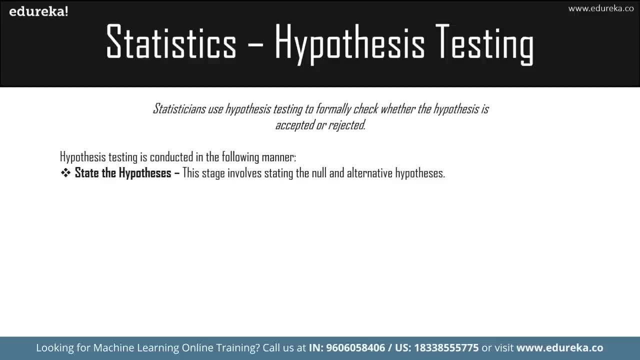 or not happening. testing that hypothesis is what is hypothesis testing is, you know, formally checking whether this hypothesis is accepted or rejected. So how is the hypothesis testing conducted? you first state the hypothesis and then you formulate an analysis plan of how you are going to, you know, test this particular hypothesis. 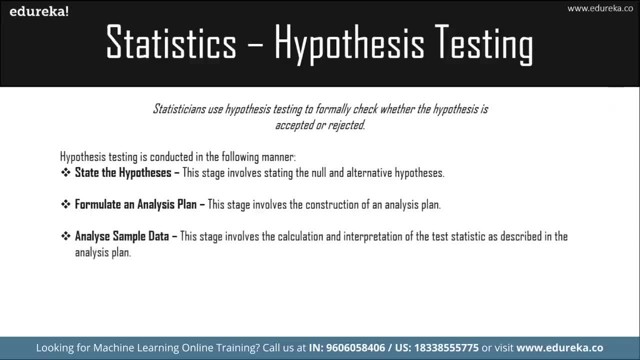 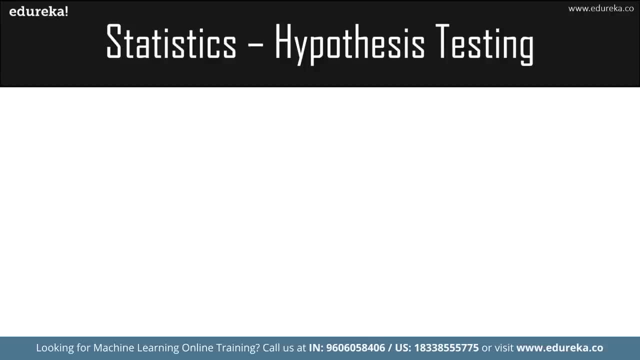 and you get all the output. you analyze the data that you've got from all of it. So then you understand whether this particular hypothesis has failed or it is a good hypothesis. Okay, suppose I have four boys over here, which are Nick, John, Bob and Harry. 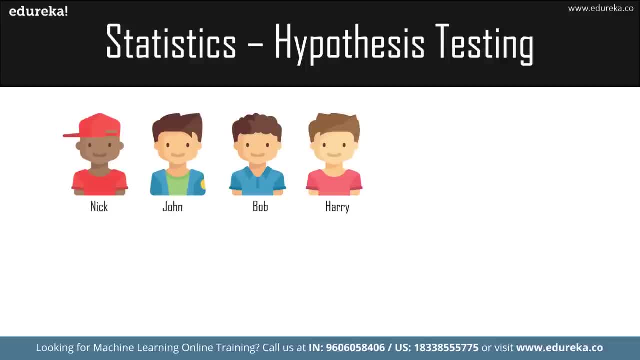 So they were caught doing mischief in the class and they have to now serve detention for almost two months. Okay, the detention is is basically they have to clean the classrooms. So John, over here, comes up with an idea, saying that I'm going to write all the names of ours into chits. 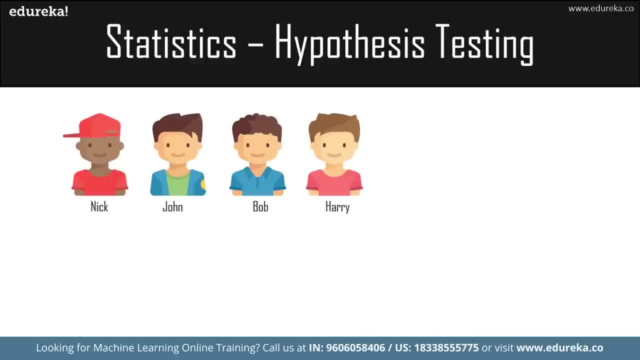 And then put them into a bowl. Who's ever name comes out has to clean the classroom. So what happens here? that we are going to assume that the event is free of bias. So our hypothesis is: what is the probability of John not cheating? 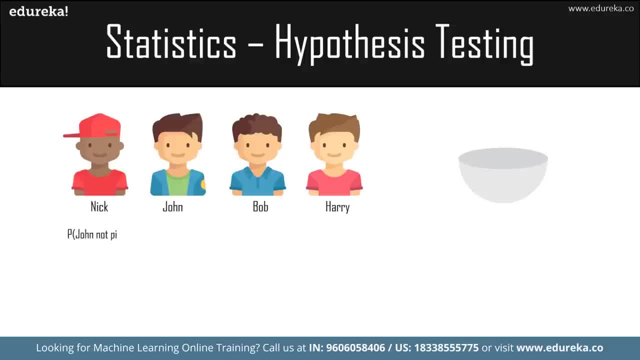 Let's find out what happens actually. the probability of John not being picked up for a day is 3 by 4.. Now the probability just keeps increasing on and on if he is not picked up for three days. Okay, so it is 3 by 4 into 3 by 4 into 3 by. 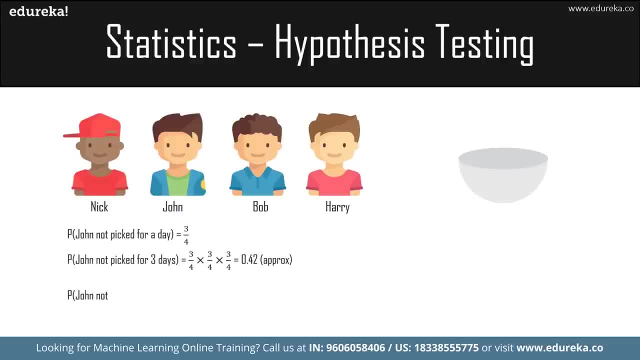 Is equal to 0.42 approximately. and what is the probability of John not being picked up for 12 days? It is 3 by 4 into 12 is equal to 0.03 to do, which is equal to 3.2 percent, which is less than 0.05, which is 5%. So what this? 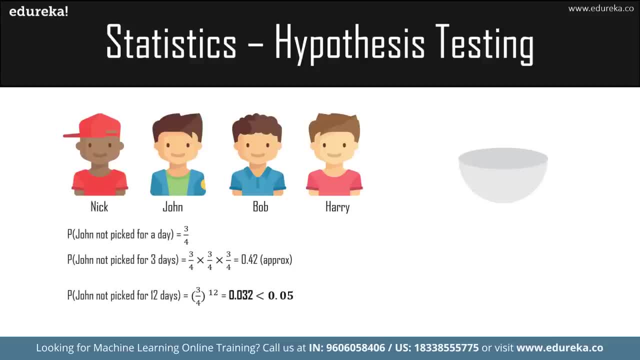 means is that our hypothesis was that John is not cheating, but actually John is cheating over here because it has come down and it is come below the threshold value of 5%, which is 3.2.. So now all of us have come to know that John is cheating. 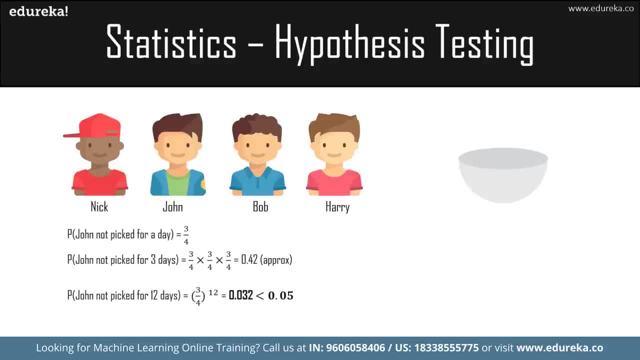 because he has not even written his name in the chits. So this is how the hypothesis works. So what is the null hypothesis? is the hypothesis that we have created in the beginning. Okay, that John was not cheating. that was a null hypothesis. It has no result which is different from the assumption and 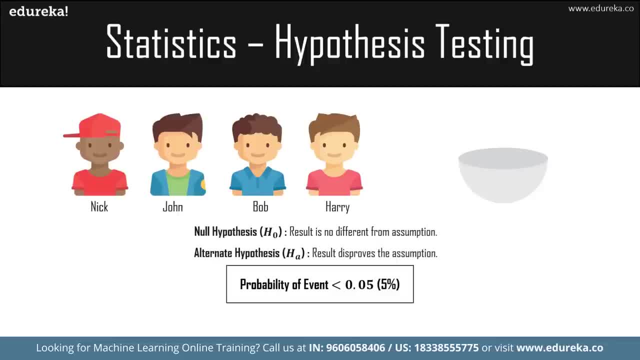 we have an alternate hypothesis, which means that our results disapprove the assumption. We had a hypothesis that John is not cheating, but actually through our results We found out that John is cheating. So this is what is the hypothesis testing thing, and we have a 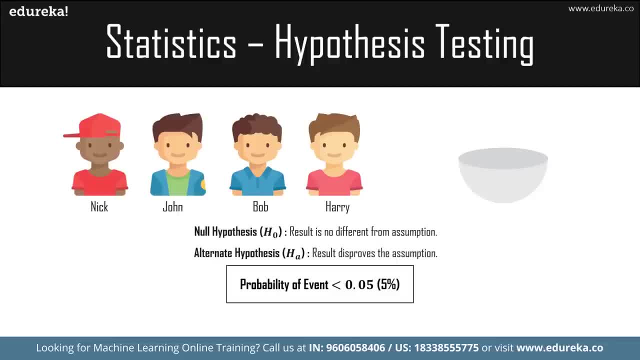 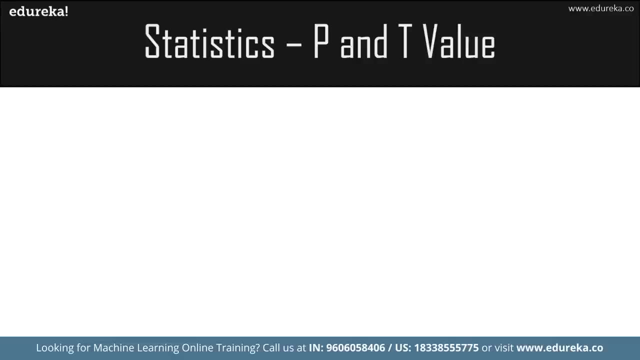 threshold value. If the probability that we are testing goes below this threshold value, it means that the particular hypothesis has failed. So this is what is the hypothesis testing. So now we need to know something about the P and T values. Okay, what is the P and T values? the P value and the T value? 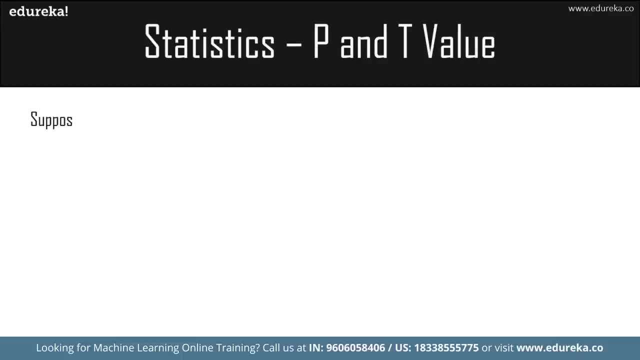 help us in our hypothesis testing. Okay, we want to find the height of students, Students who are greater than 5 feet and 7 inches. Okay, So we take a sample of hundred students and find that the mean height was 5 feet and 9 inches. 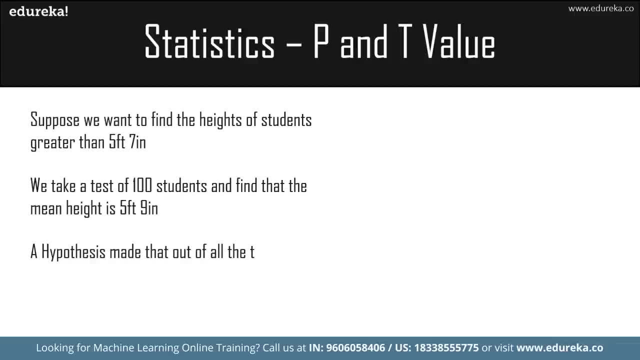 Okay, we make a hypothesis that out of all the hundred students, there is going to be at least six students who are greater than 5 feet and 9 inches. So this is our P value. It is the probability value that we are seeing that this 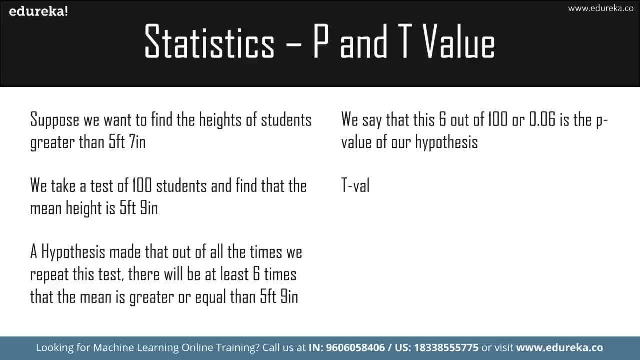 particular hypothesis is going to be correct. We say that at least out of hundred times six students will at least have a height which is greater than 5 feet and 9 inches. Okay, So this is the P value. This is the probability value that we have given to a hypothesis. 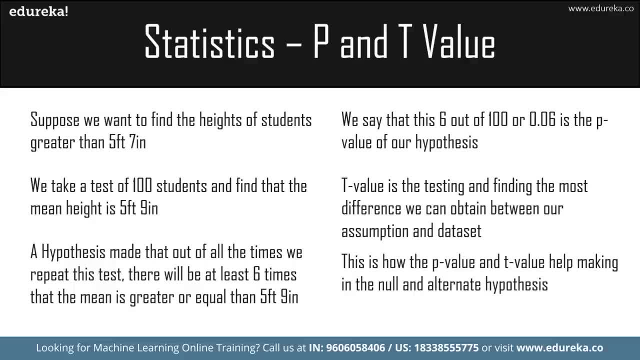 The T value is testing this particular hypothesis and finding the difference that we have found out from our assumption and what we have actually calculated from our results. So this is how the P value and the T value help in making the null and alternate hypothesis. You know, you find the result of the null hypothesis and the 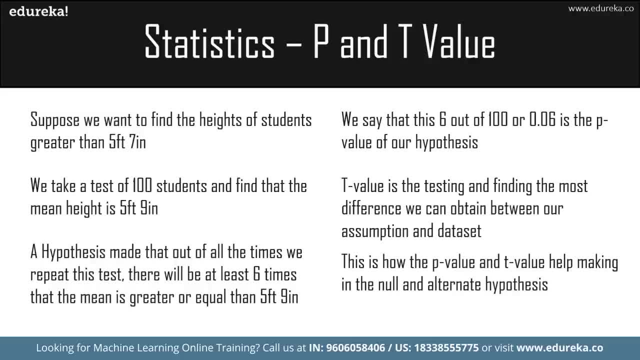 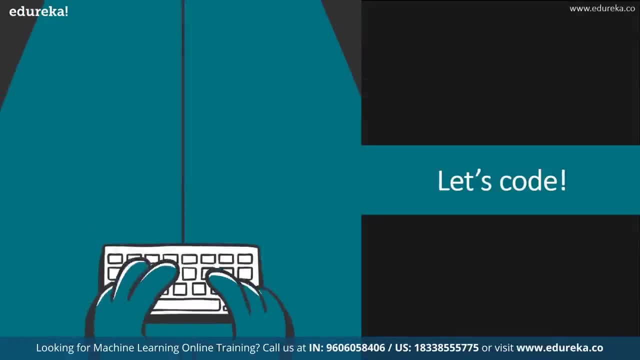 alternate hypothesis. So this is how the P and the T values help in making and observing the results from the null and alternate hypothesis. Okay, let me show you a code where we are going to find the mean median mode accordingly and how that becomes helpful to us. 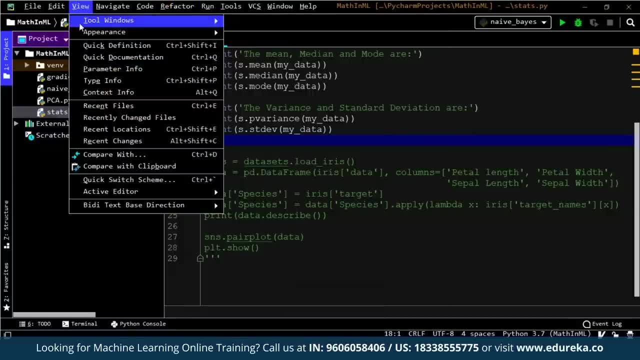 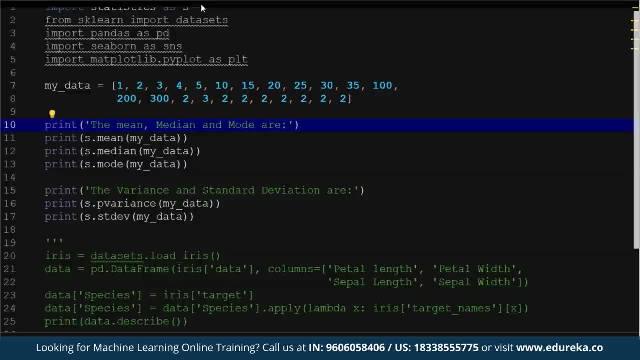 Okay, so let me go back to the presentation mode. I have my data over here, which is this particular data. So I am going to import statistics as s and I am going to just find the mean median mode of it. So let me just run this program for now. 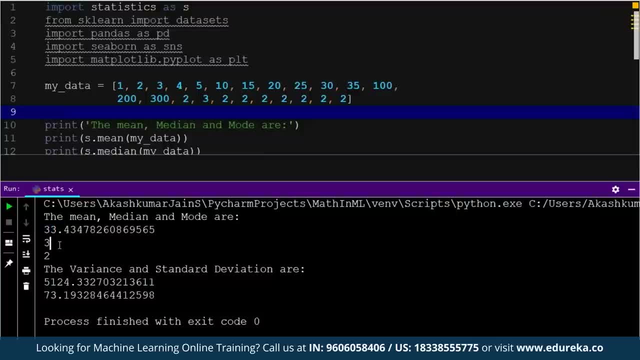 So, as you can see here, the mean is 33.43 and the median is 3, and the more is 2. 2 has been repeated the most number of times, So that is the reason it is the more, and the variance is a 5: 1: 2. 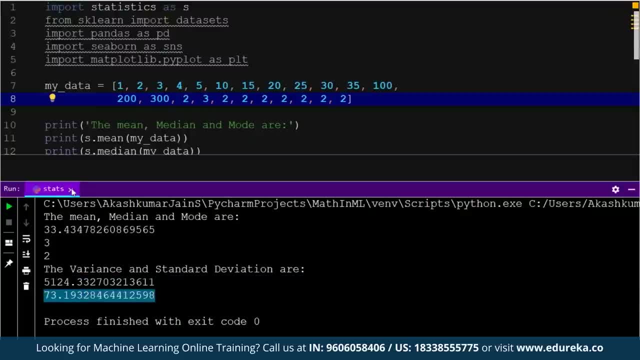 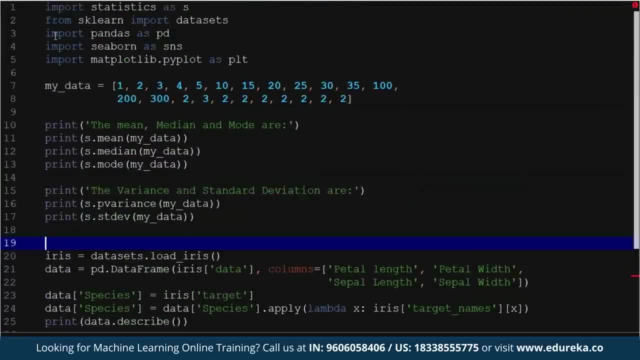 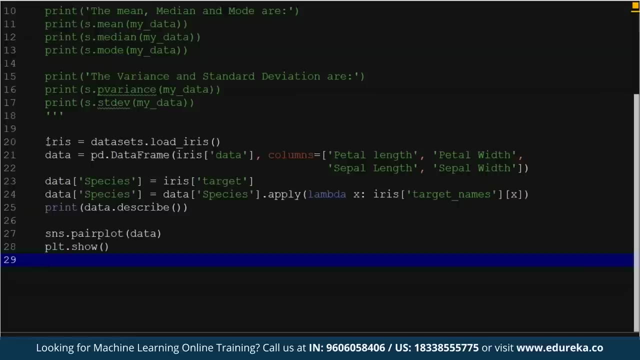 4 and the standard deviation is 73.. That is how the mean median mode is calculated. Let me run the program now so that you can understand what we are trying to do. So let me close this out. What's happening over here is: I have the iris data, which is the 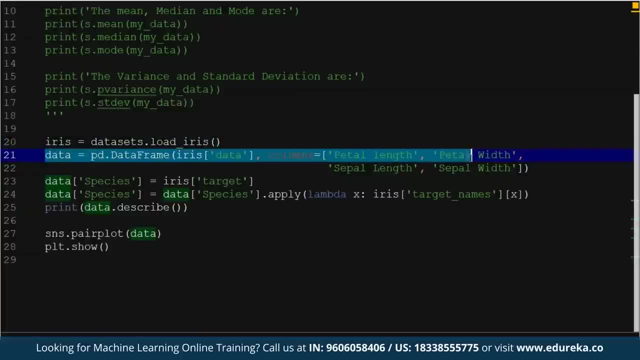 load iris and then I am creating it into a data frame. Okay, simple enough. after that I am seeing that those species is the target and the data species is equal to. I am going to just apply all the Lambda parts of it, Okay, and then I am going to 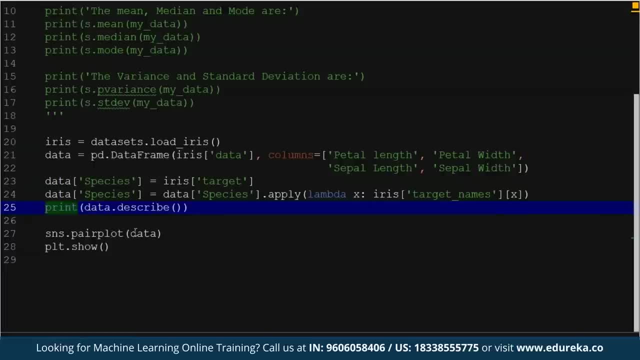 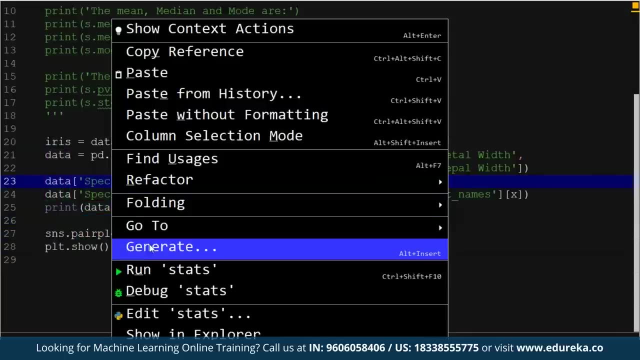 Get the description of the data and after that what I'm going to do is I'm going to take this data and I'm going to pair plot it and then I'm going to show the plot to you. So let me run the program. Let me show you the figure first. 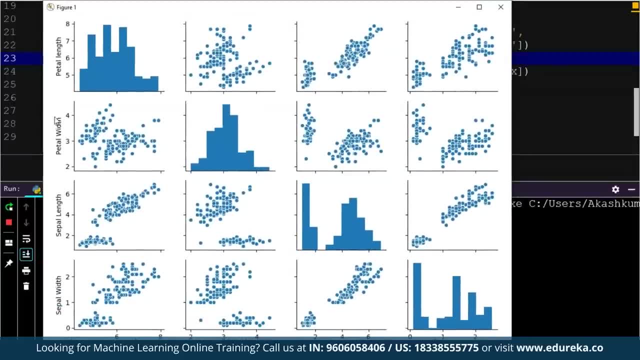 So I had four features over here, right? So that was the petal and petal with a sepal and then sepal with. so if you can take a look at this data, you can see that there is a normal distribution here. There's a normal distribution here. 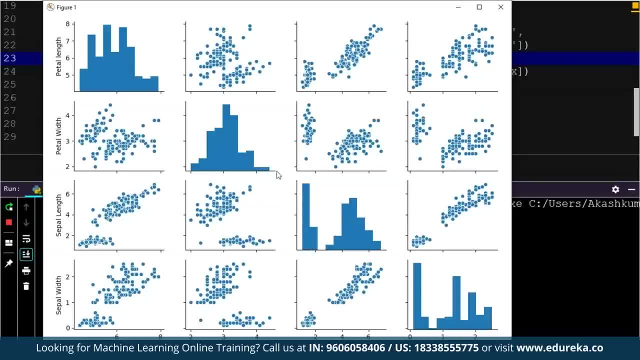 Also, there's a normal distribution over here, with some exclusions over here, and there is a normal distribution here too, but with some exclusions here. So, looking at this, I will be able to understand. if I want to, you know, apply the Gaussian name based classifier or accordingly. 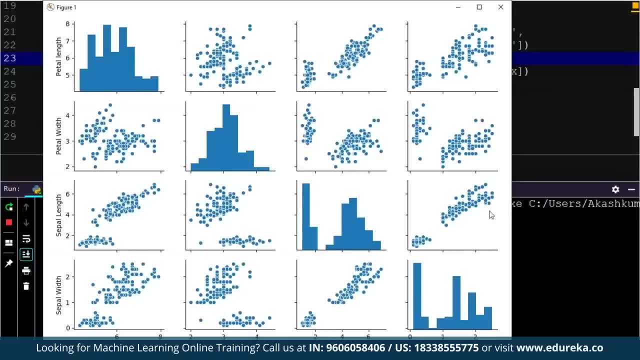 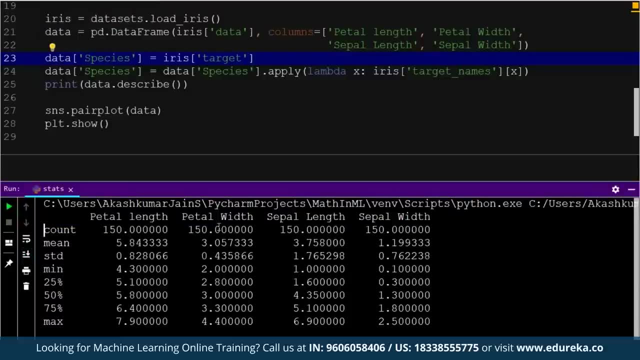 to, however I wanted to, so this is how statistics has helped me to understand. What is my data looking like? now? Let me go back over here. So, as you can see, This is the count of a 150 right. simple enough, Then? what is the mean? 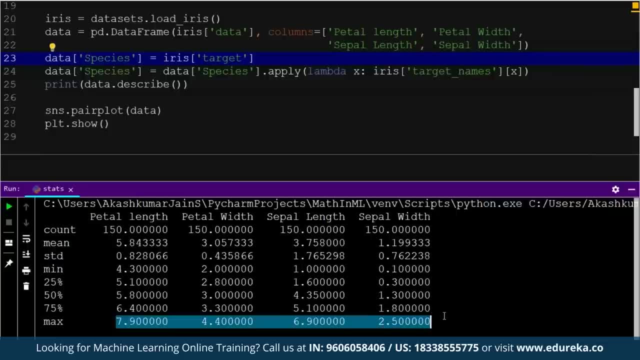 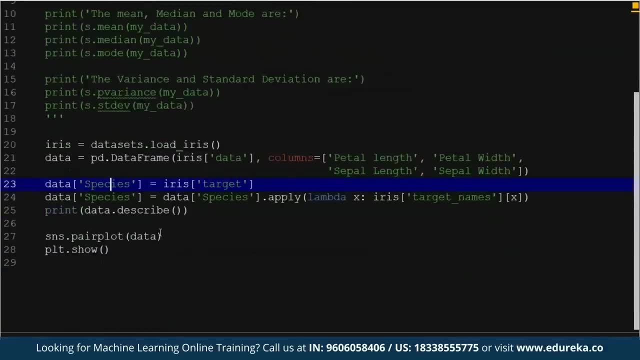 What is the standard deviation? What is the maximum length and maximum width that you can find over here? All of this is done using the describe part of it. Okay, and describe is a function that is already available in pandas, So that was a very simple example of how I was able to understand. 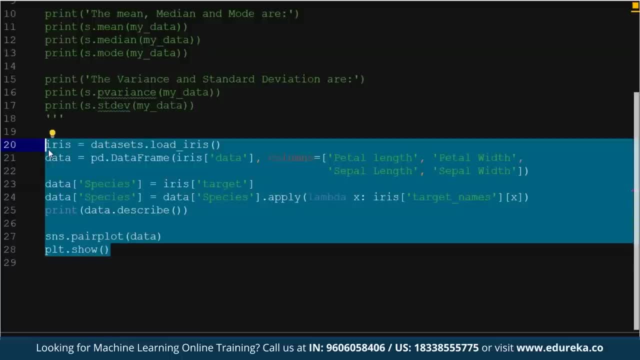 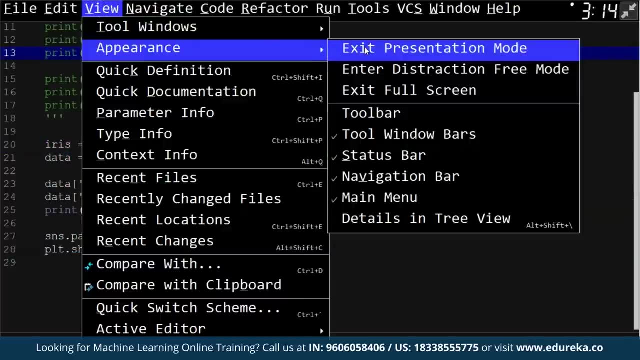 how I have to use the Gaussian name based classifier for my iris data, which I showed in the probability part. right now, We are done with this. Let's go back to the presentation. So with that program, that brings us to the end of statistics.